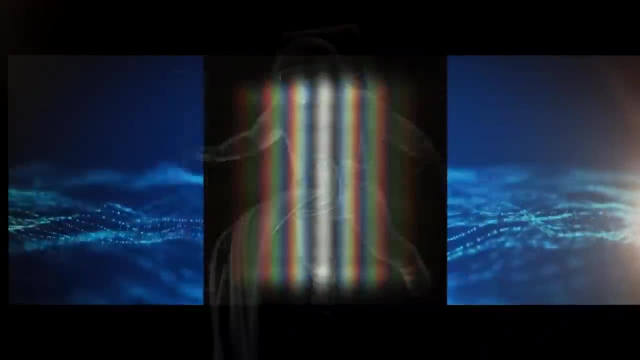 But of course it will be eerie to realize that light is not just a thing, But of course it will be eerie to realize the eternal cold. So as long as we can see, we'll see. No optical sensor can detect total darkness Or take black holes. 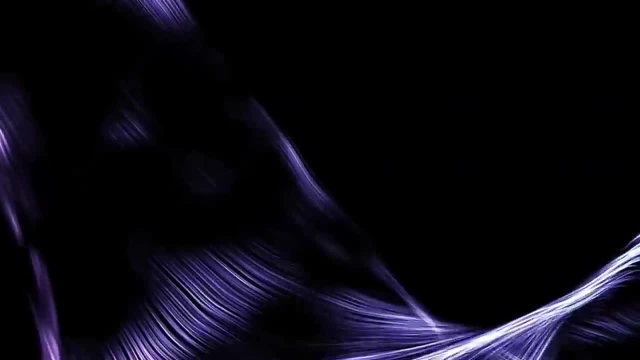 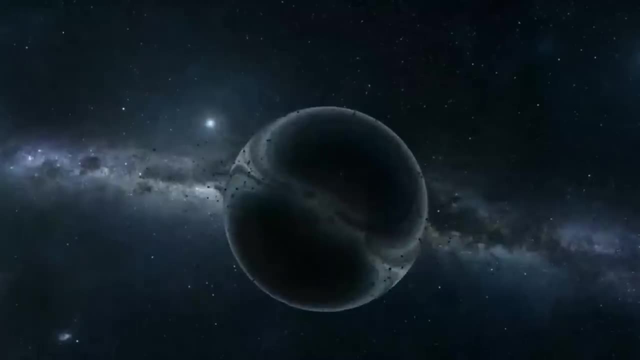 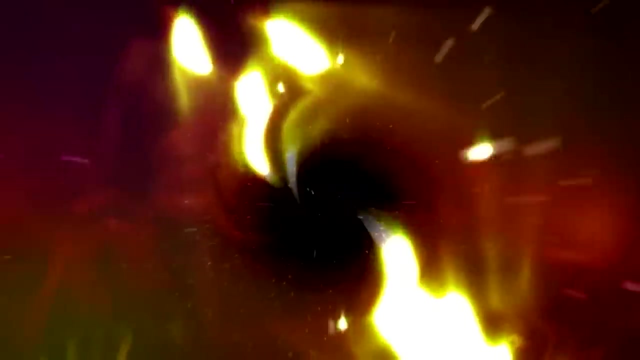 The darkest of the supposed objects. Even they are capable of emitting some percentage of light, according to some theories. In physics, unlike in the realm of interpersonal relationships, light always defeats darkness. Electromagnetic waves are a collection of all sorts of things. 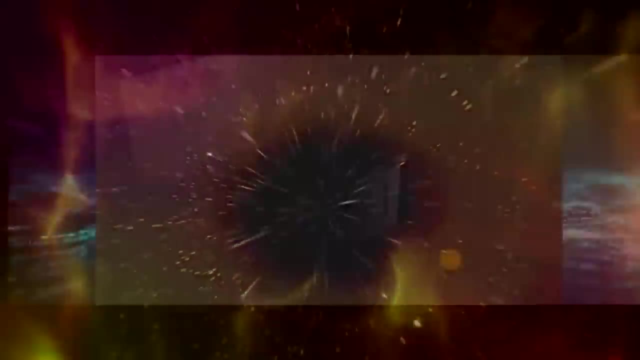 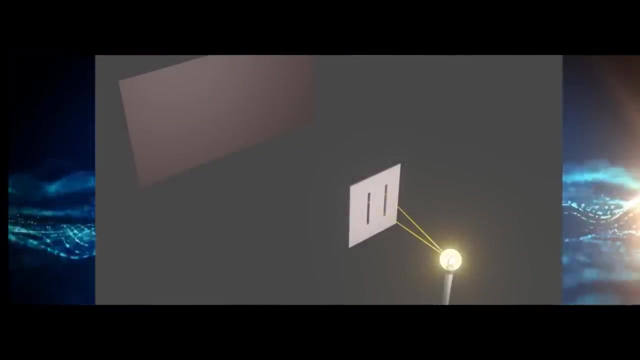 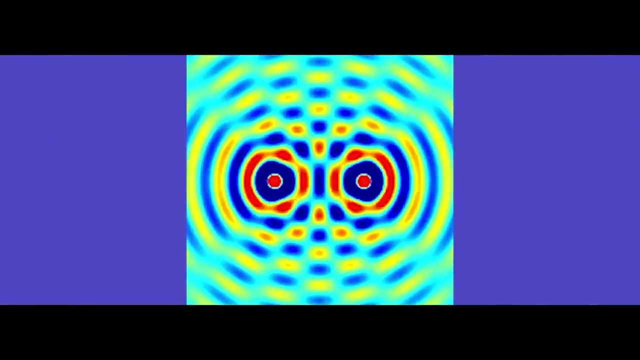 Alternating electric and magnetic fields that propagate through space at a specific frequency and wavelength. The spectrum of electromagnetic radiation includes, in addition to visible light, radio waves, microwaves, infrared, ultraviolet, x-rays and gamma rays. Yes, light plays an important role in physics. 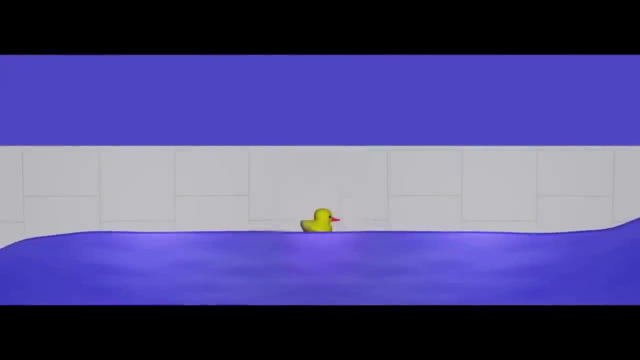 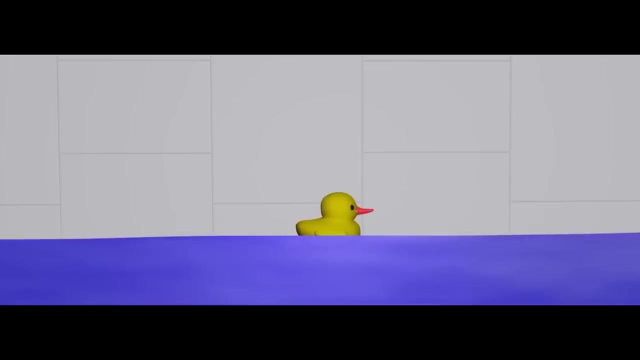 because of its ability to interact with matter and change its properties. When light particles, photons, are absorbed, atoms and molecules move to higher energy levels, which can cause chemical reactions, thermal radiation, changes in the state of matter and even nuclear reactions. 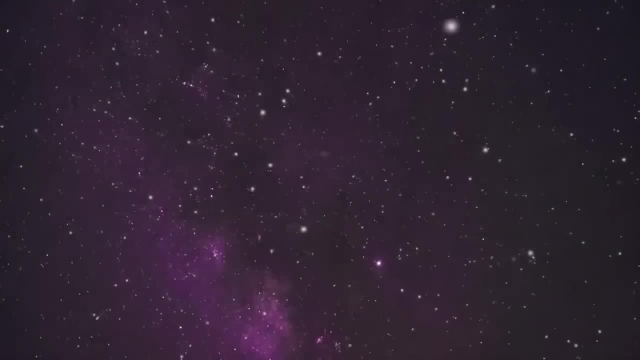 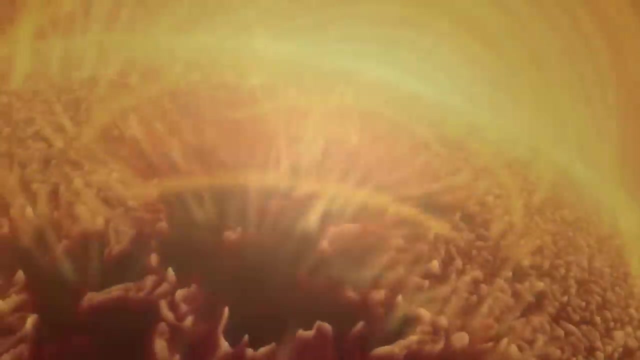 Where does light itself come from? Let's take the example of the emission of light by the sun. In our star, numerous chemical and thermonuclear reactions take place which are accompanied by the emission of quanta of light When two hydrogen atoms collide. 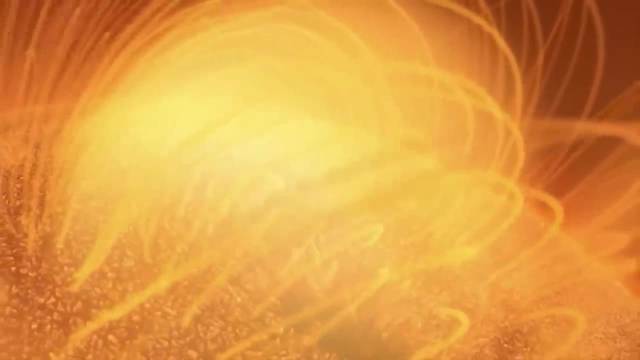 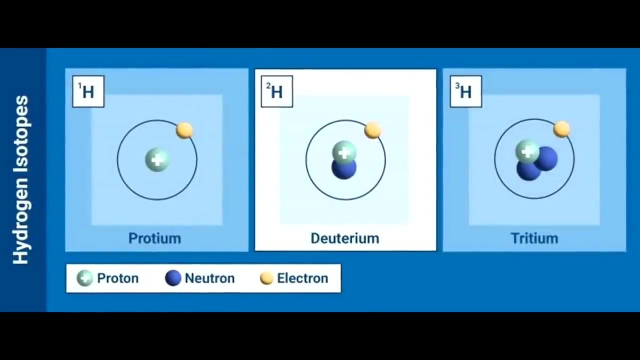 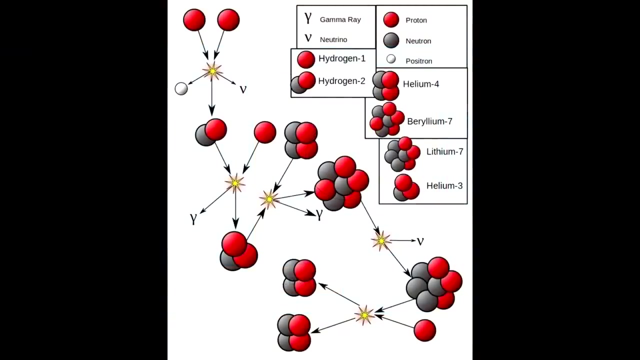 they combine to form one atom called deuterium, Which is lighter than the atoms from which it was formed, And the extra energy is released as a photon Deuterium in turn joins one more hydrogen atom and helium Three is formed. and one more photon is released. When two helium three atoms collide helium, three atoms collide, helium, four, two hydrogen atoms and one more photon are formed. So the sun from four hydrogen atoms produces one helium atom and three photons, and that's just from one chain of reactions. 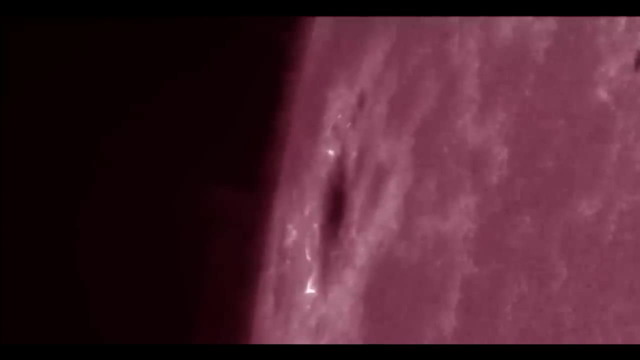 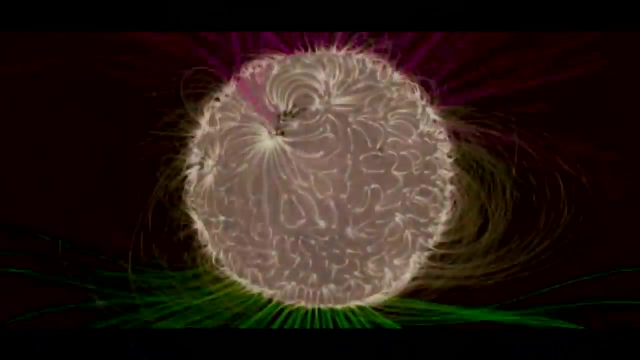 Each of these photons carries a large amount of energy and, for tens of thousands and millions of years, wanders inside the sun, colliding with atoms, heating up the sun and turning into dozens of photons with less energy and frequency visible to the eye. 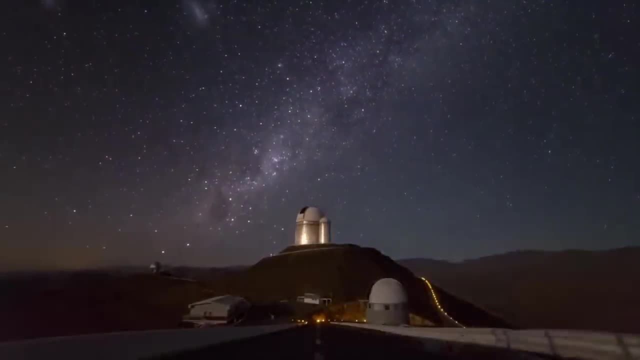 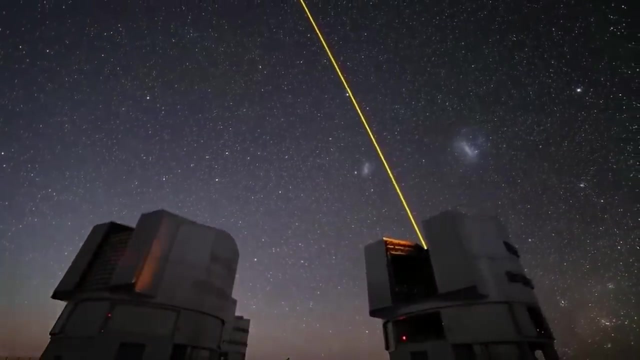 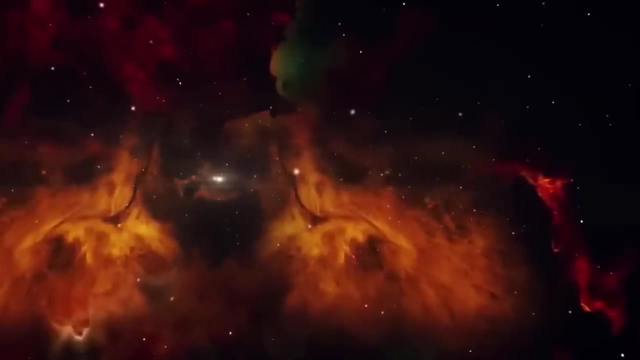 Sooner or later, these photons fly out of the sun and go on a long and sad journey through space, and some of them come to Earth giving us light and warmth. So what are the physical characteristics of light? First, it is speed. 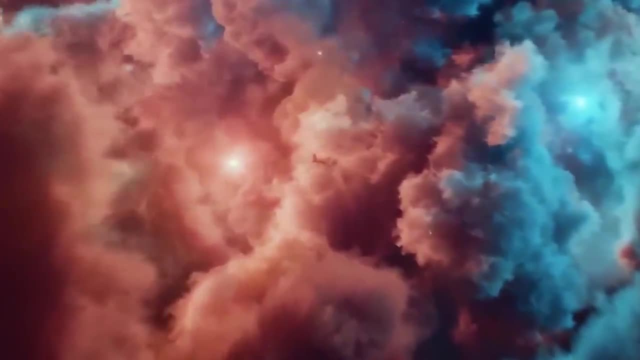 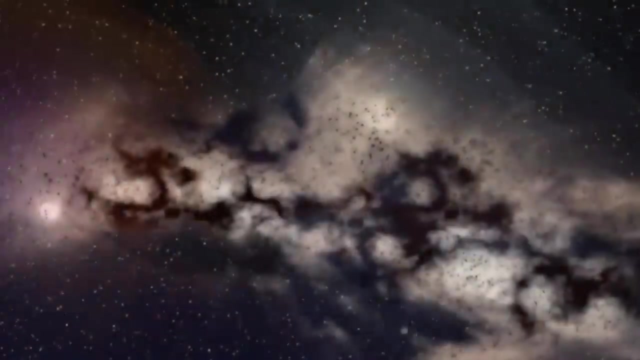 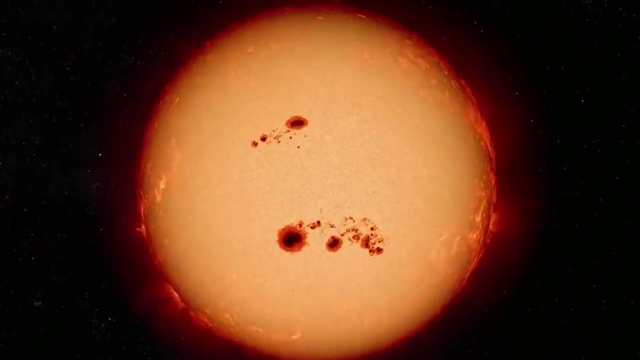 one of the most important fundamental concepts and constants in physics. In a vacuum, it is equal to almost 300,000 kilometers per second. What about the speed of darkness? How fast will the eerie darkness descend upon us? The simplest answer is that the speed of darkness. 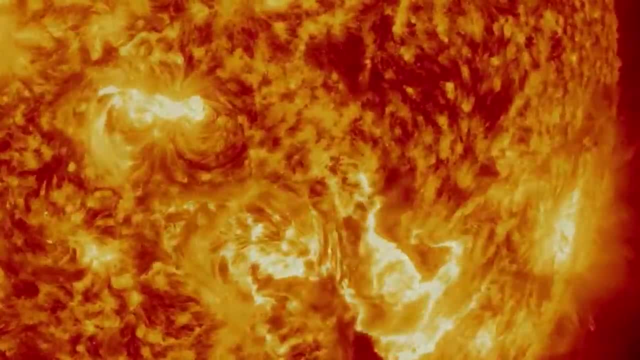 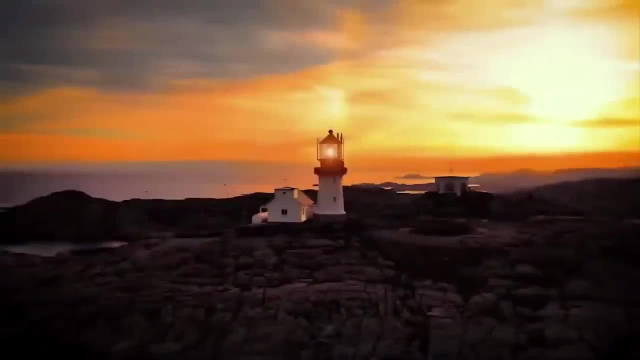 is the same as the speed of light. Turn off the sun and our sky will be dark eight minutes from now. What we used to call the speed of light is the speed of propagation, and it is not always the deciding factor. The shadow that falls across the landscape is cast by objects. 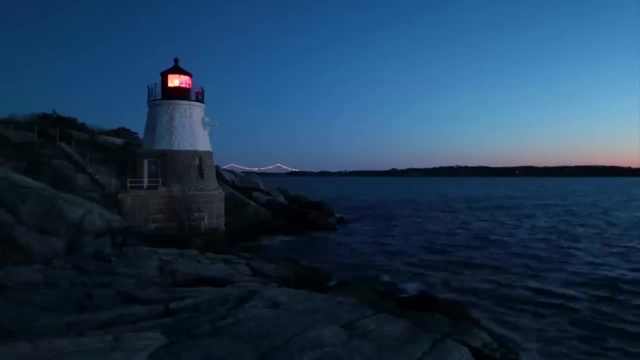 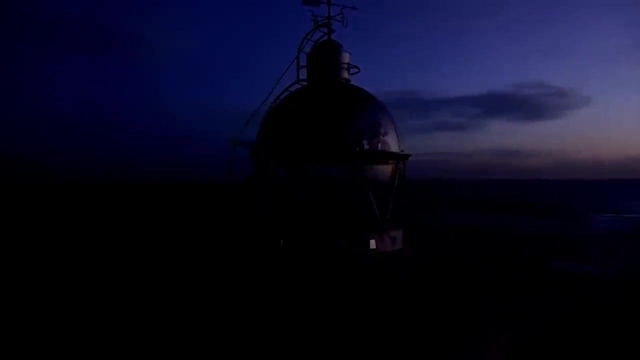 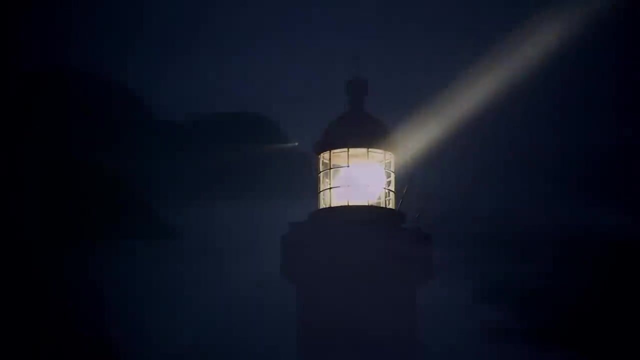 And the feature of those objects and the distance from them will determine how fast it falls. For example, a rotating lighthouse searchlight illuminates the surroundings at regular intervals. However, the relative rate of dimming of the surroundings increases with increasing distance from the lighthouse itself. 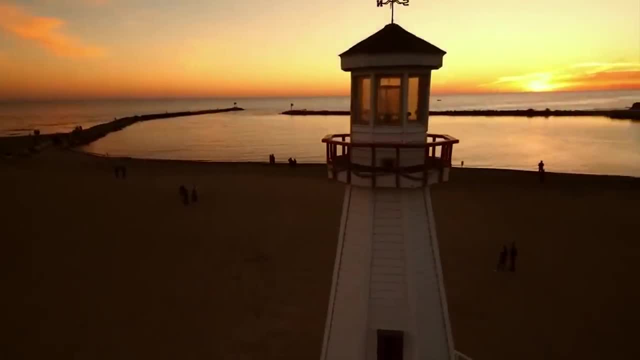 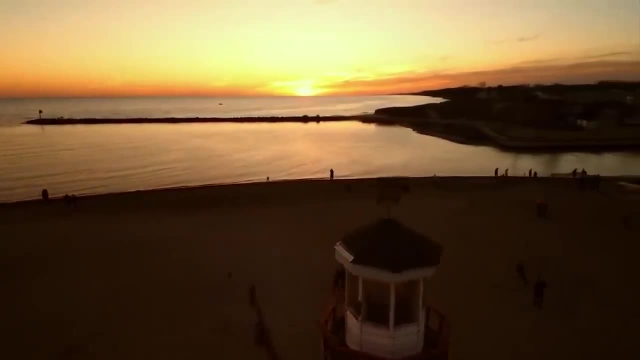 If you move far enough away from the lighthouse, lighthouse, the shadow will catch up with you faster than the speed of light propagation. Isn't that right? The same thing happens with neutron stars in space, For example. in other words, in this case, the speed of light will only mean a. 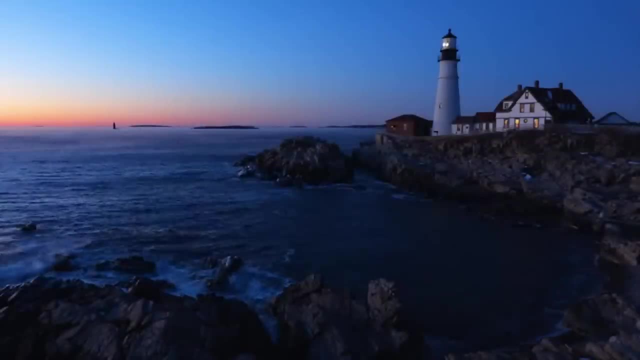 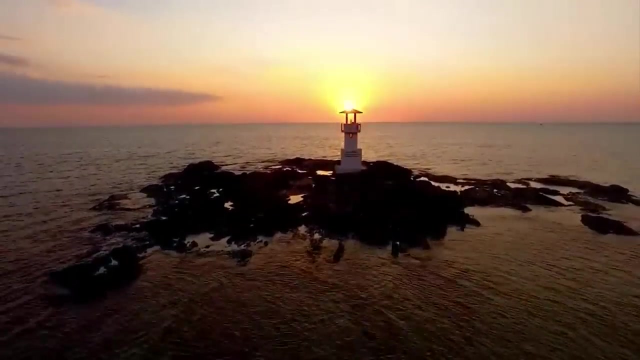 delay. Even if the beacon is pointed directly at you, you will see the light, Not immediately, but with some delay. However, this will have no effect on the course of events that you will see when you are in your position. In any case, you. 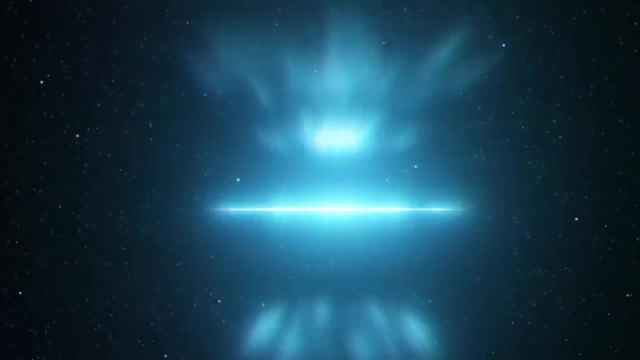 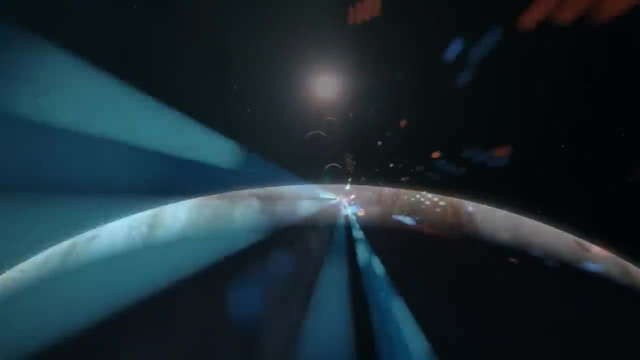 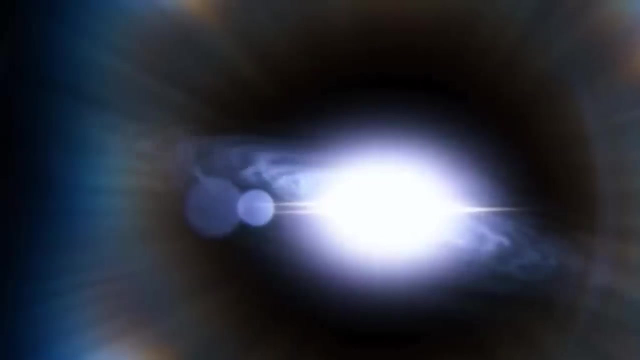 have been detected and have nowhere to run to. Moreover, light has an inherent wavelength. The spectrum of visible light is just the part of the electromagnetic spectrum that the human eye can see. The cone-shaped cells in our eyes act as receivers tuned to wavelengths in this. 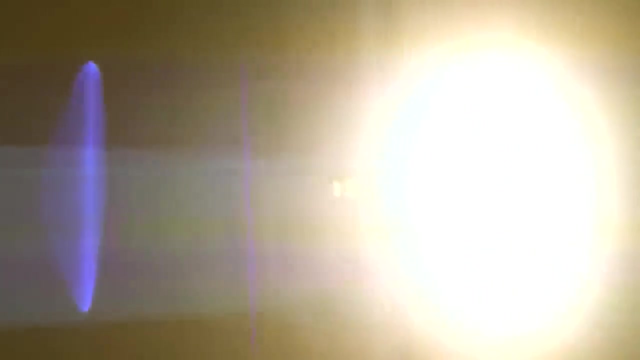 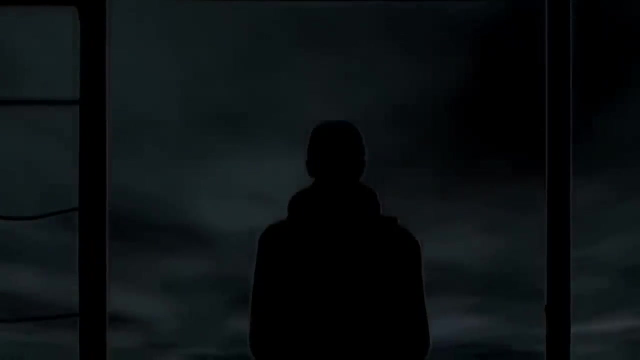 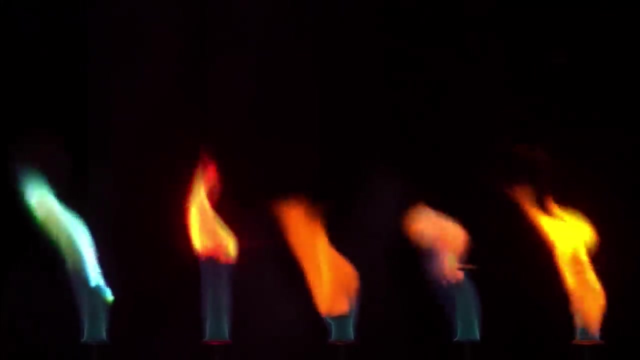 narrow band of the spectrum. Other parts of the spectrum have wavelengths that are true to mass, too large or too small and energetic for us to see. When objects get hotter, they emit energy dominated by shorter wavelengths, changing color before our eyes. 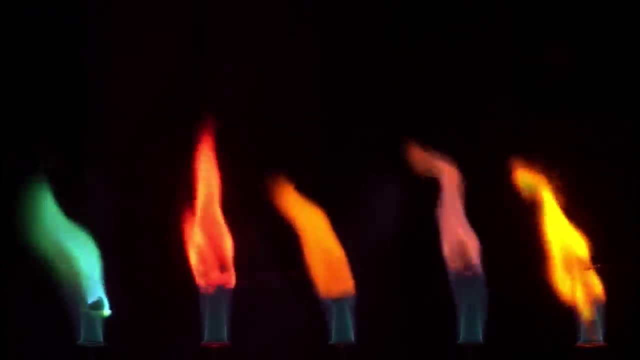 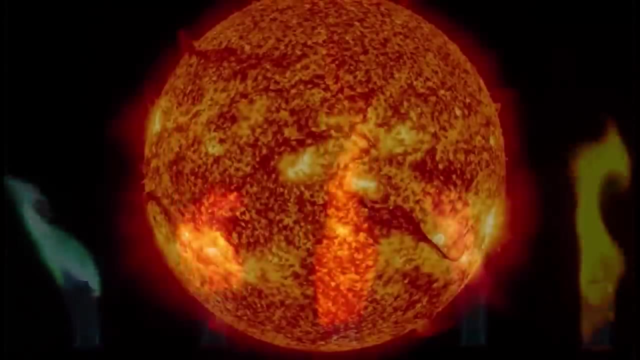 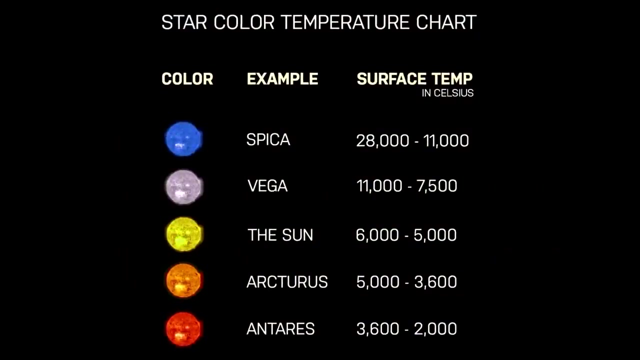 The flame of a blowtorch changes color from reddish to bluish as it is set to burn hotter. In the same way, the color of stars tells us their temperature. Our sun emits more yellow light than any other because its surface temperature is 5,500 dik. 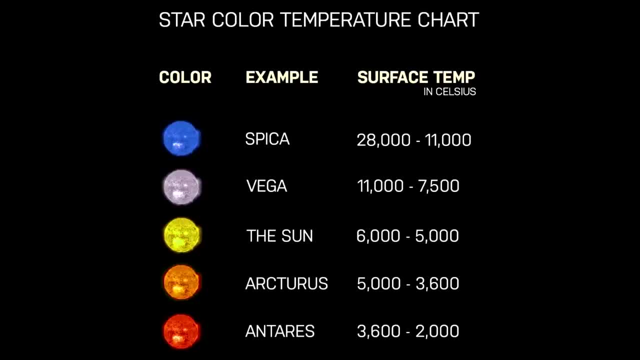 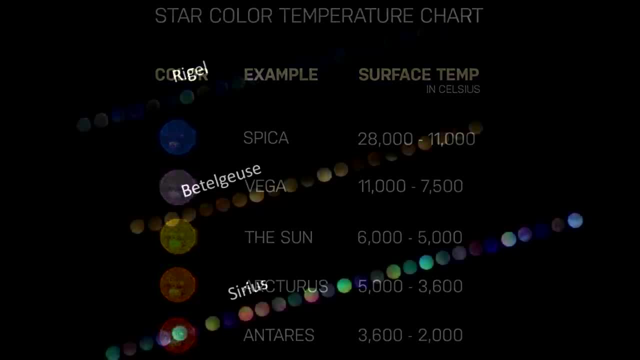 If the sun's surface were colder, say 3,000 diks, it would look reddish like the star Betelgeuse. If the sun were hotter around 12,000 dik, it would look blue like the star Rigel. 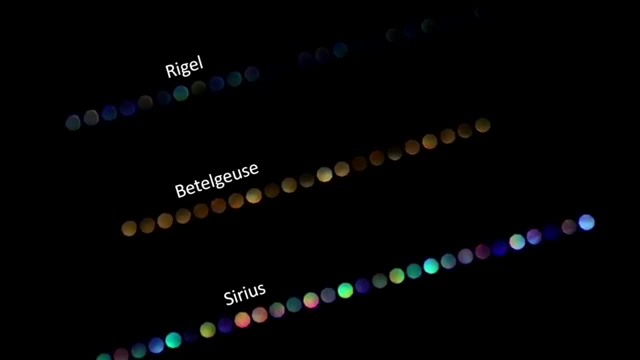 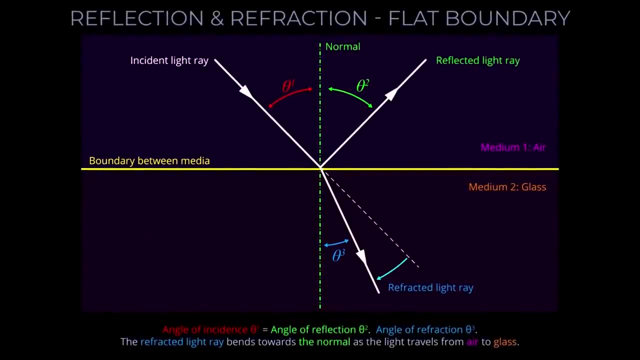 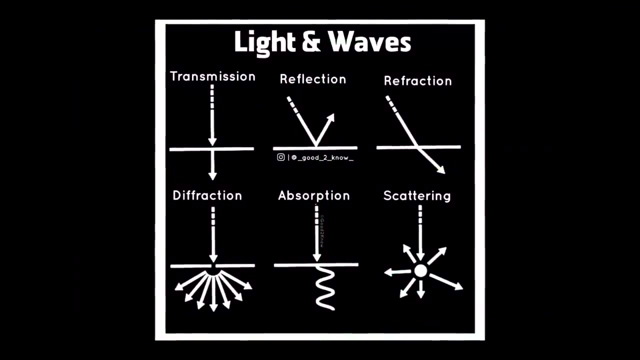 Reflection, refraction and absorption of light are the basic processes that occur when light interacts with matter. Let's break Each of them down a bit. Reflection is the process by which light reflected from objects hits the smooth surface of a mirror and is then reflected back. 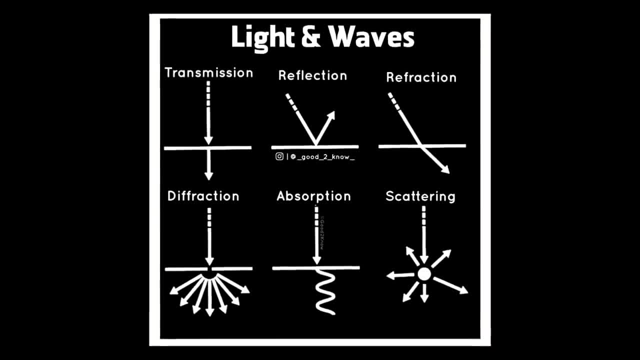 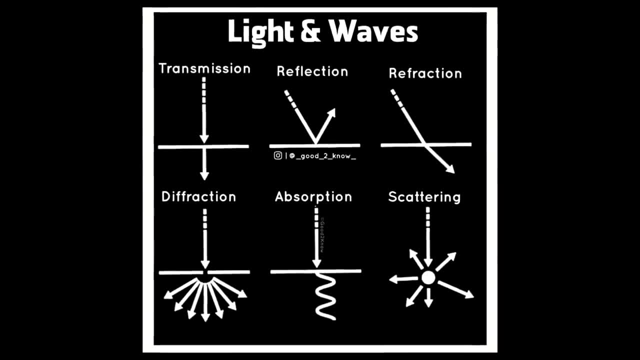 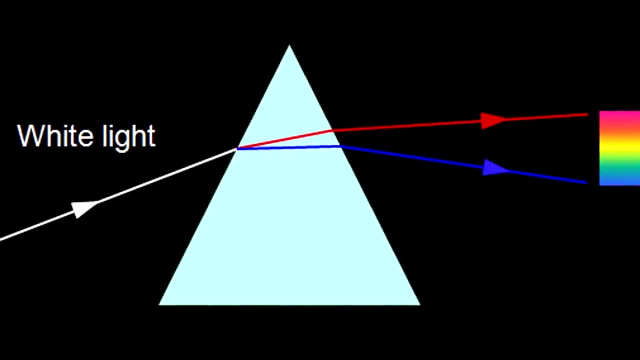 giving us an image of the object. That is, the angle of incidence of light is equal to the angle of reflection. Further, refraction of light is a phenomenon in which light rays change their direction of travel when passing from one medium to another with different densities. 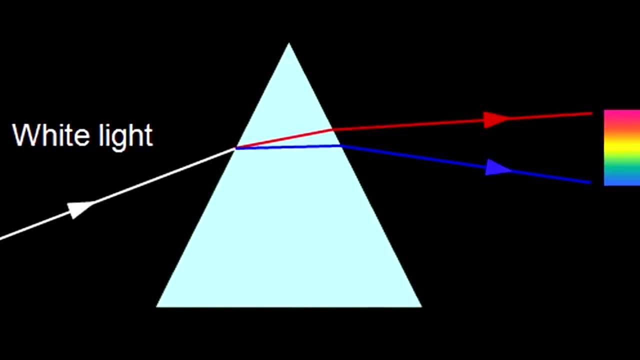 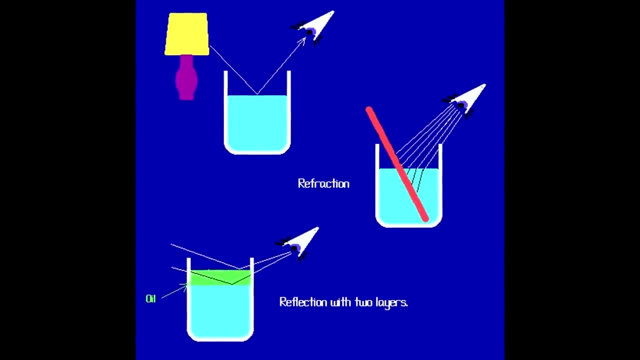 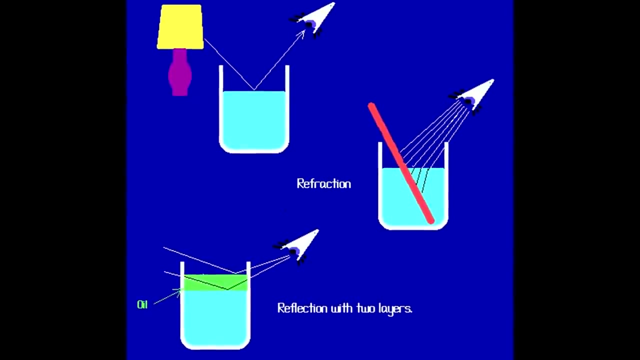 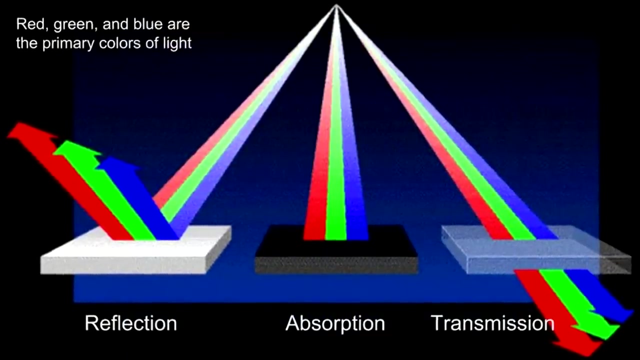 This causes objects in water to appear displaced or distorted compared to their position in the air. This is why faces in water are so creepy. Finally, absorption is the process by which light hitting the surface of an object is converted into another form of energy, such as heat. 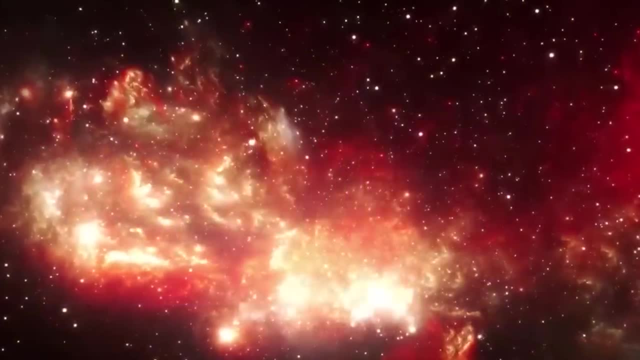 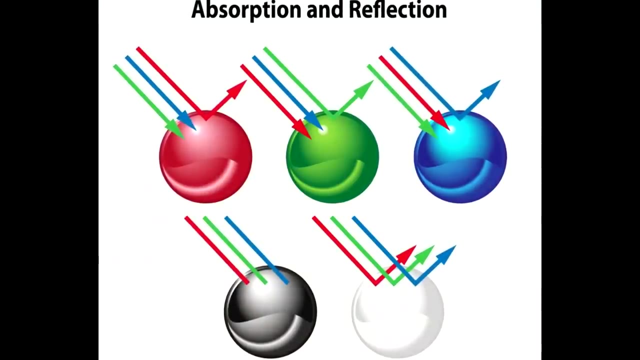 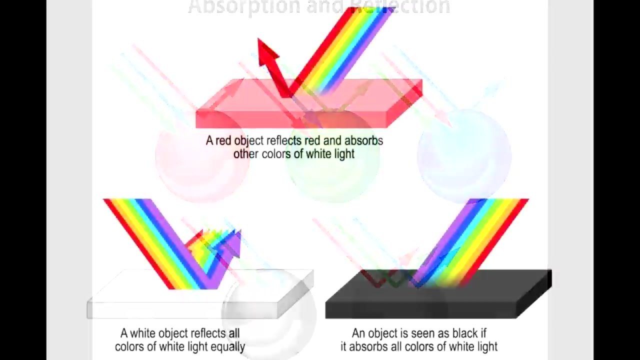 This occurs due to the interaction of light waves with material particles. For example, when an object is illuminated with blue light, the object may absorb all the blue waves and reflect red and green waves. As a result, the object will appear greenish. 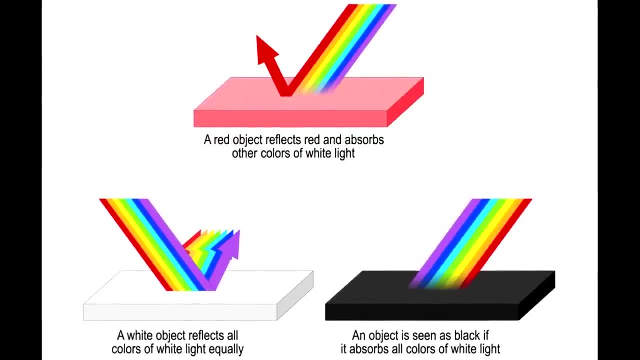 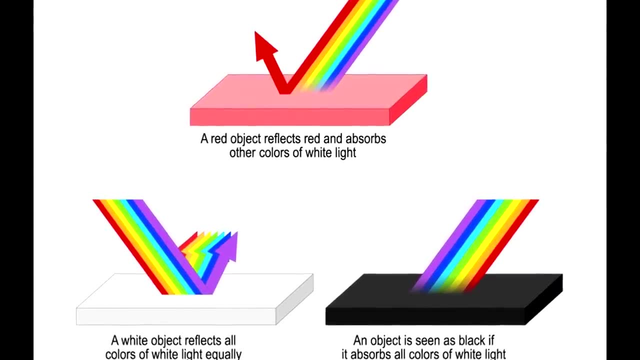 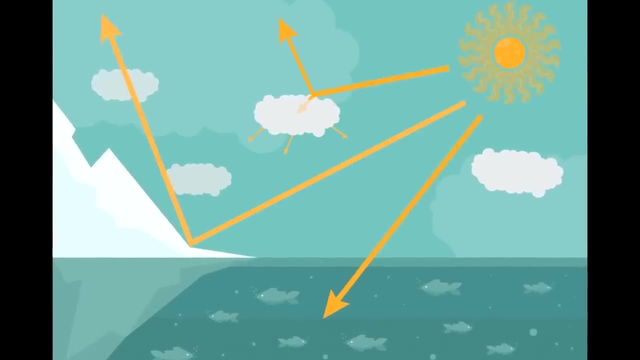 Red will appear greenish Red. This explains why objects have certain colors. They absorb some light waves and reflect others, and is not the work of sorcerers. So the interaction of these three processes determines how we perceive light and see objects. 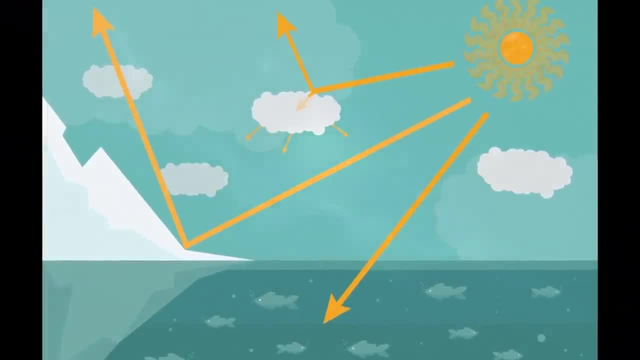 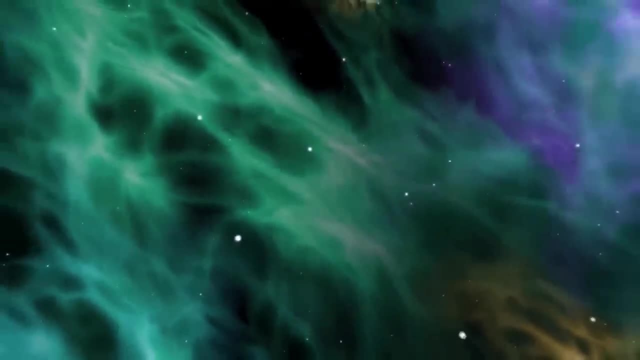 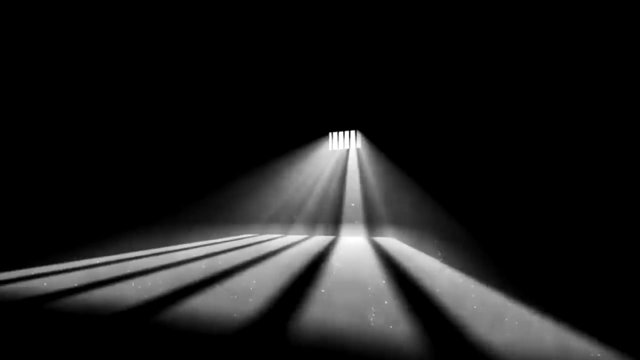 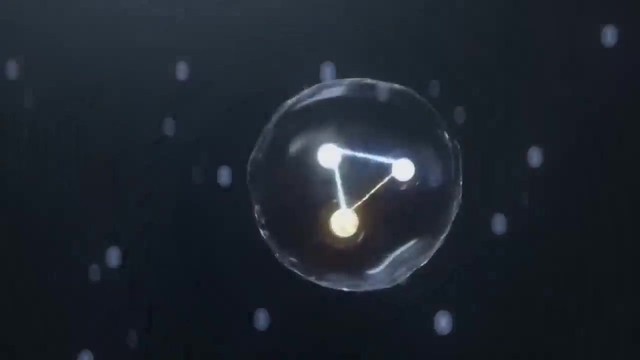 in the world around us. Reflection and refraction form the images of the objects we see, while absorption determines their color and brightness. Unlike light, darkness is not a physical category, but rather a relative state. It's not even that: It is a subjective perception of the state. 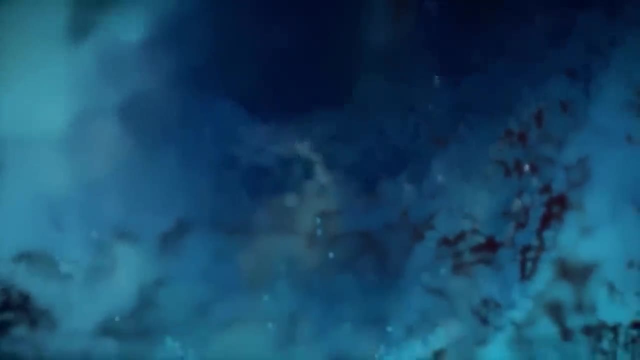 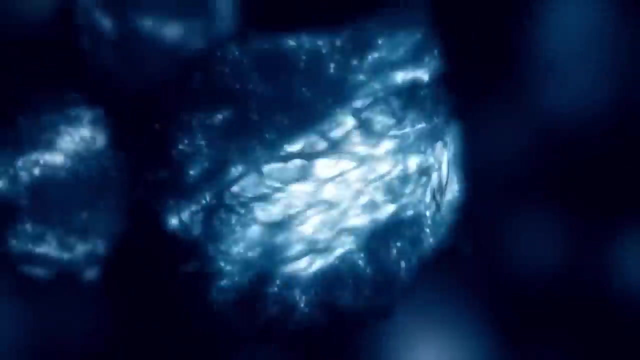 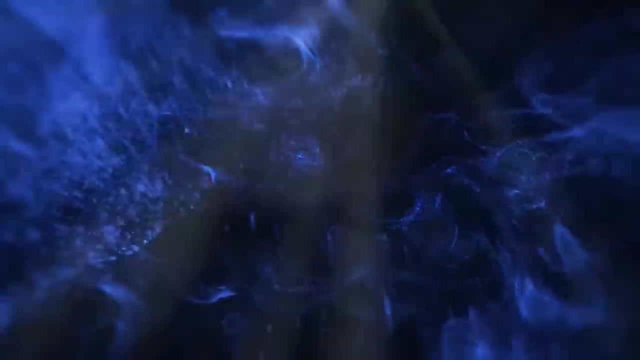 Photons may or may not be reflected. retinal cells may trigger memory processes but cannot explain the subjective experience of darkness, Just as waves cannot be represented by anything more than our experience of color or sound. Our subjective experience changes from time to time. 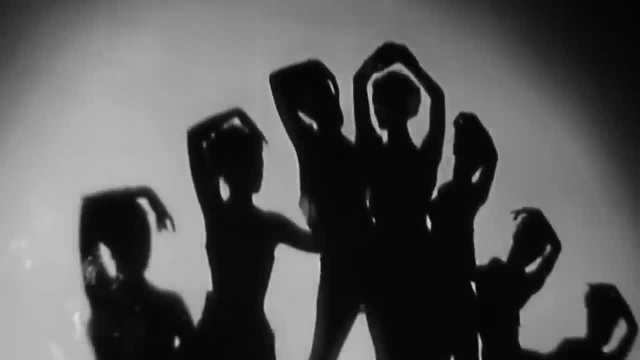 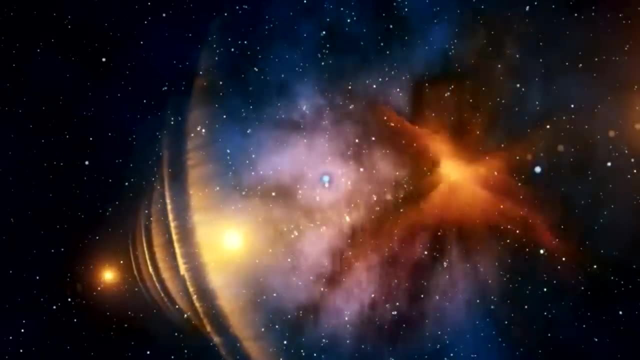 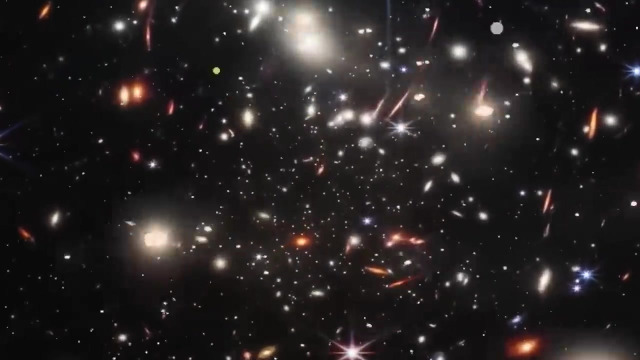 but the individual parts of that experience lie outside of time, And in this sense we can say that darkness itself has no speed. What is speed in the common understanding, And does it exist at all? It presupposes in advance the existence of some space. 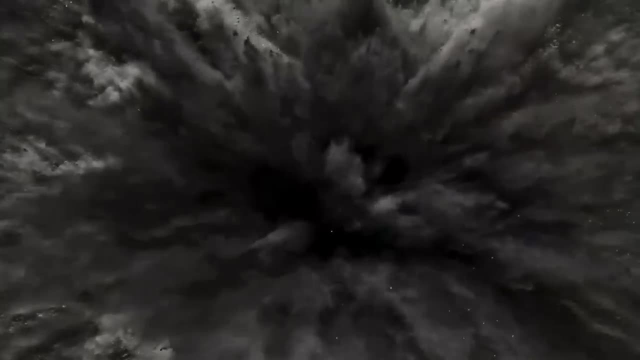 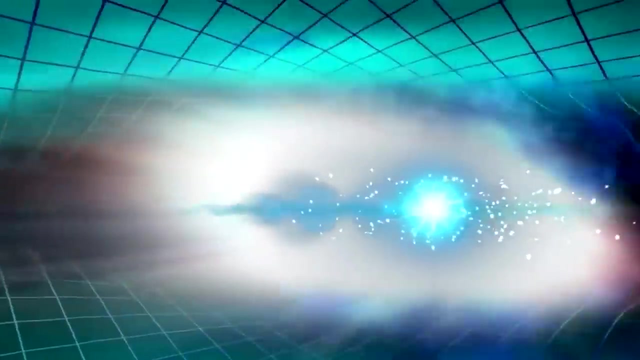 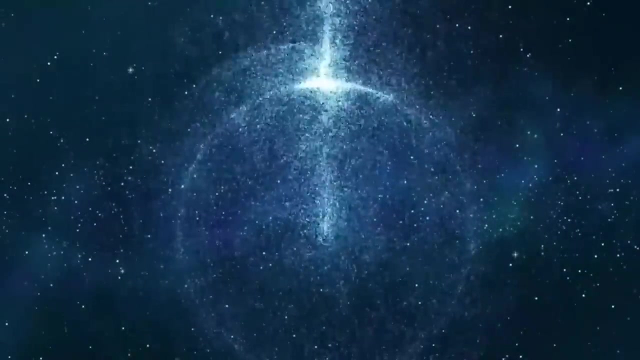 in which it can be measured. However, in the world of quantum physics, where the familiar concepts of conventional physics often become useless, it is believed that space itself is one of the derivatives of a more fundamental level of reality where there are no such concepts as position, distance or speed or speed. 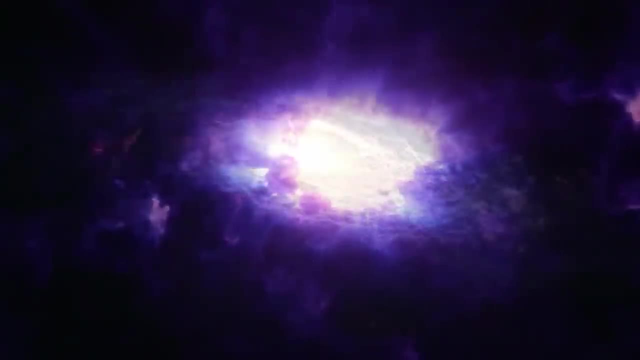 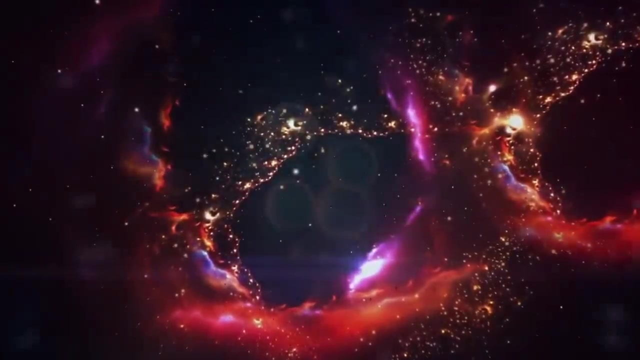 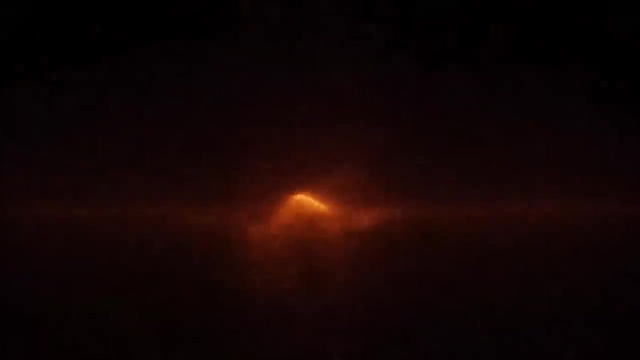 In conclusion, let us try to draw some conclusions and clarify how important and inseparable all the properties of light are. We already know the basic characteristics of light. It is a form of electromagnetic radiation consisting of photons and has the ability to propagate in a vacuum. 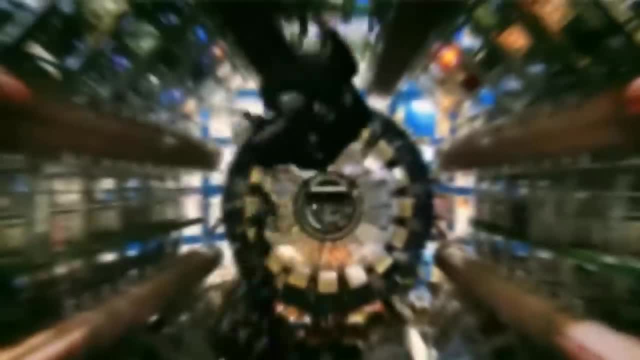 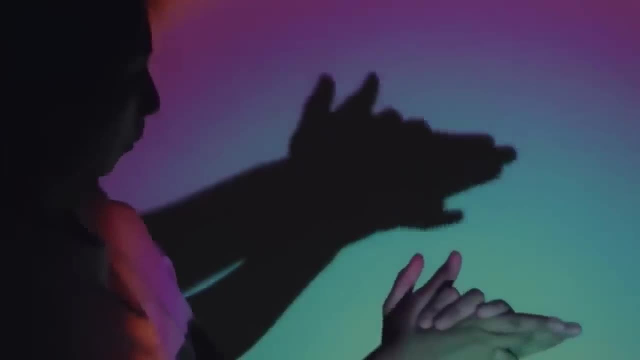 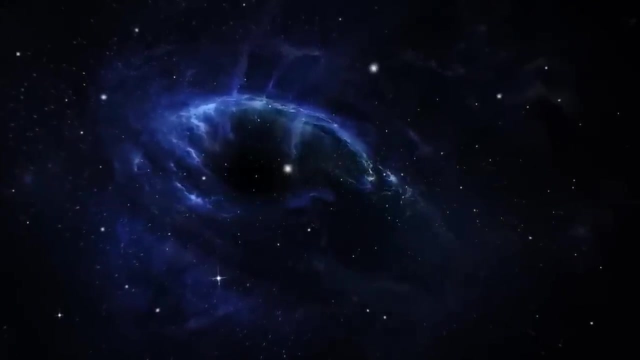 at a constant speed. At the same time, light is often described in terms of its dual nature, having the properties of both waves and particles. This unusual property is not only striking and surprising, but is also an important key to understanding fundamental mechanisms in quantum mechanics. 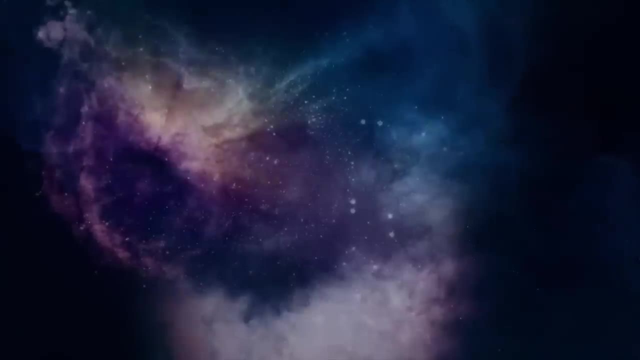 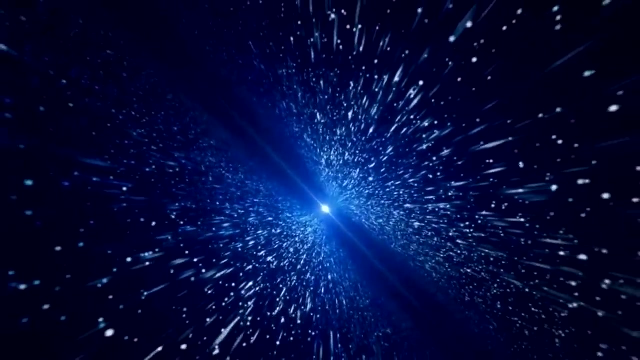 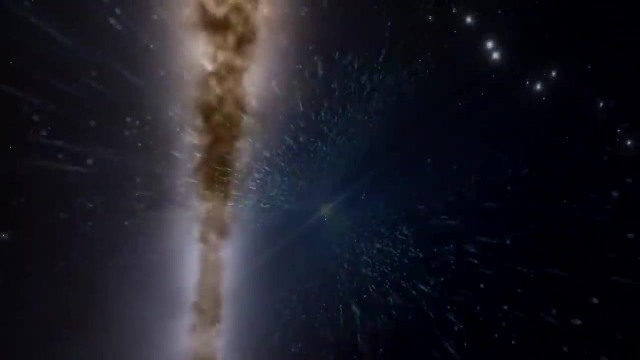 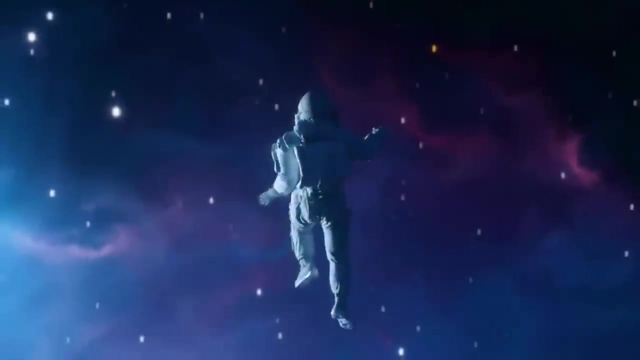 as well as phenomena such as interference, diffraction and polarization in light. Light also plays an invaluable role, not only on our planet but in the universe as a whole: Its ability to deliver information from the farthest reaches of space to create conditions for life on Earth. 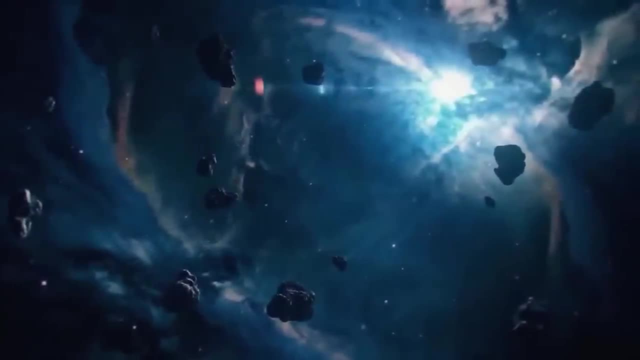 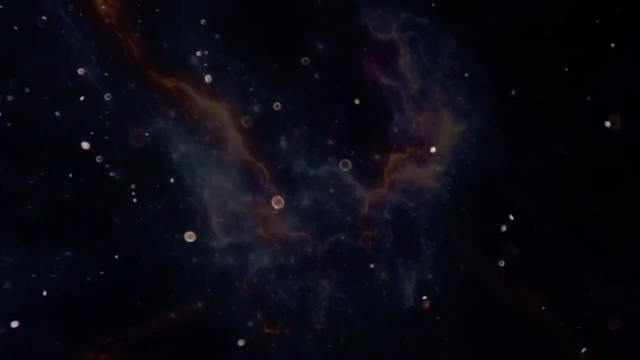 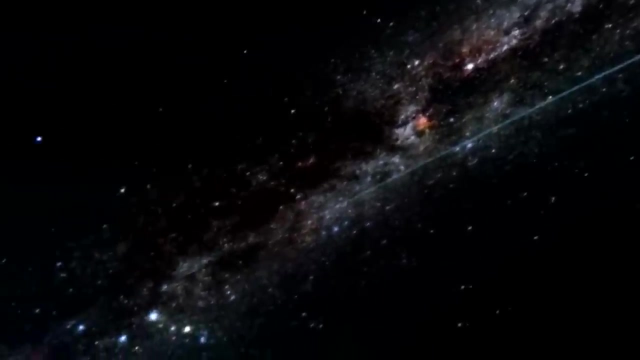 and to serve as a tool for studying and understanding the world around us makes light a true magical phenomenon. We owe it to light for the ability to see and perceive our surroundings. It allows us to admire the beauties of nature, distinguish colors and shapes. 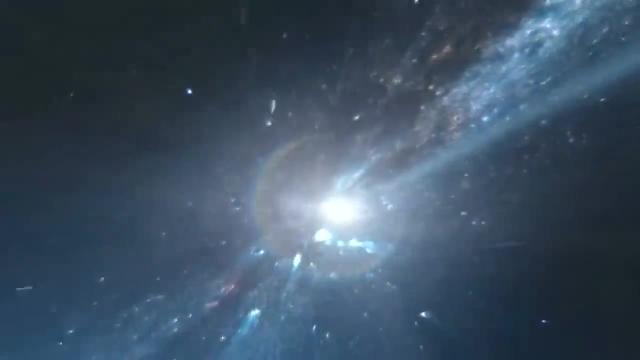 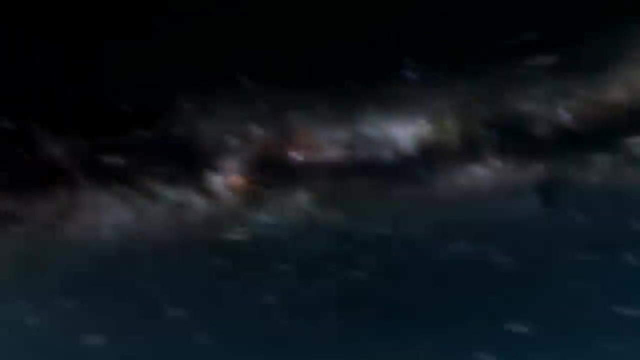 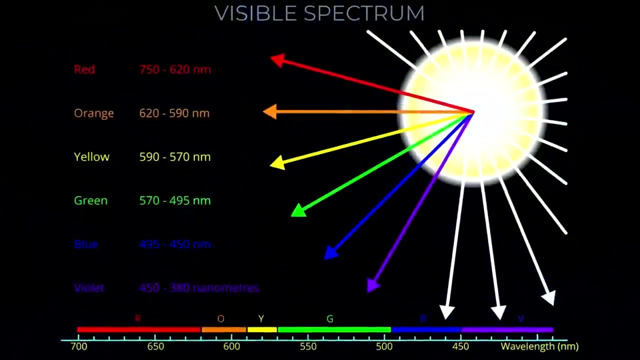 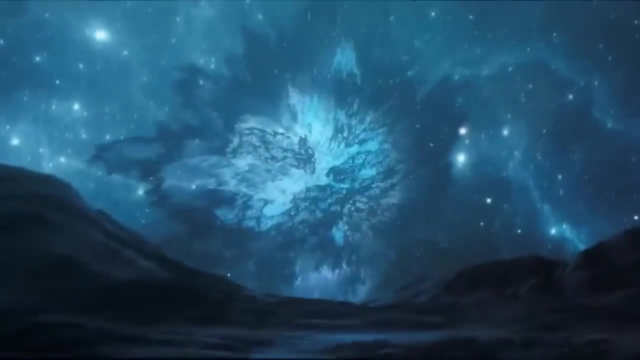 and facilitates our social interaction and communication. Thus, whatever light is by nature, it is one of the most amazing phenomena ever discovered by mankind, But the question of how light originally came to be remains open. The question of how light originally came to exist. 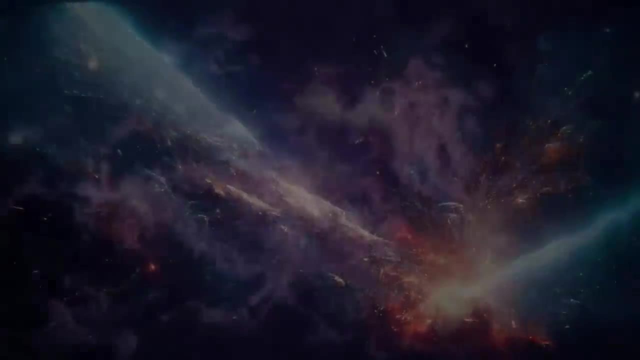 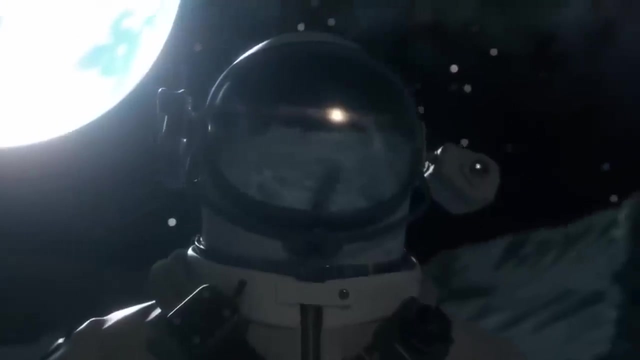 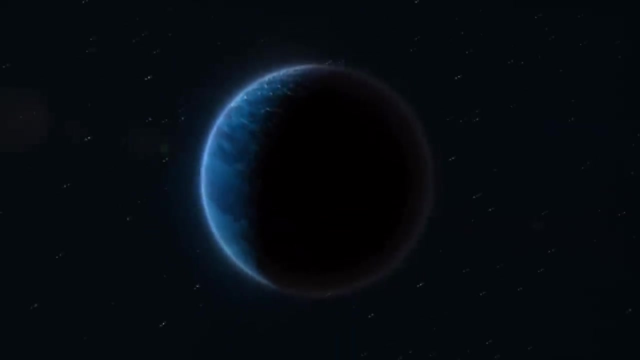 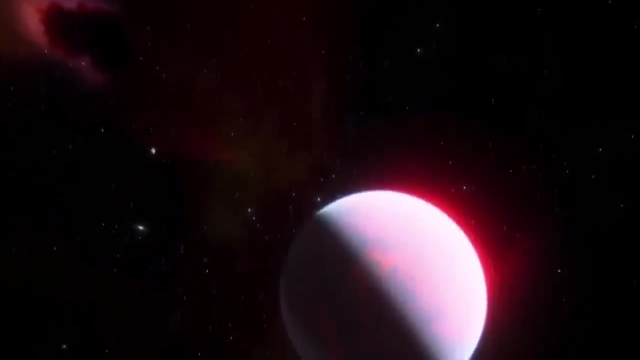 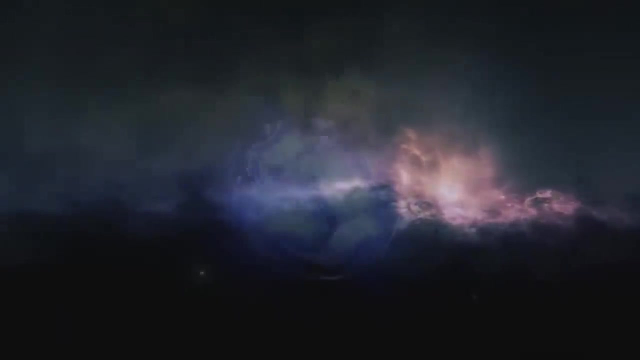 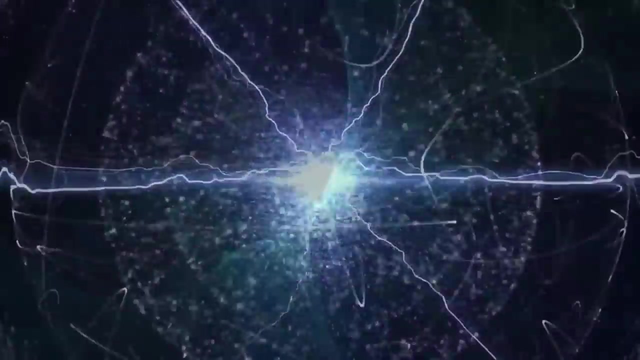 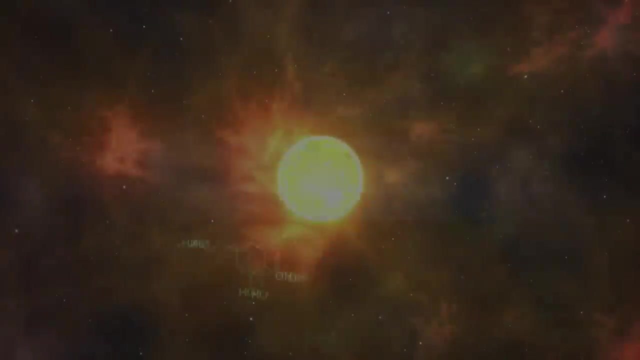 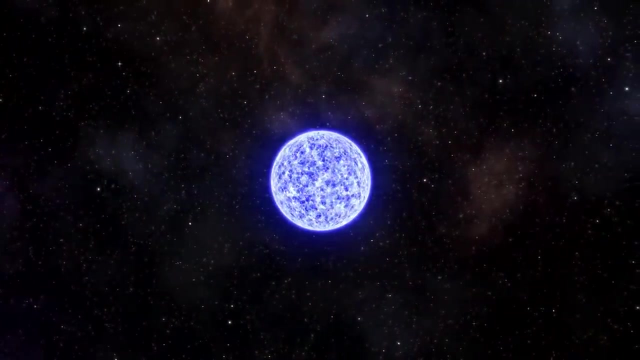 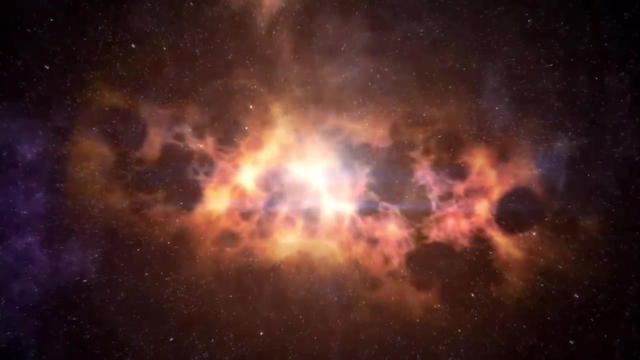 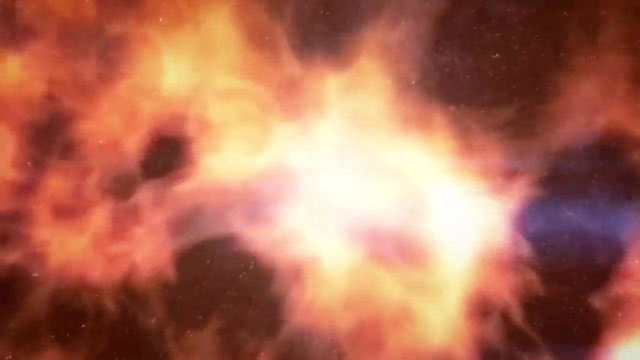 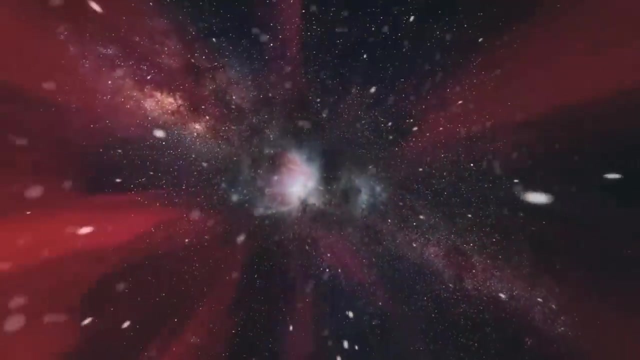 creates a feeling of The birth of stars. Stars is unique and exciting, but it doesn't happen in a moment. The transformation of a molecular cloud into a luminary takes time and, importantly, suitable conditions for this. These dense regions with stars inside look like dark silhouettes against the background. 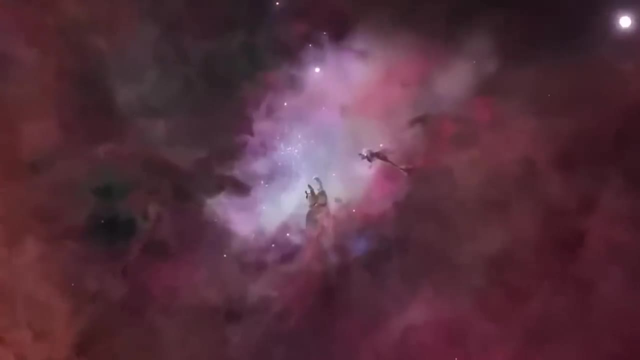 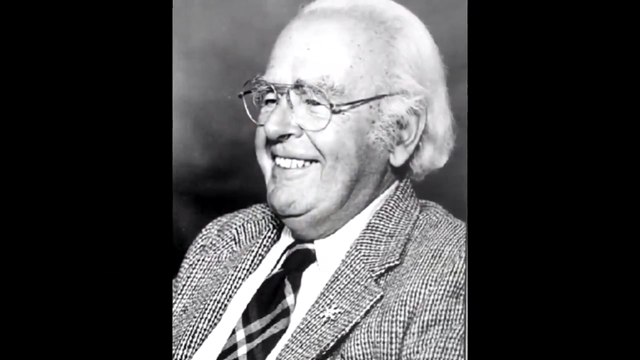 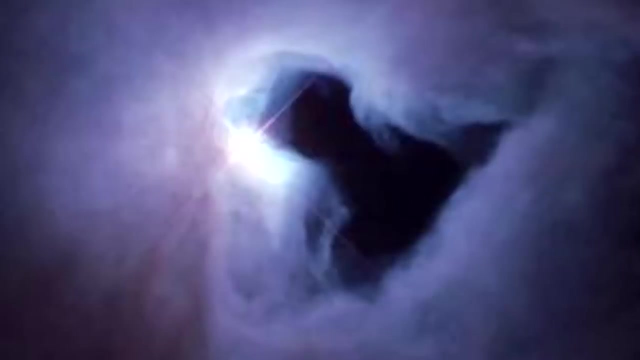 of the rest of the ionized nebula. Such formations are known as Bach Globules in honor of astronomer Bart Bach. Back in 1947, a researcher hypothesized that these clouds were like insect cocoons, And he wasn't wrong. 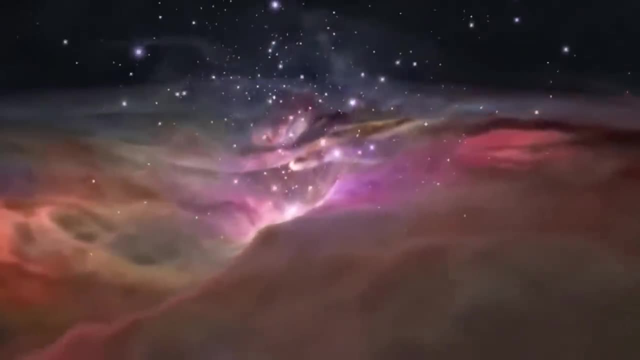 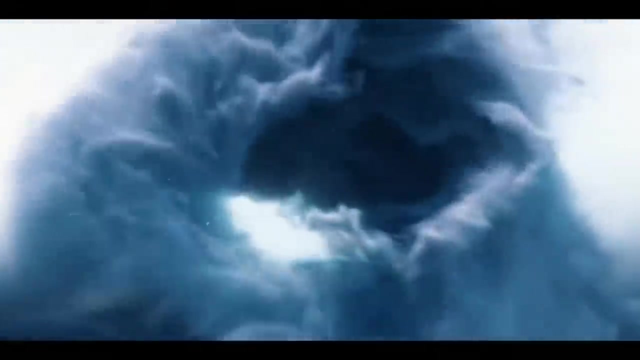 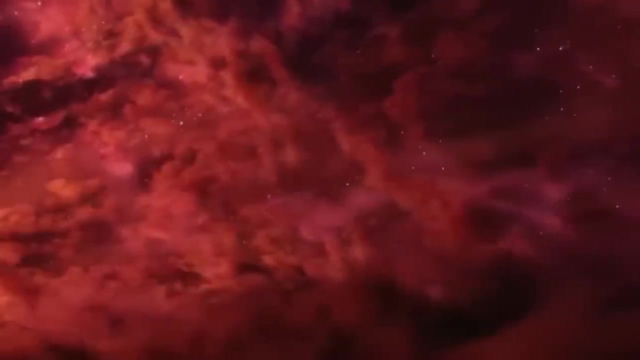 Decades later, we now know that bokeh globules are dense clusters of cold gas and dust living in the interstellar medium, Hiding in the shadow of huge molecular clouds. these seemingly harmless and isolated formations play a key role in the birth of stars. 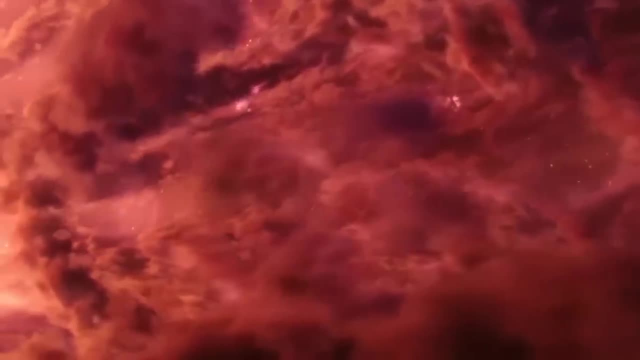 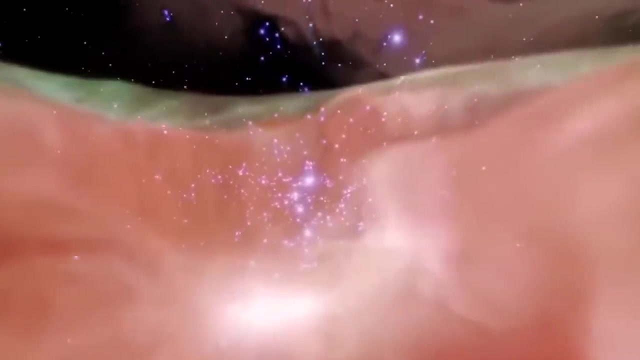 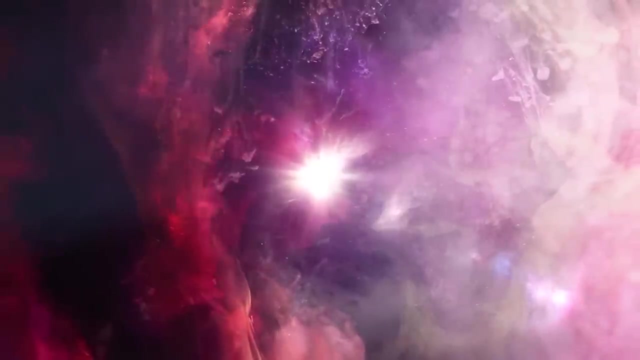 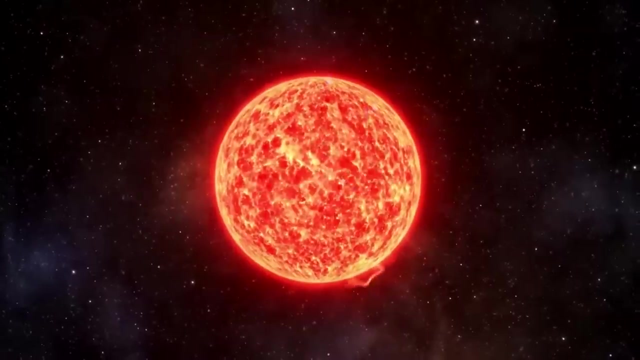 Yes, inside these dark cocoons, the smallest gravitational inhomogeneities gradually accumulate matter, increasing their mass and gravitational attraction. Over time, the particles of matter combine into dense nuclei that contract under the influence of their own gravity. As the infallible force of gravity condenses matter, a nuclear chain reaction begins as. 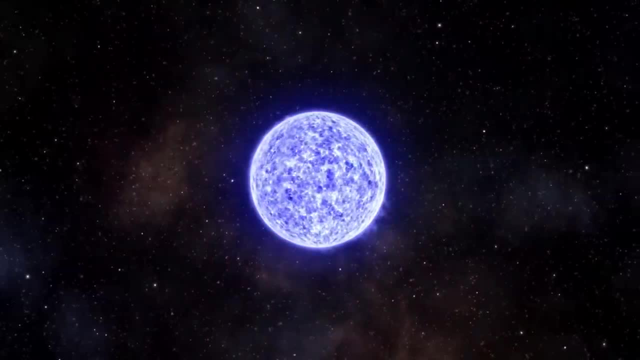 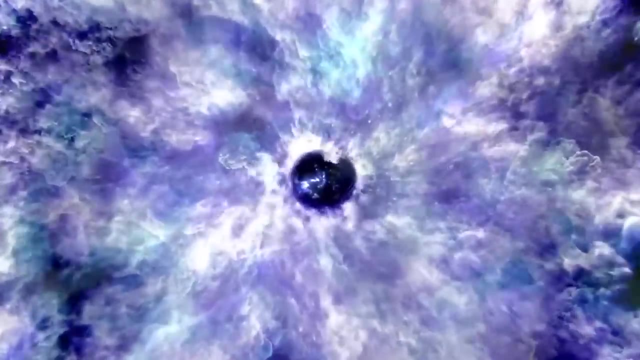 a result of an increase in gravity. The nuclear chain reacts to the another and the particles of matter are then absorbed into the nucleus. The nuclear chain reacts to the other and the particles of matter are then absorbed into the nucleus. This explosive phenomenon known as nuclear fusion releases a staggering amount of energy. 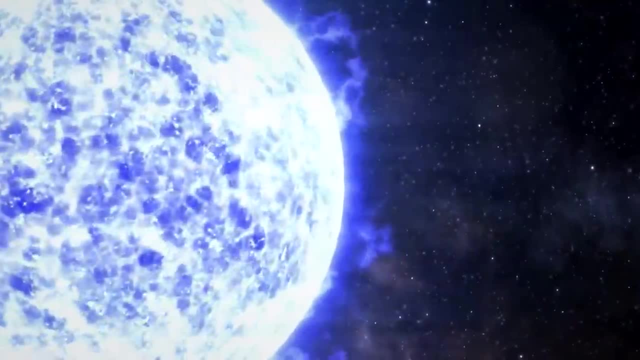 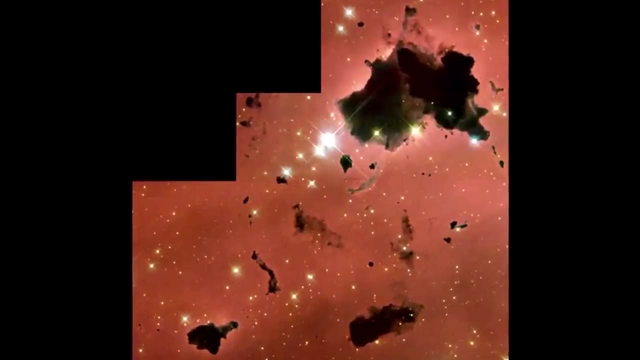 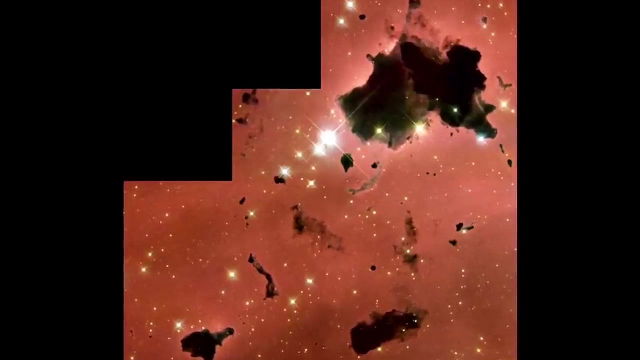 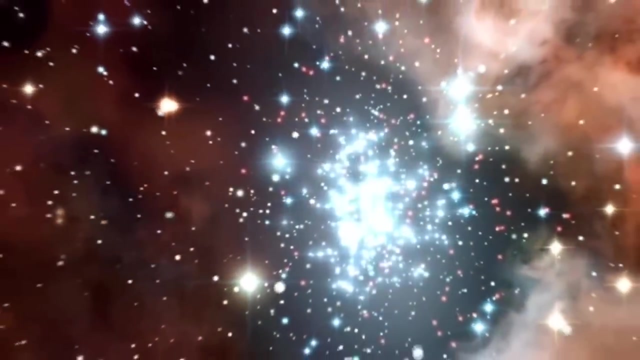 and marks the birth of a new star. Today we know that the Boca Globules are one of the coldest gas formations. Their temperature, determined by the radio emission of molecules, does not exceed an average of 255 degrees Celsius, degrees Celsius below zero. The bulk of the gas is a mixture of molecular hydrogen and helium. 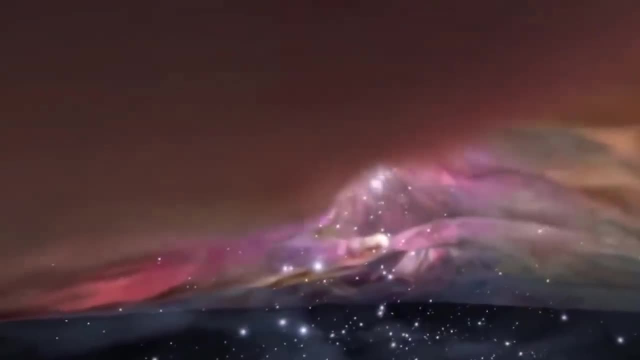 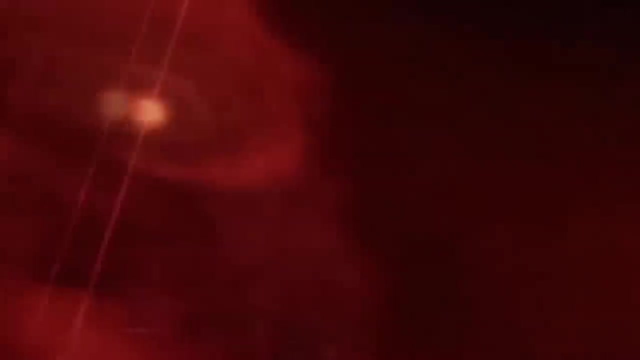 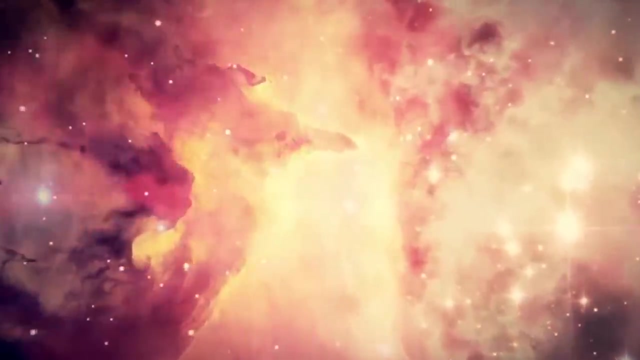 The concentration of atoms and molecules in these formations is higher than in ordinary clouds of interstellar gas. It increases towards the center and averages several thousand molecules per cubic centimeter. The mass of dust is about a hundred times less than the mass of gas, But it is the dust that provides the opacity of the globules. 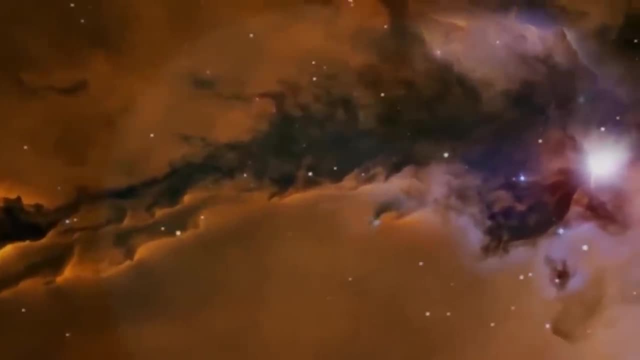 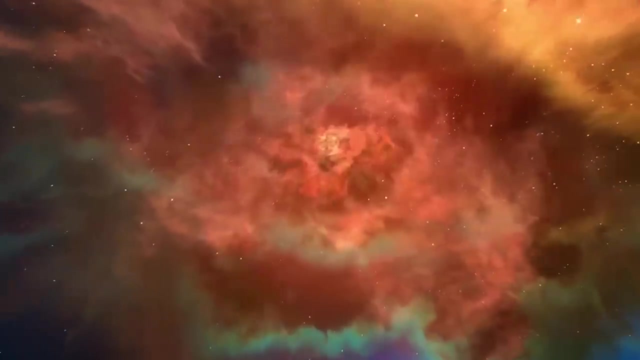 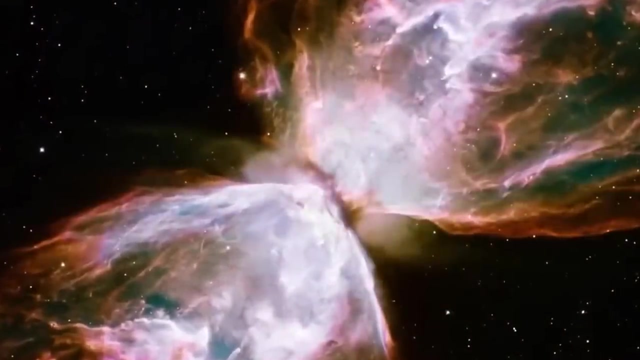 because of which they are visible as dark spots. Due to the low temperature in the most massive globules, the process of gravitational condensation of matter, leading to star formation, becomes possible. This is confirmed by the discovery of sources of infrared radiation in the bowels of formations. 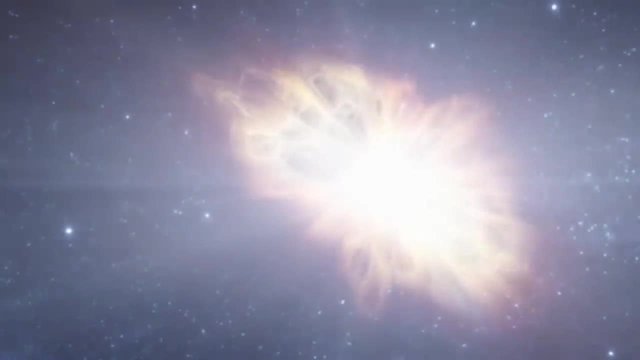 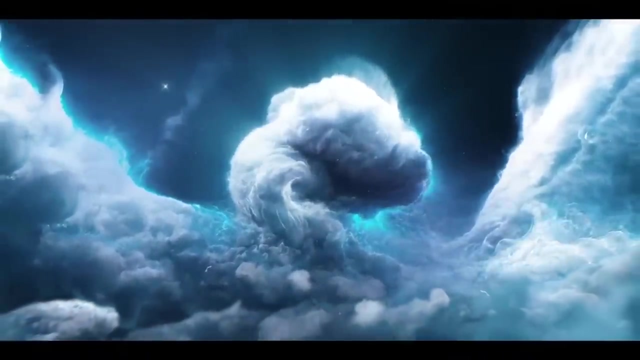 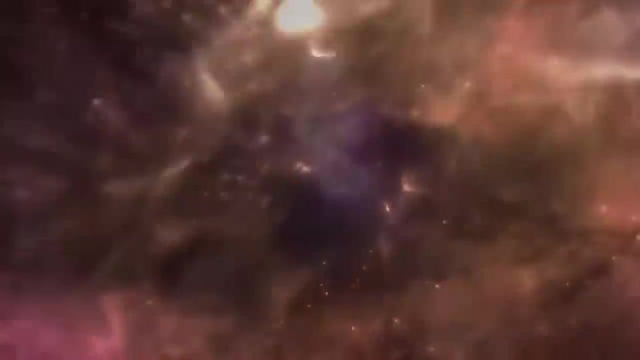 The appearance of infrared sources is associated with the Fraser algorithms, the heating of dust by the radiation of one or more born stars, the visible light of which does not penetrate through the dust. The high density is justified by the fact that substances such as carbon and hydrogen 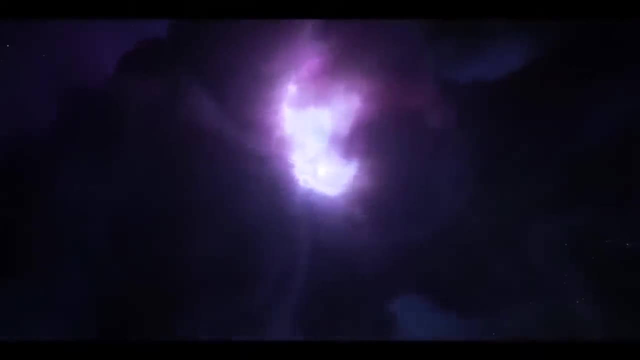 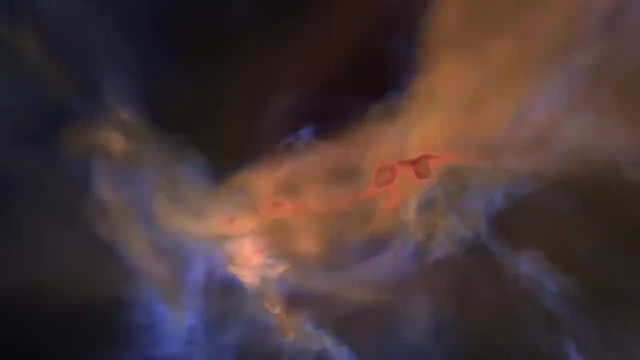 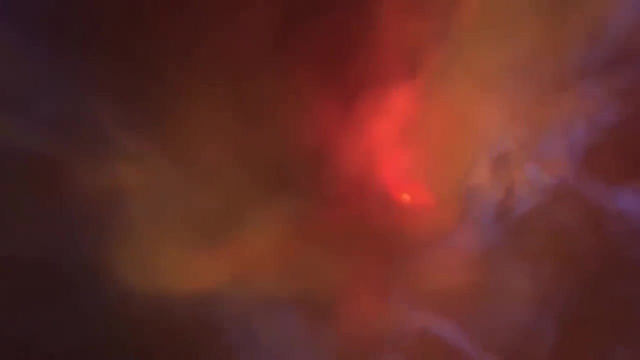 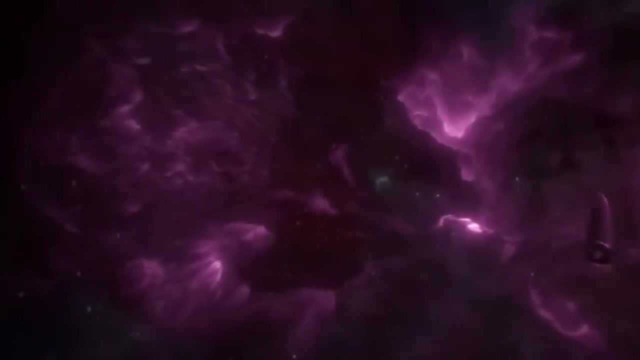 under the influence of low temperatures, begin to combine into molecules from individual atoms. Thus, the fusion of a denser substance into molecules is also the cause of high density. These cosmic clouds are almost completely dark and unsightly even for the most modern optical instruments, which is their most famous characteristic feature. 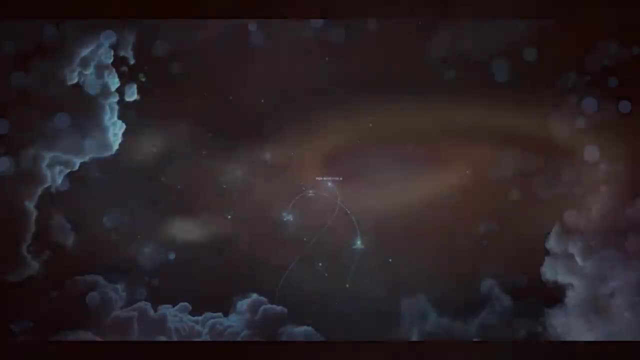 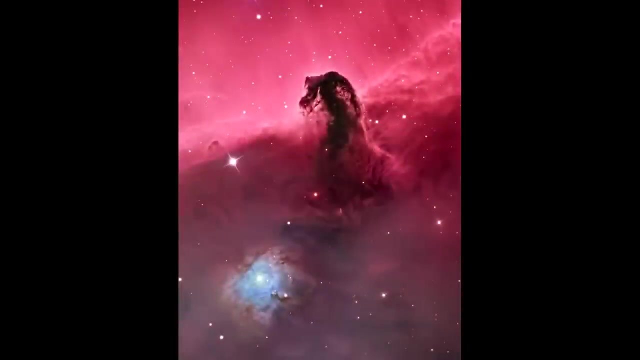 At the moment, no less than 349 dark nebulae have been discovered. The most famous examples of them are the Horsehead Nebula, the Coal Sack, the Snake, fragments of the Eagle Nebula and the Bernard 68 molecular cloud. 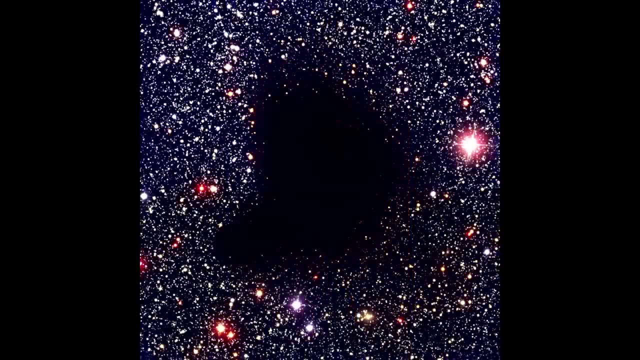 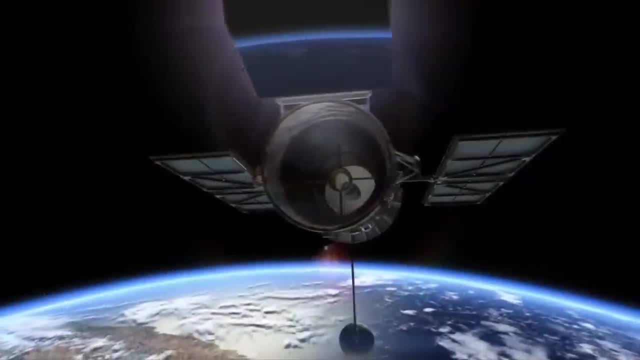 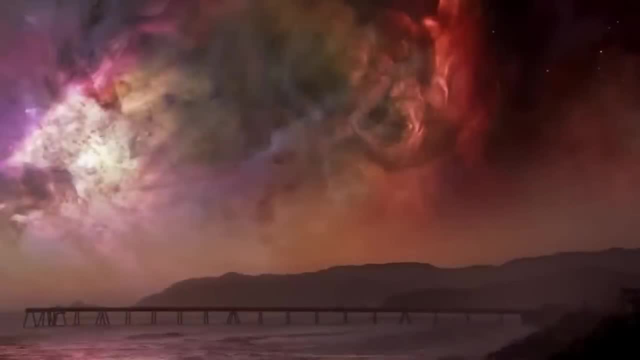 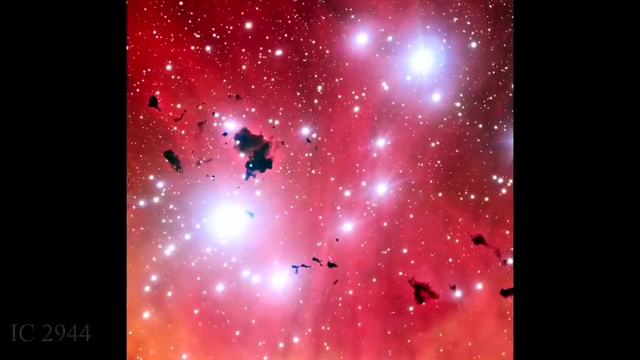 Thank you for watching. Most of the globals have been discovered and studied by astronomers using modern telescopes, in particular the Hubble Orbital Telescope. We propose to consider some of them in more detail, for example, detailed images of the area of the AISI 2944 or a running chicken. 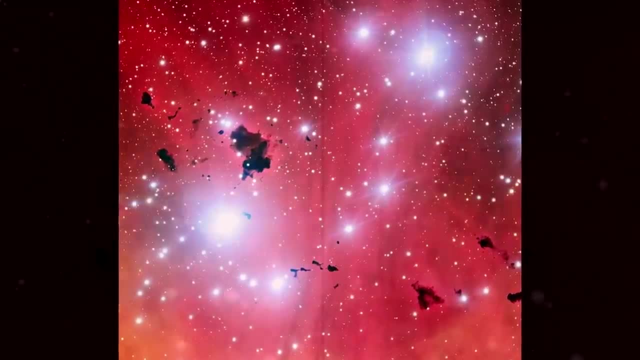 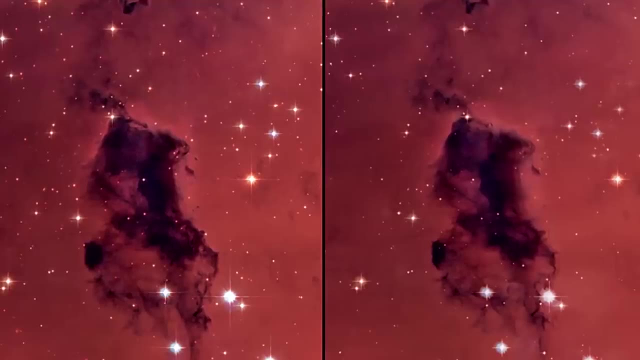 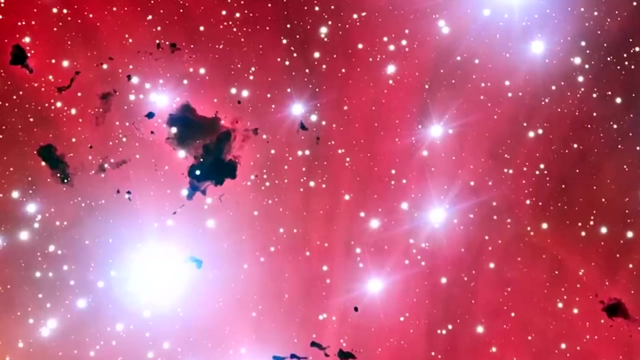 Where he is running to and why is truly unknown. The mysterious region is located in the continental constellation Centauri, at a distance of about 6,000 light-years. Here we observe dense, opaque dust clouds that stand out clearly against the background of bright stars. They 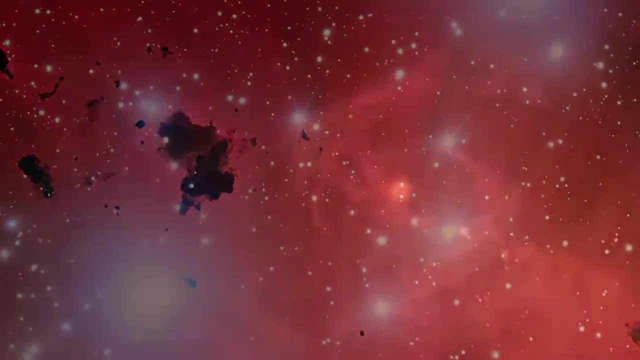 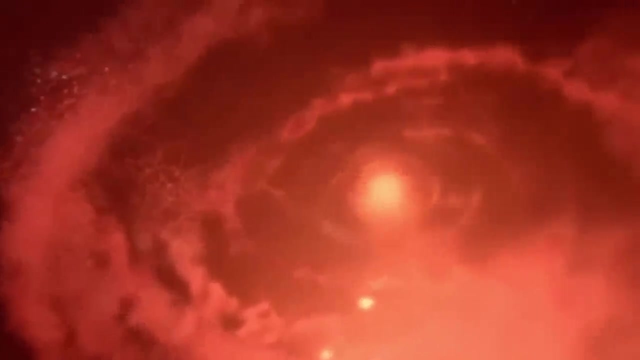 are filled with gas and dust, which is illuminated and heated by the radiation of the stars of the scattered cluster. These stars are much hotter and more massive than our sun, But in the constellation Cepheus, located at a distance of about 30,000 light-years, the stars are much hotter and more massive than our sun, But in the constellation Cepheus, located at a distance of about 20,000 light-years, the stars are much hotter and more massive than our sun, But in the constellation Cepheus, located at a distance of about 20,000 light-years, 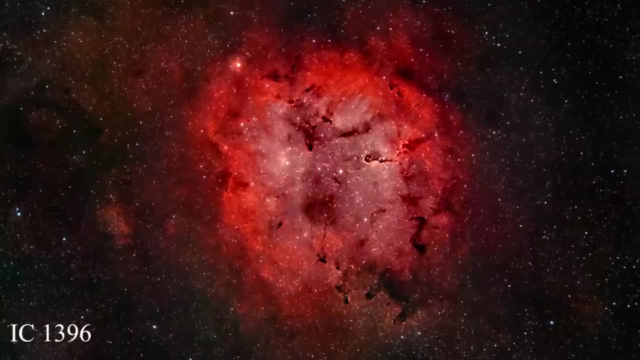 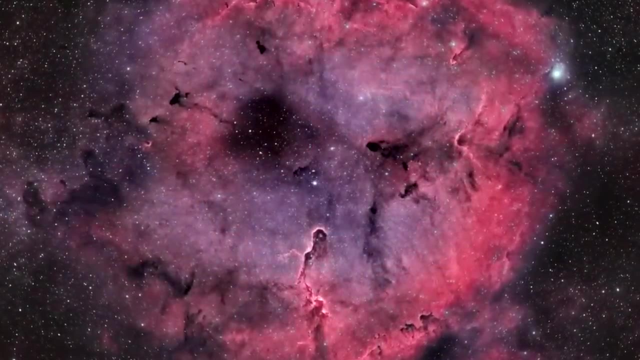 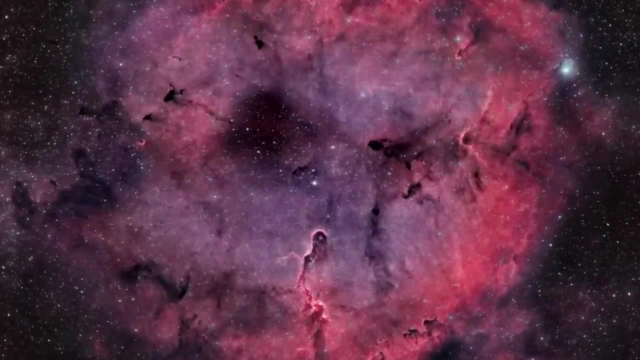 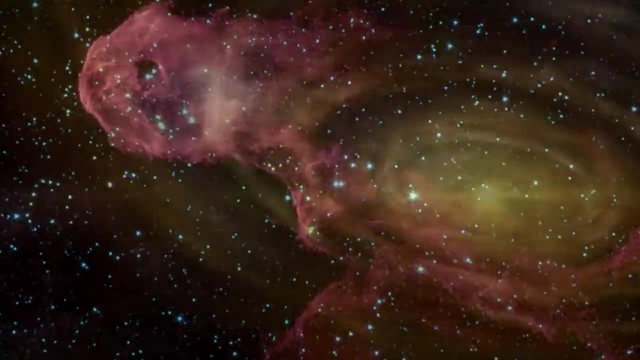 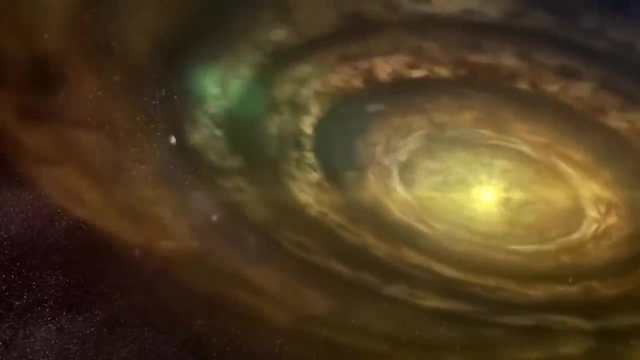 nine. Among the intriguing dark figures in this area, the elephant trunk nebula looks not only unusual but even sinisteremberg Fragrance. Nebula, Elephant間, Nebula, Ele hubs, Nebulas, Nebula, Ele, inside Nebula, Ele, outside New New, New New. The high-energy light emitted by this star separates the dust in a dark comet-like region. 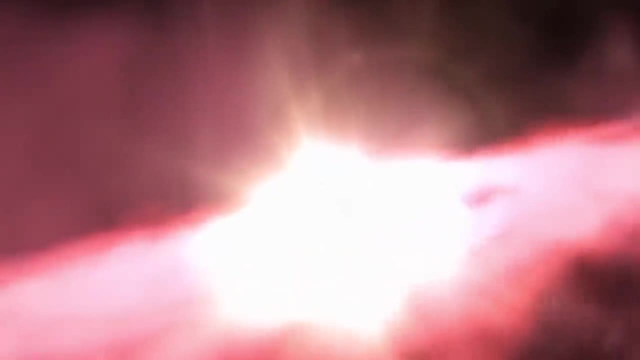 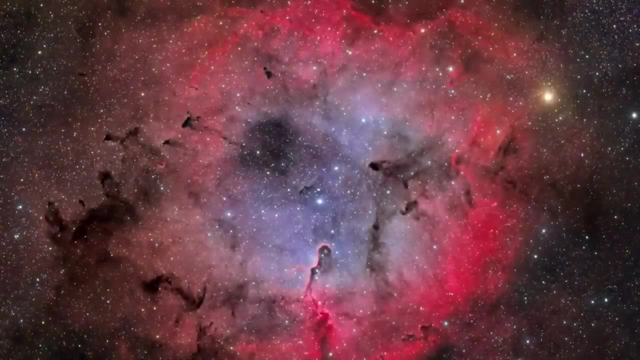 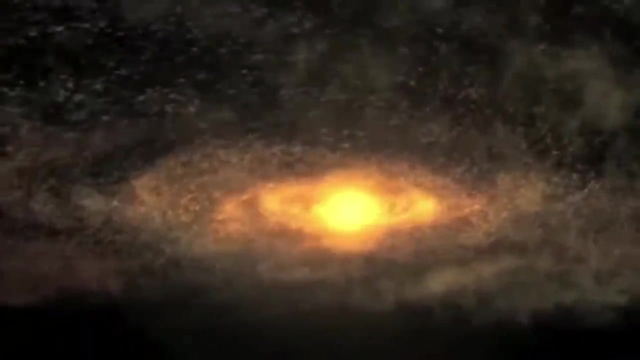 The wind jets from. the particles ejected by this star also repel the surrounding gas and dust. And there are many other smaller, irregularly shaped globules in the entire emission nebula which are likely to be destroyed over time. Consider the following cosmic formation: 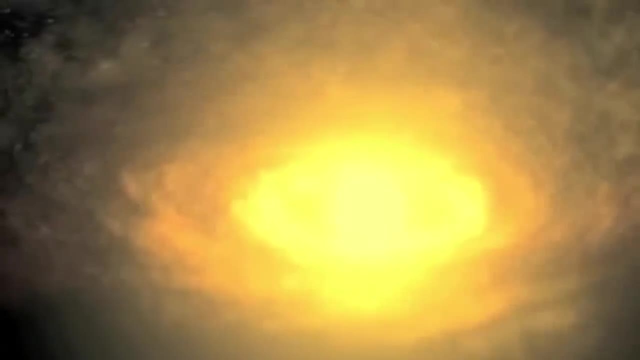 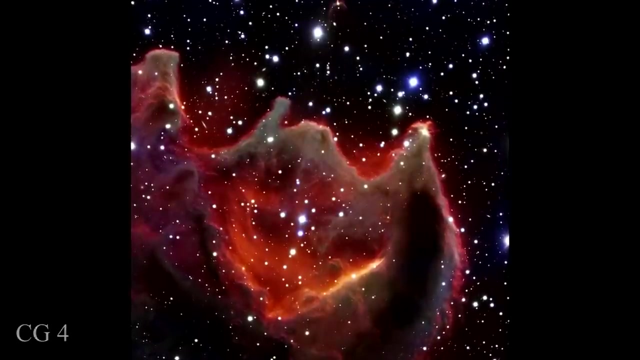 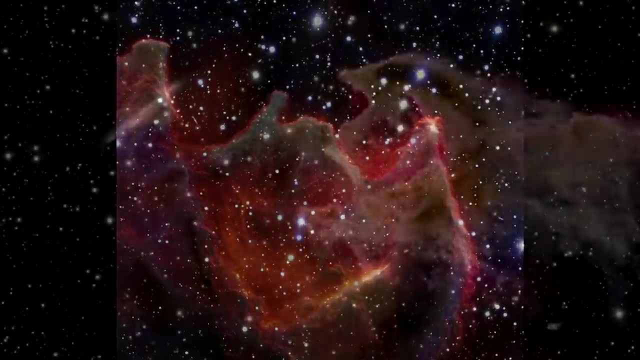 This is another comet-like globola, located in the region of star formation known as CJ4 in the constellation Corma, 1,300 light-years away from us. The coma-like globola is named because its shape is similar to the shape of a comet or. 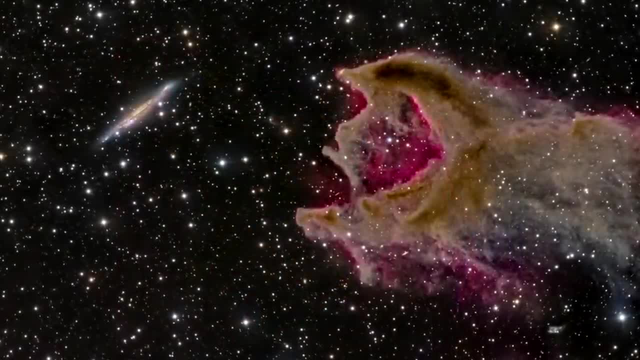 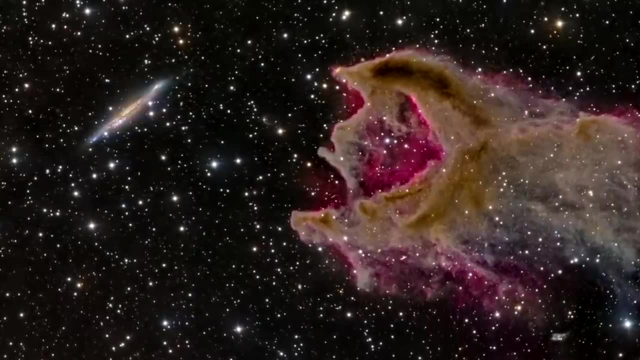 a giant space worm from a dune: A dense head formed of gas and dust with a diameter of about 1.5 light-years and an elongated, faint tail about 8 light-years in length. The form of the cone is marked by the arrow pointing down from the dune, pointing away. 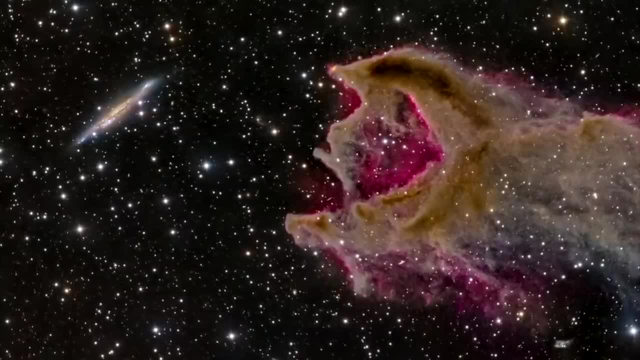 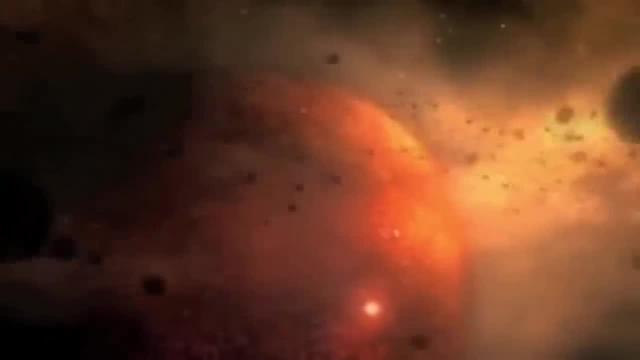 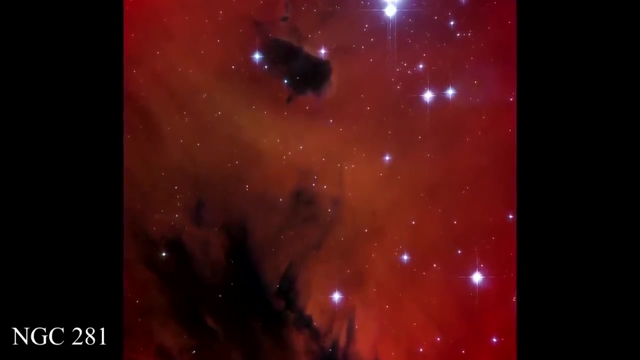 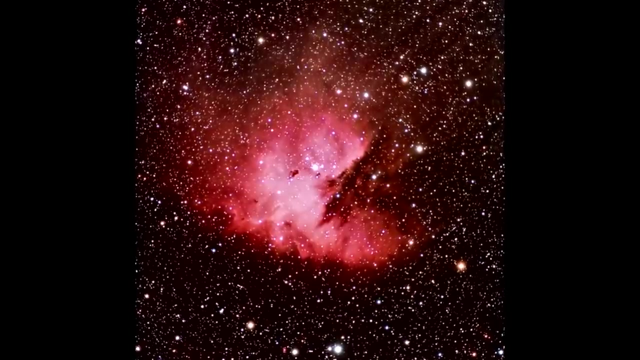 from the supernova remnant. Inside are bright young stars which apparently caused the destruction of the formation, And another interesting place in space named by NBC 281, or PACMAN for short, because of its shape, which is visible in the image with a large field of view. 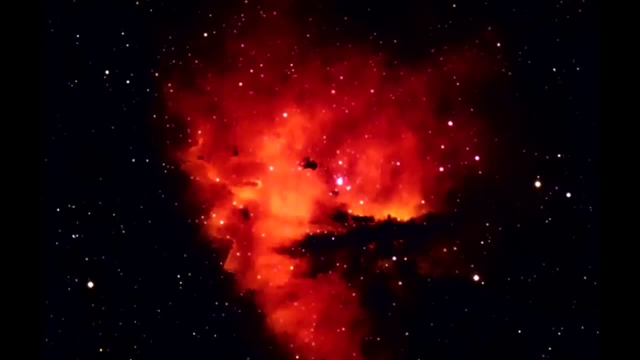 The Large Cosmic Head. The Large Cosmic Head is located at a distance of 1.5 light-years from us. This is a tropical deity that is called the Gaea, of about 10,000 light-years in the constellation Cassiopeia and includes a small scattered 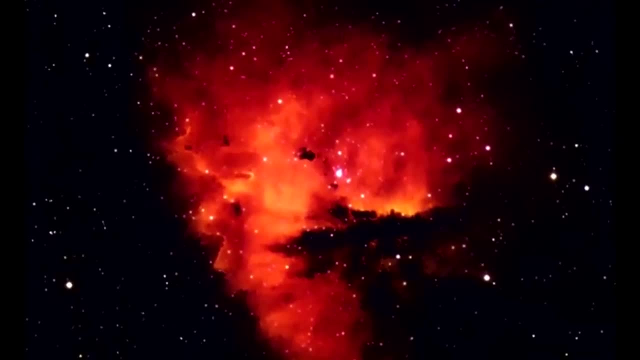 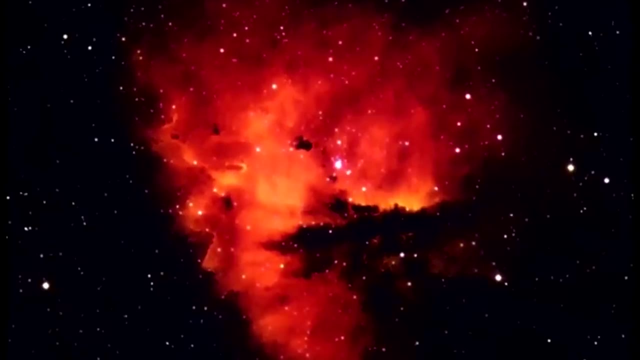 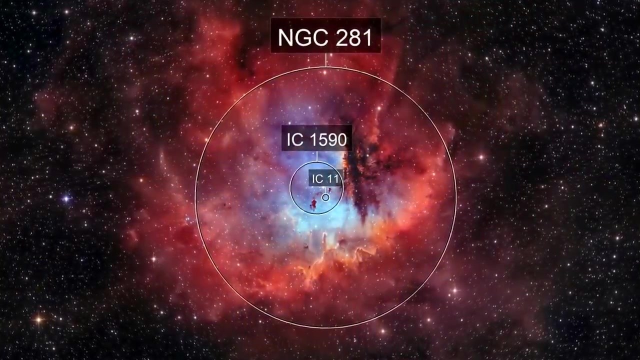 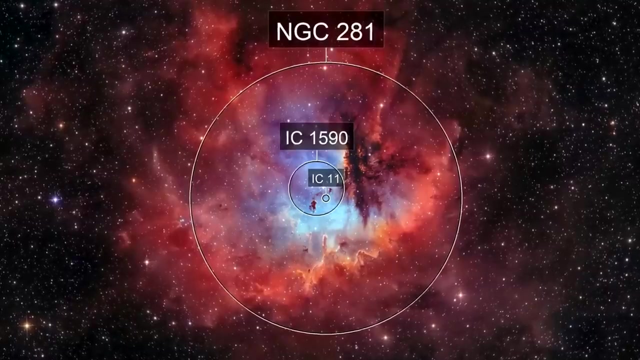 cluster of stars, a glowing reddish emission nebula, extended areas of dust and dense gas dust formations. The next contender with an unusual shape, This is the scattered star cluster AIC 1590 in the central region, which has formed over the past few million years. 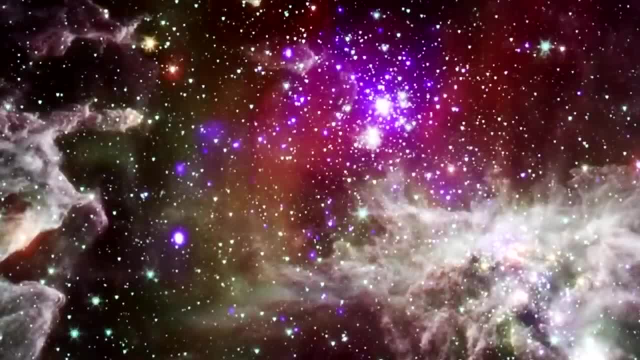 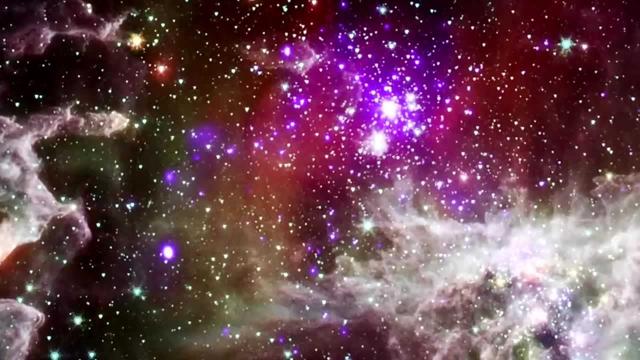 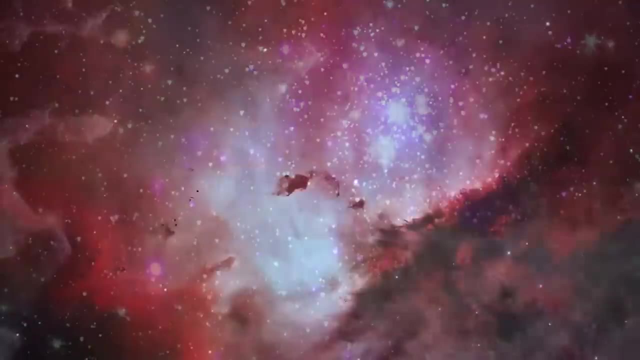 The brightest star in this cluster is a multiple system. Its radiation ionizes the gas in the nebula and therefore acquires a reddish glow. Dark globals of the side, clearly visible against the background of a bright nebula. Sometimes you can see objects coming from. 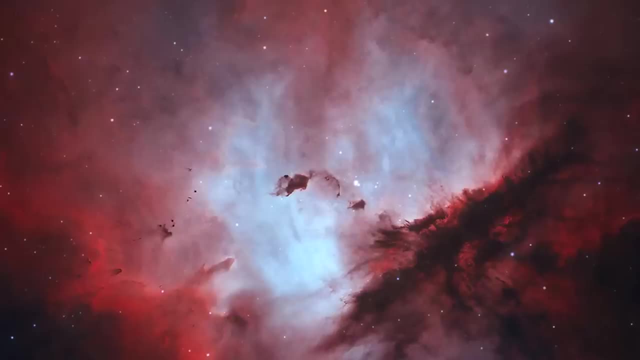 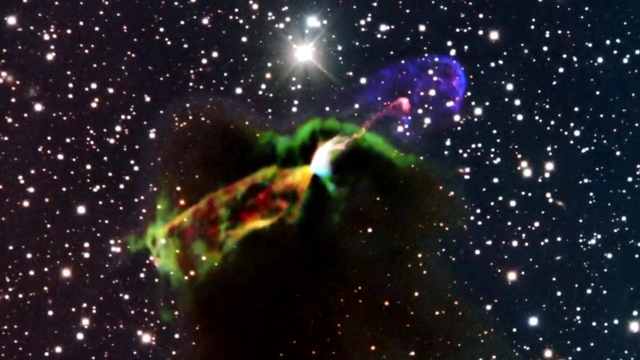 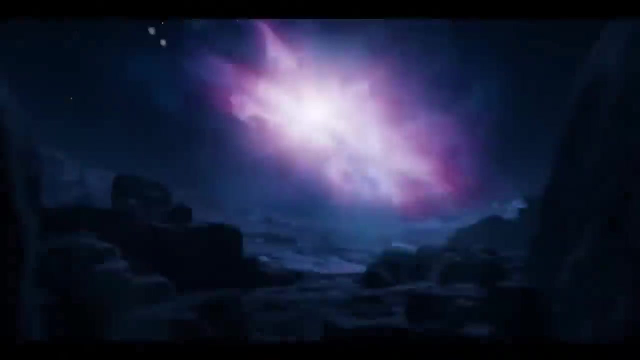 the globals themselves called herbivores. Herbiguero. These are small areas of nebulae associated with young stars. They are formed when the gas ejected by these stars interacts with nearby clouds of gas and dust at speeds of several hundred kilometers per second. 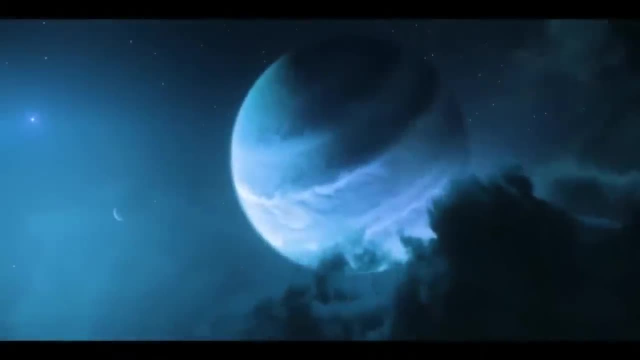 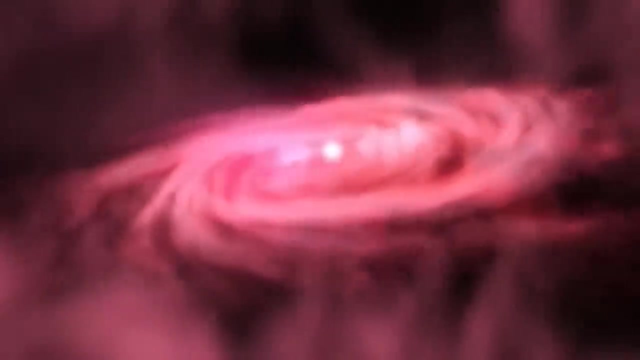 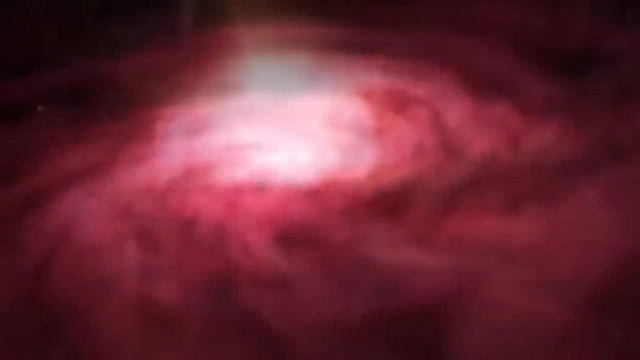 Herbiguero Objects Characteristic of Star Formation Regions. Sometimes they are also observed near single stars elongated along the axis of rotation of the ladder. These are temporary formations, the maximum duration of which is only a few thousand years. The images taken even at relatively small intervals show their high rate of penetration. 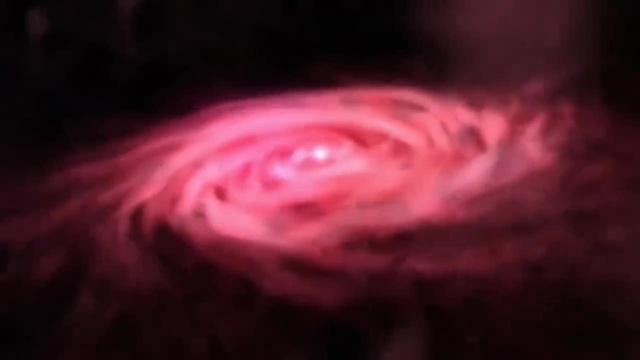 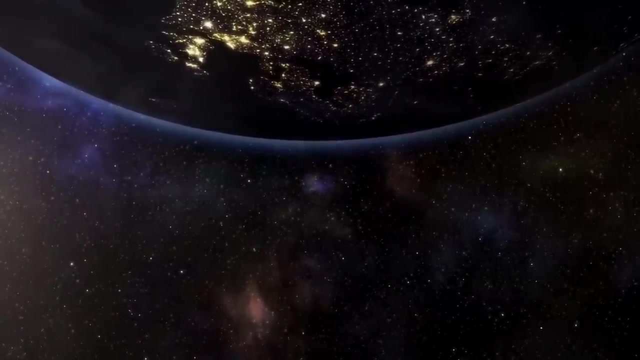 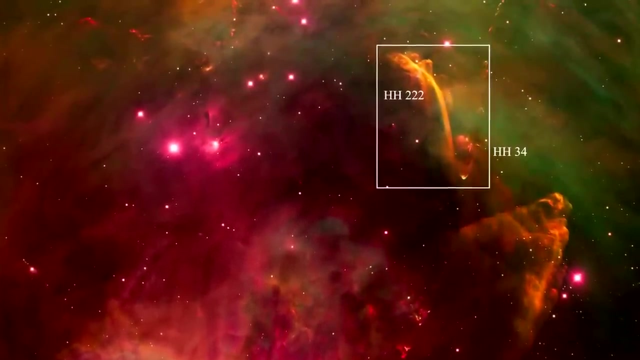 into interstellar clouds of gas far from the parent star. One of the most exciting such objects is located in the famous Orion nebula. In this photo, obtained by adding three images at different wavelengths, the waterfall nebula, or HH222, is visible. 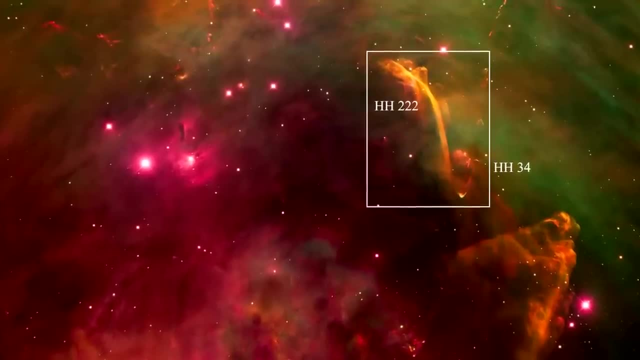 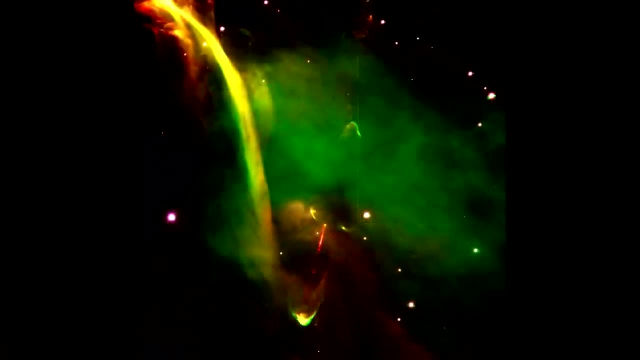 visible a yellow-green stripe running down from the upper left corner. It is located in the giant gas field cloud of Orion, at a distance of about 1,500 light years from us, And the length of the waterfall is about 10 light years. 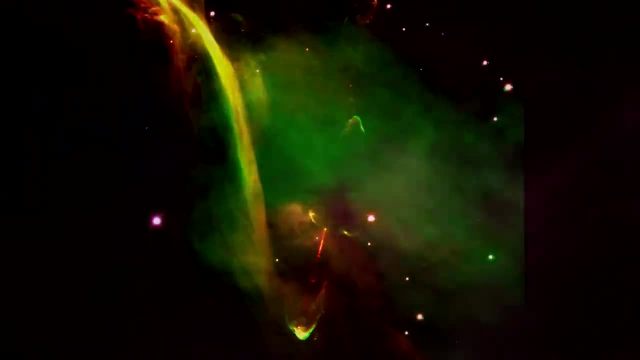 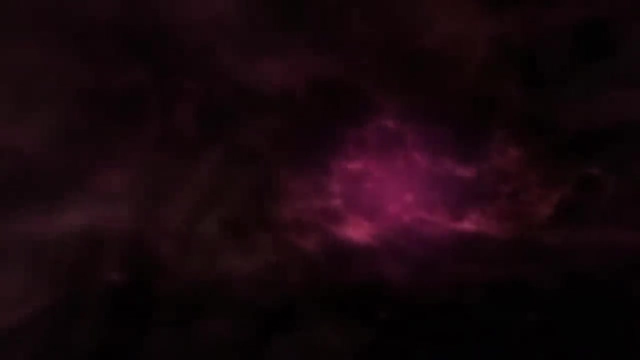 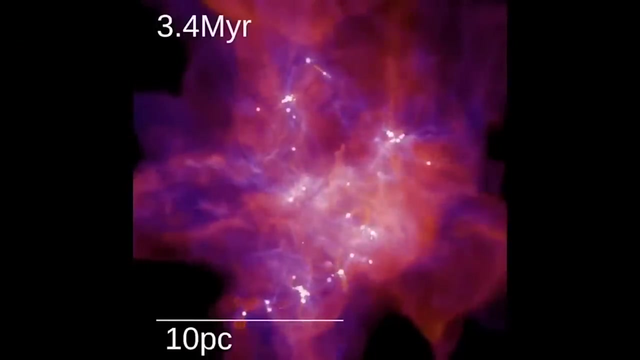 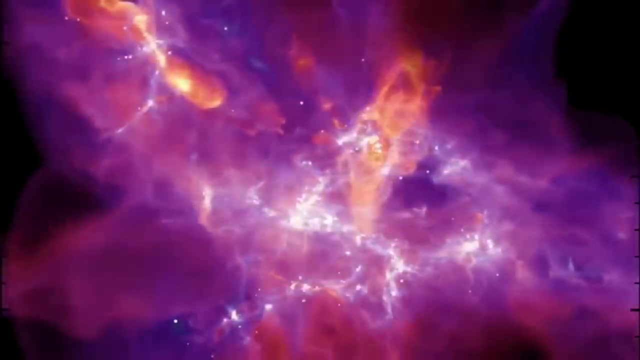 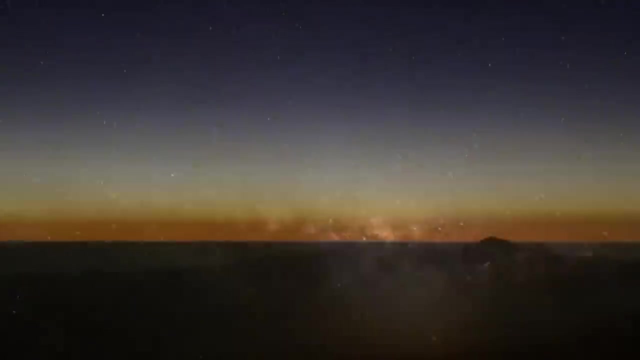 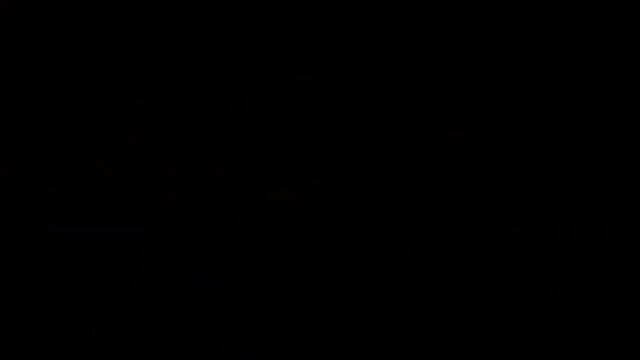 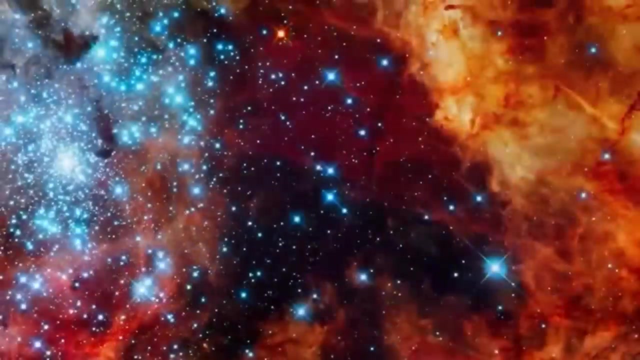 Yes, space is full of mysteries. In conclusion, summing up, it can be noted that the study of globals and their role in the birth of stars is of great importance for our desire to understand the cosmos. Thank you very much for your attention. see you in the next video. 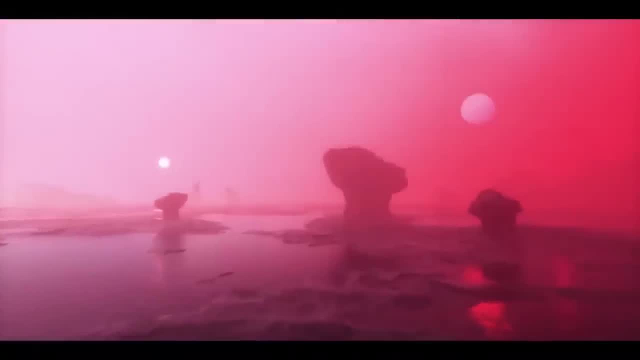 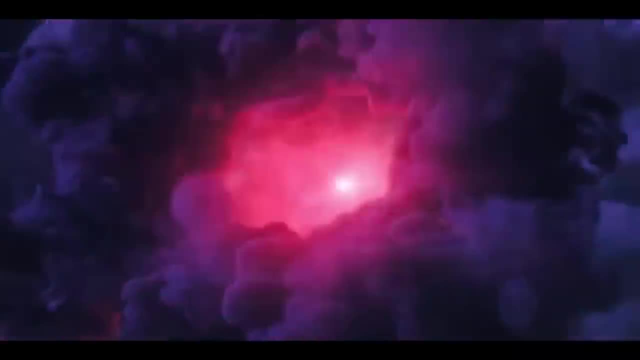 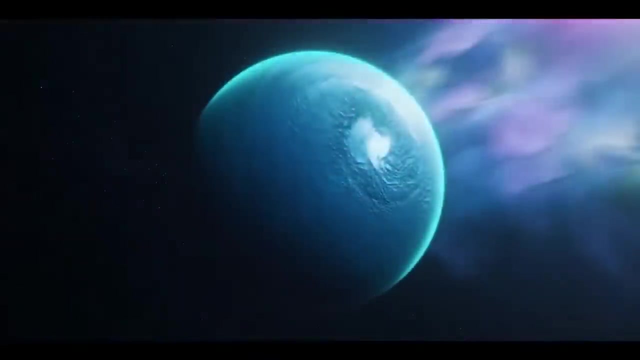 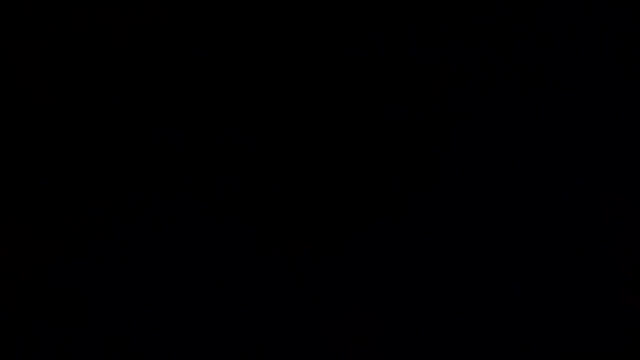 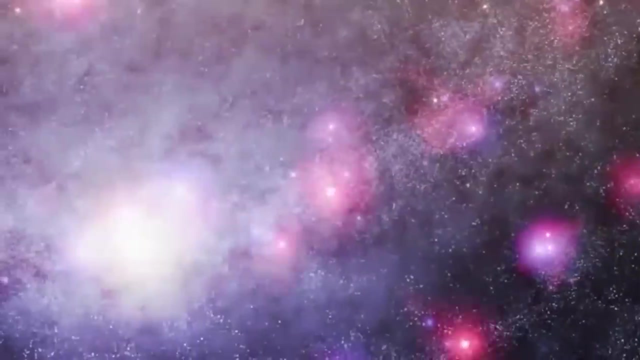 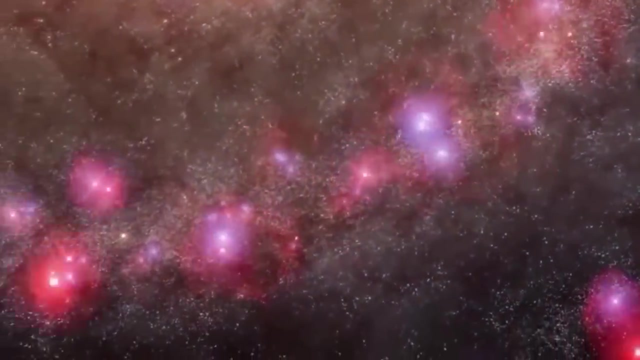 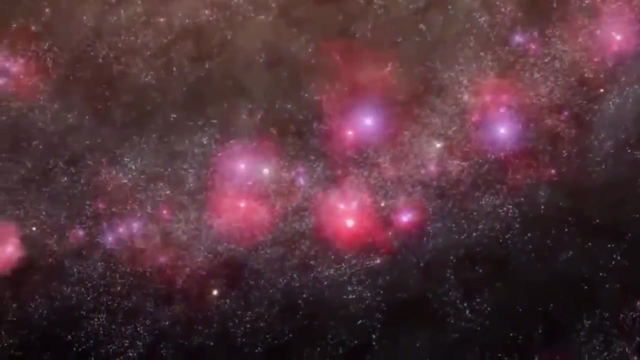 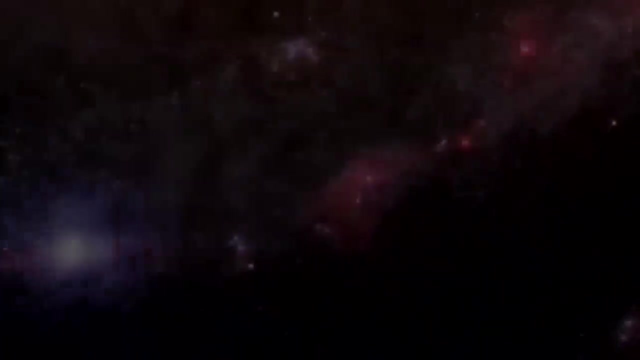 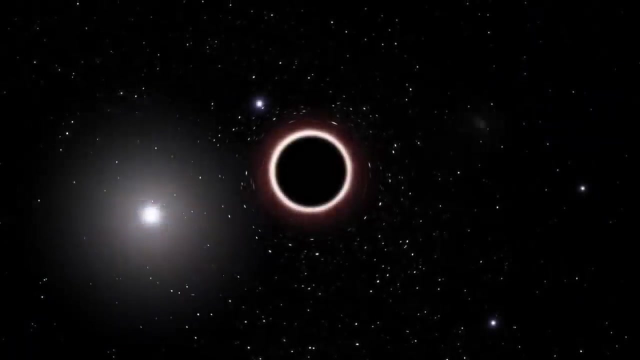 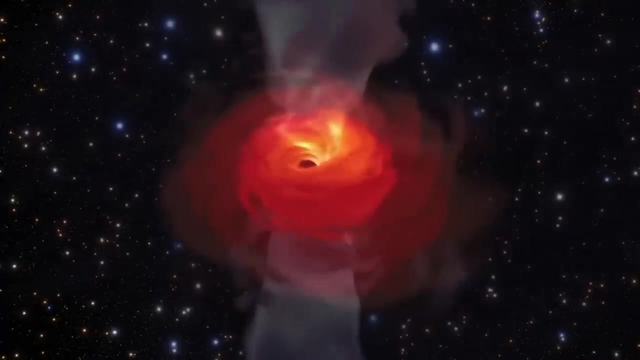 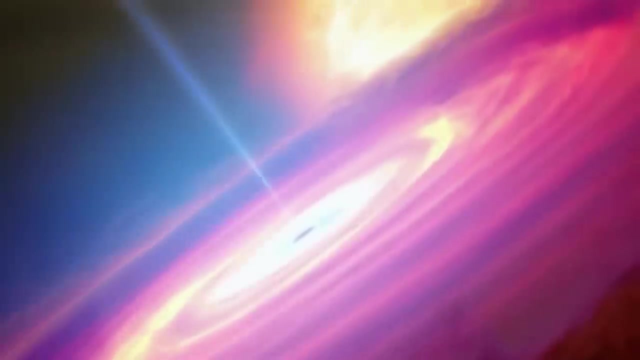 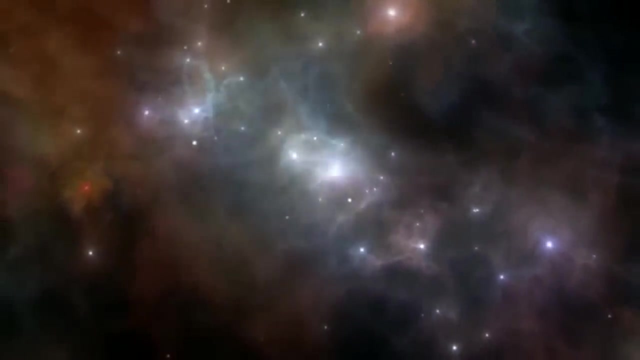 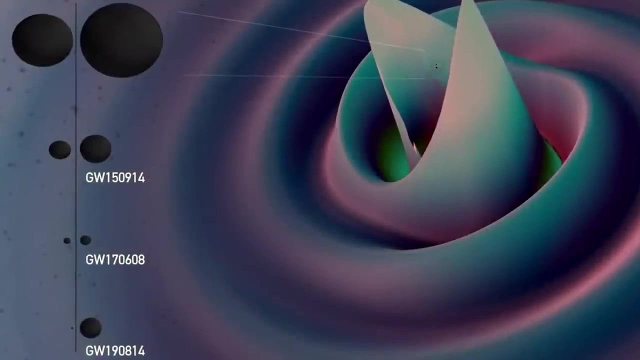 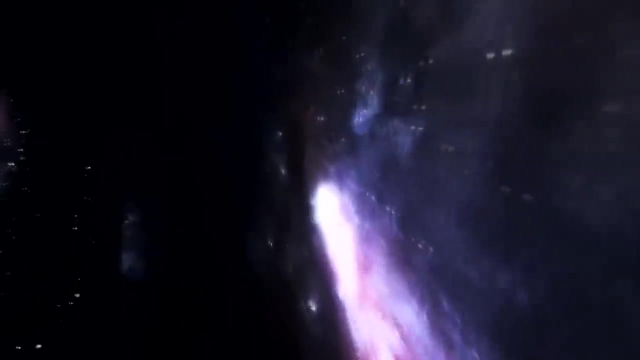 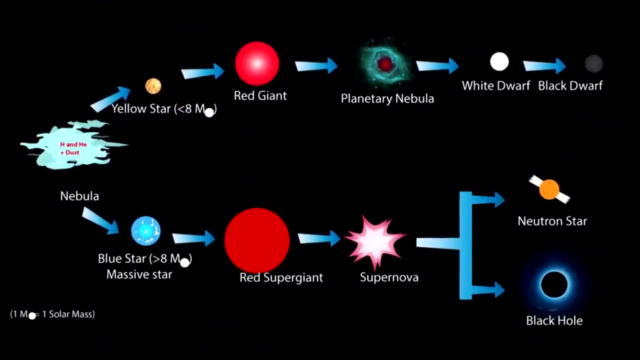 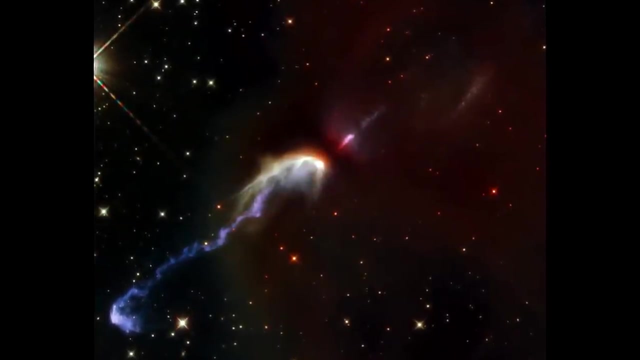 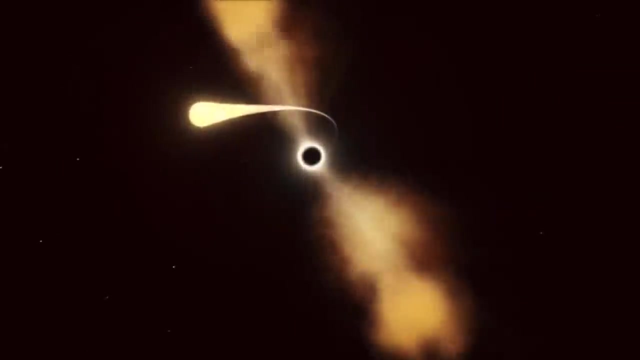 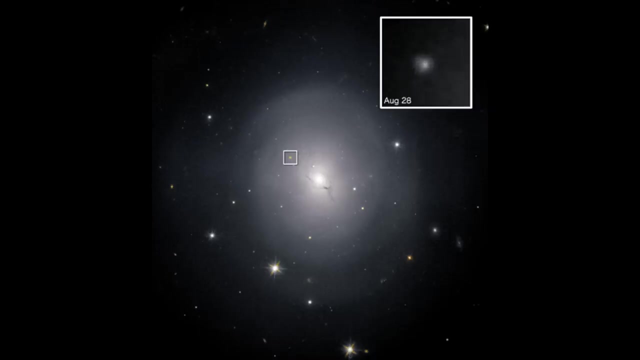 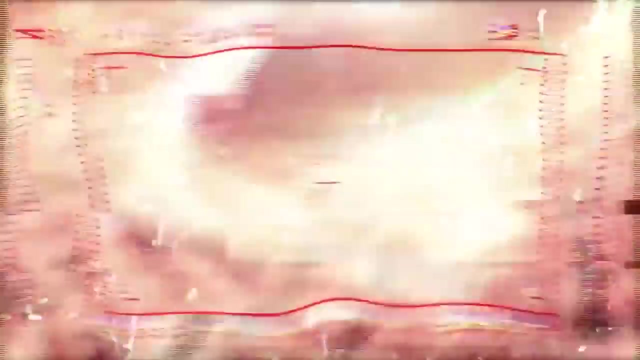 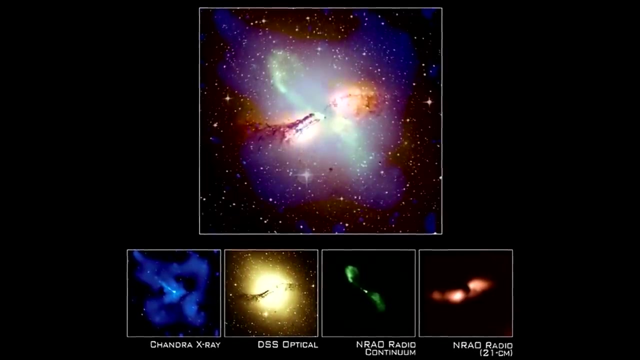 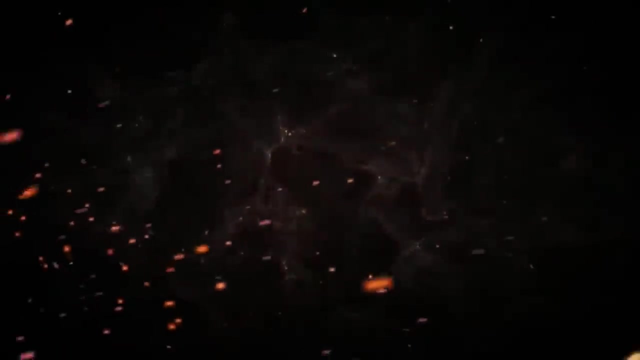 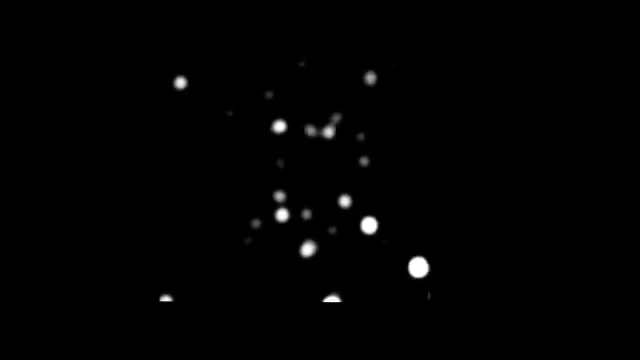 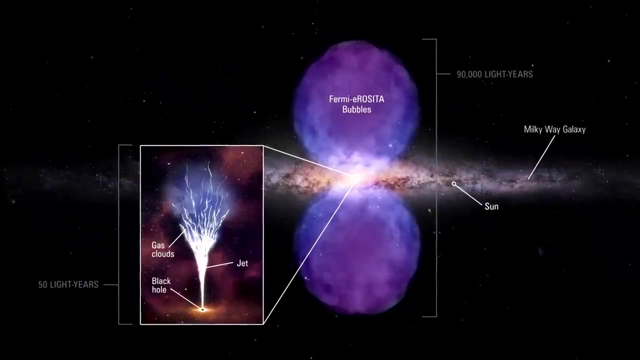 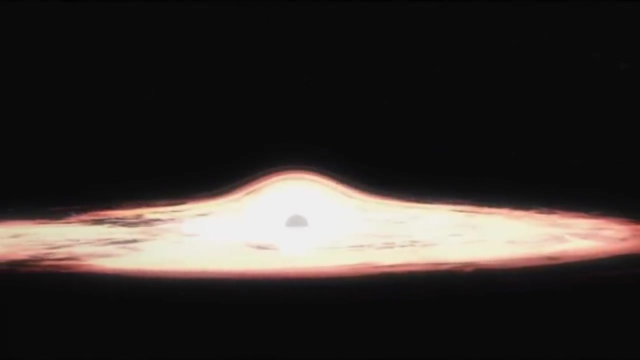 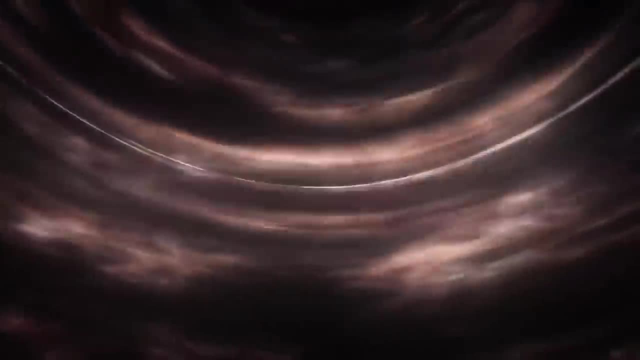 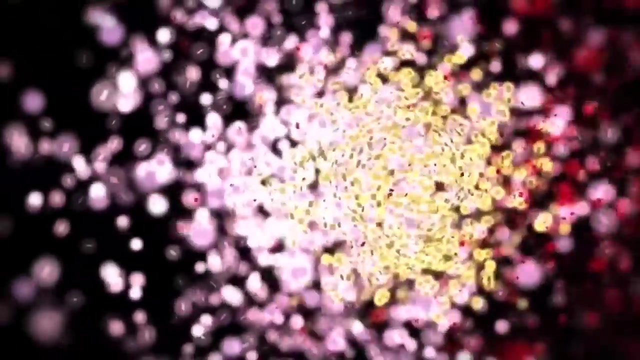 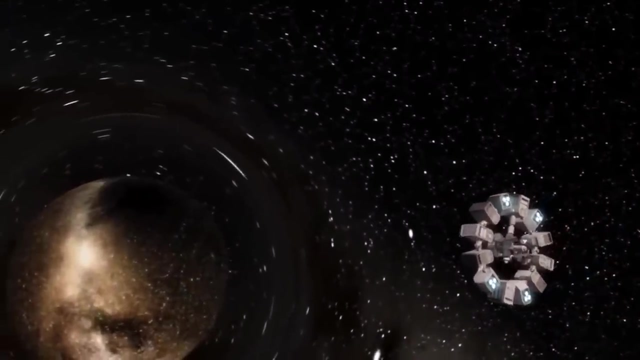 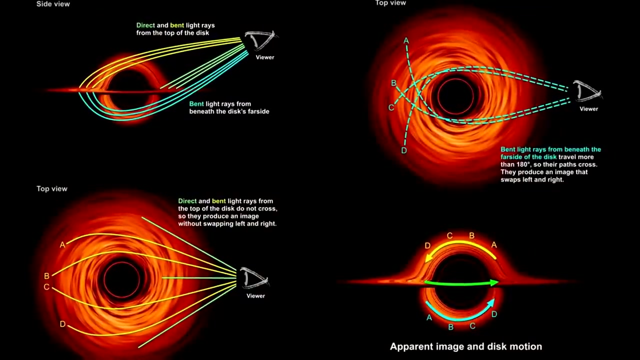 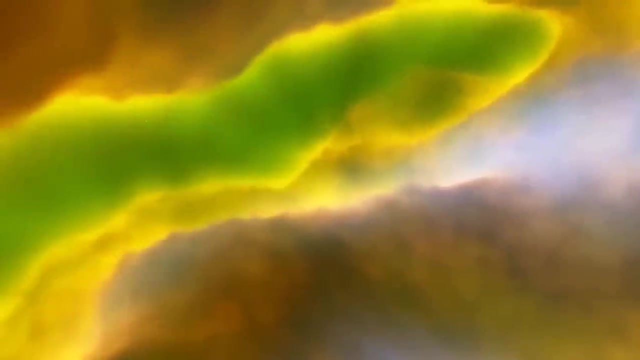 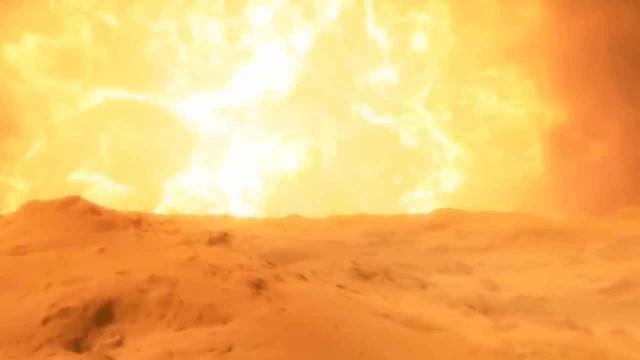 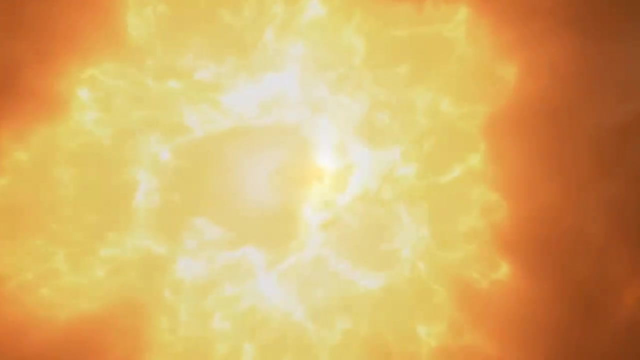 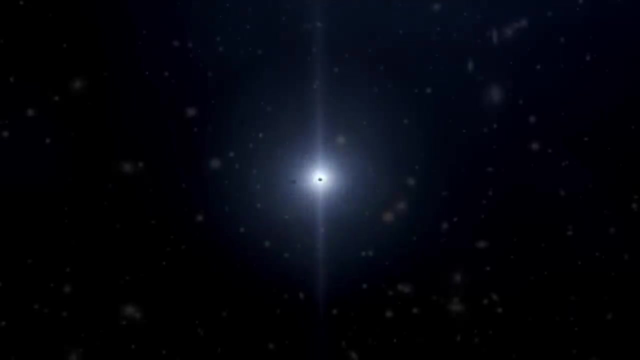 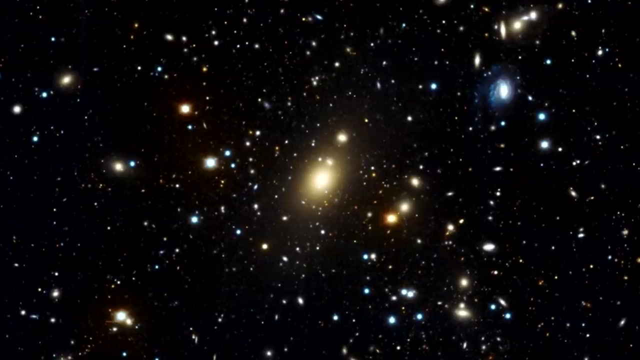 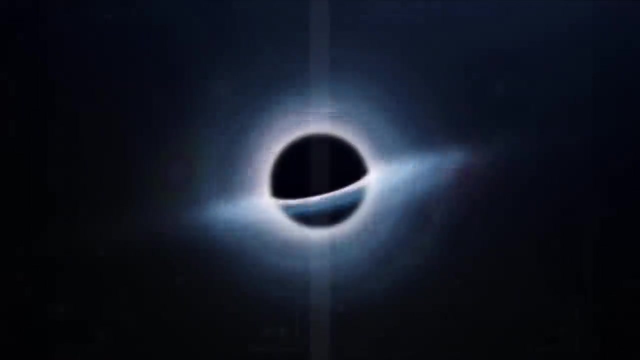 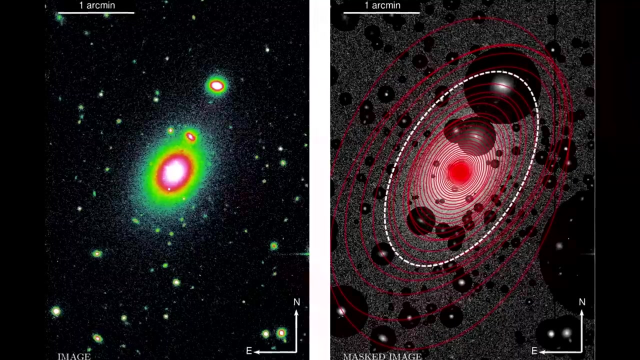 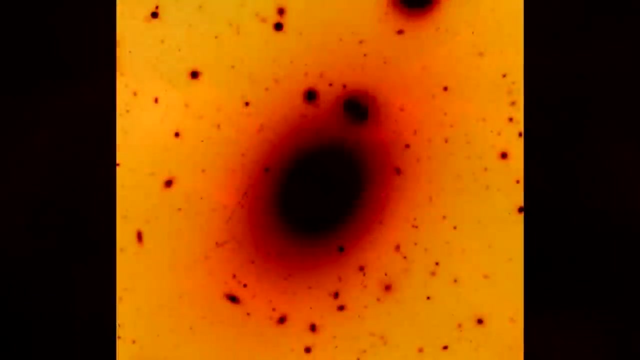 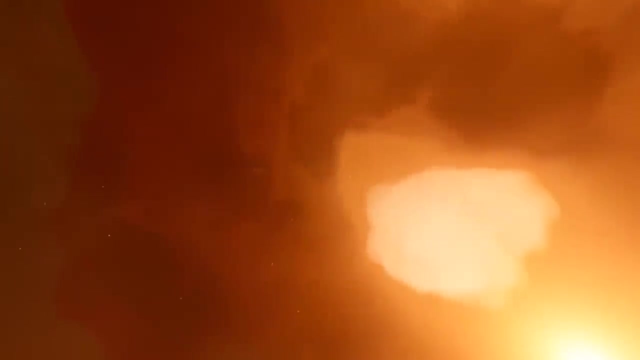 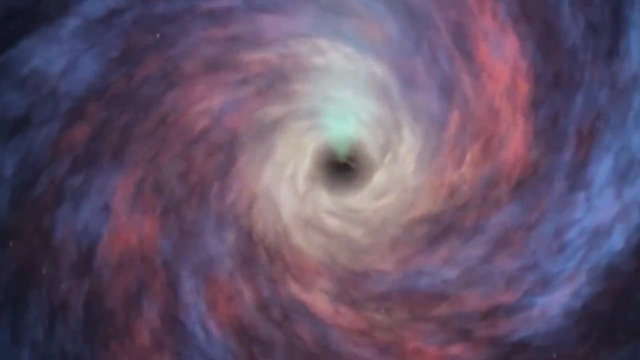 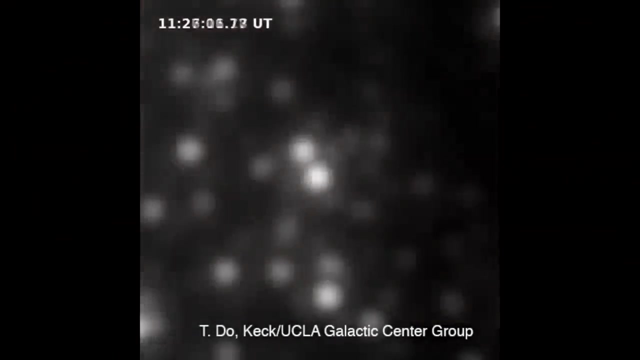 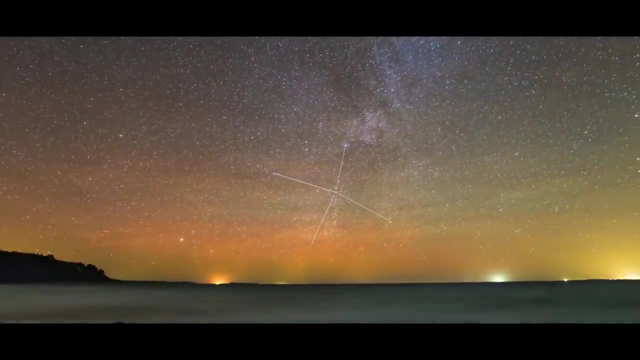 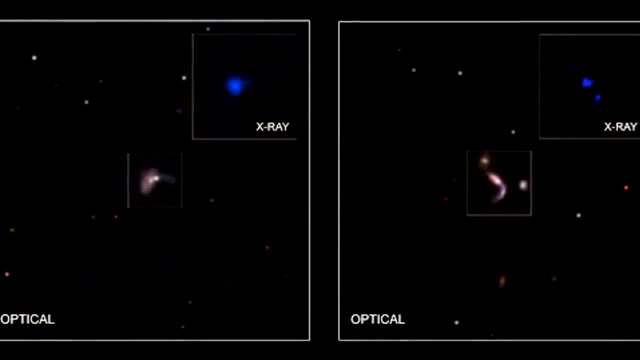 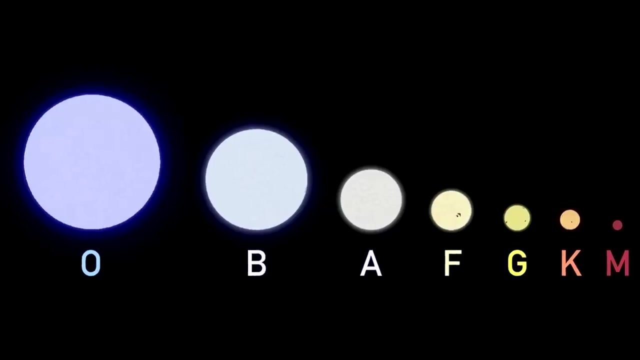 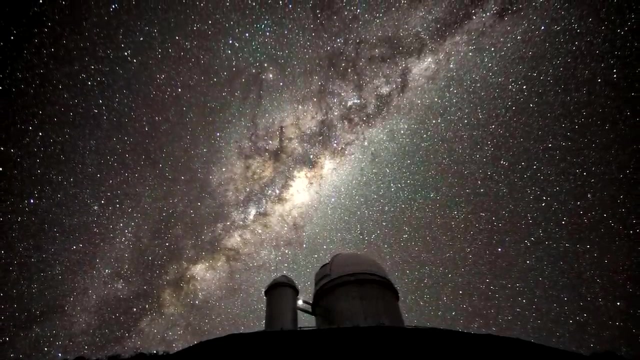 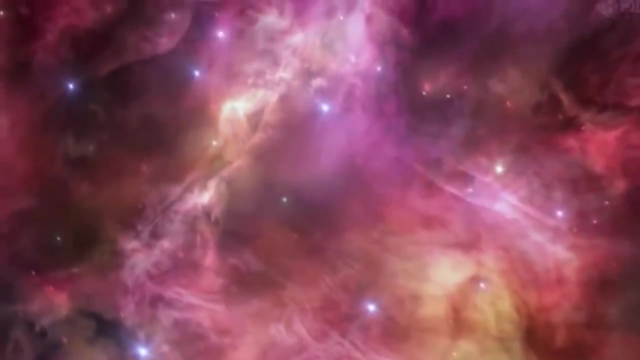 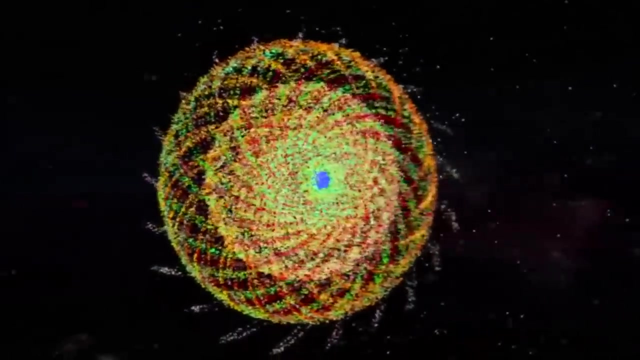 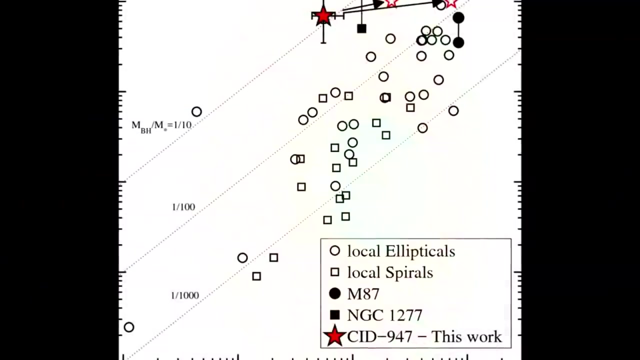 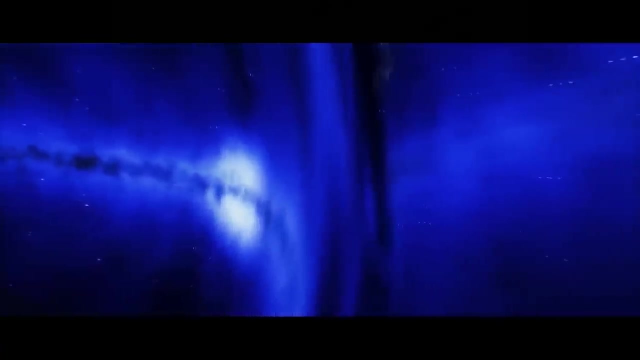 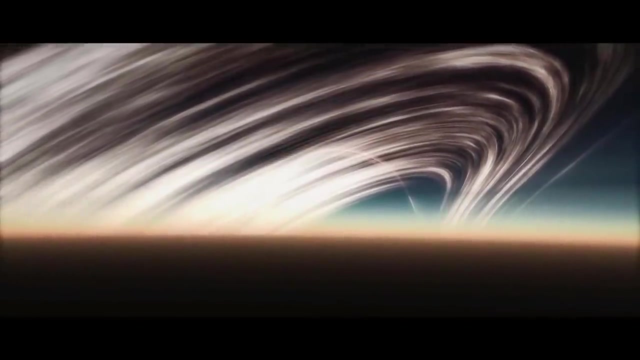 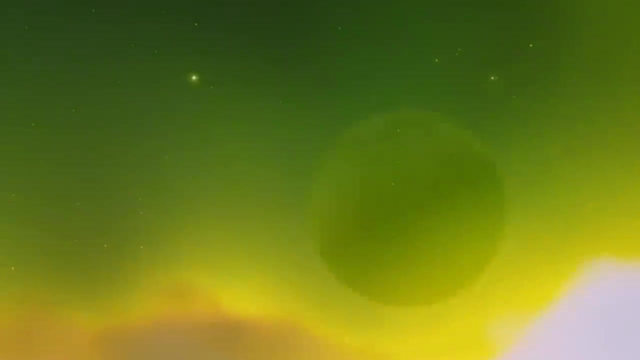 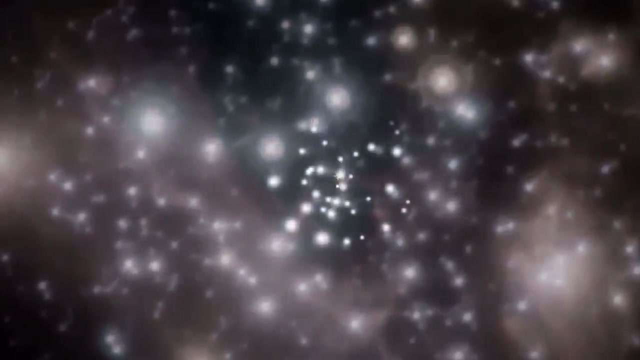 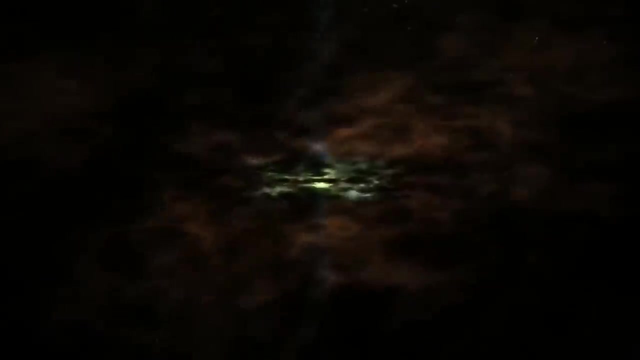 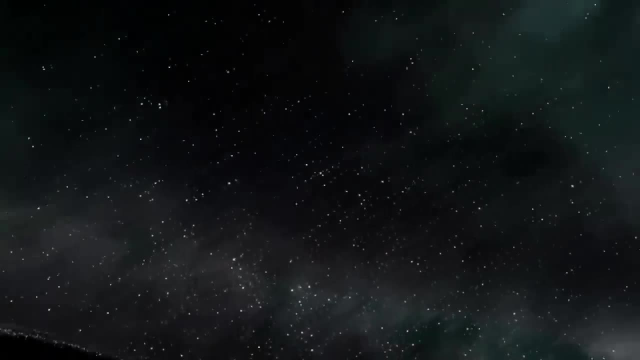 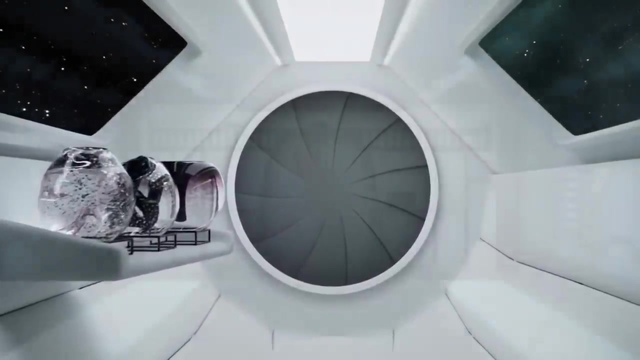 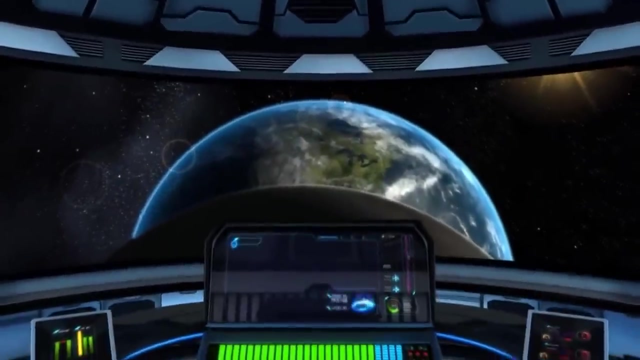 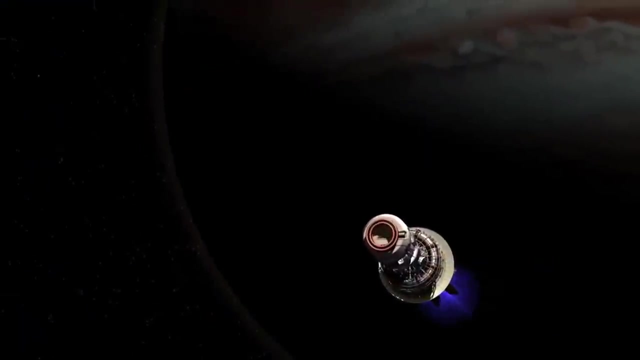 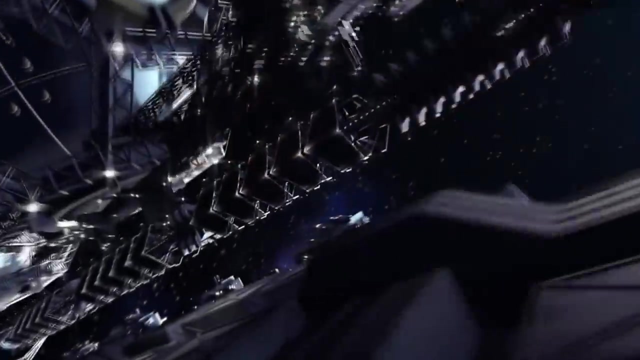 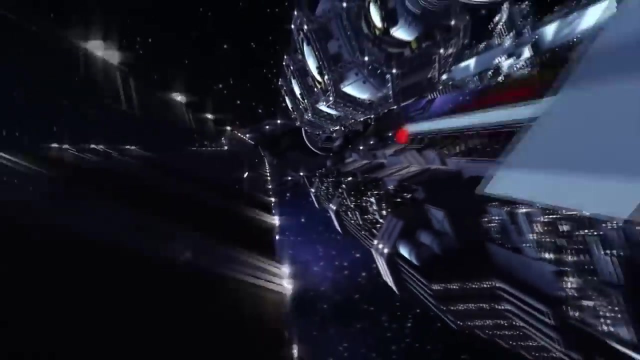 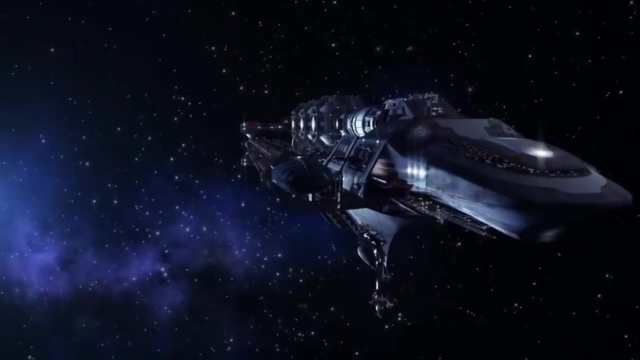 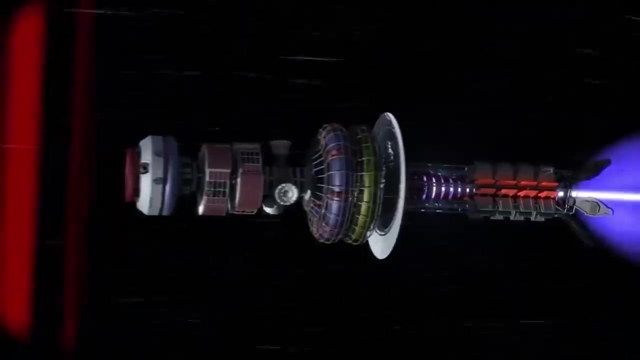 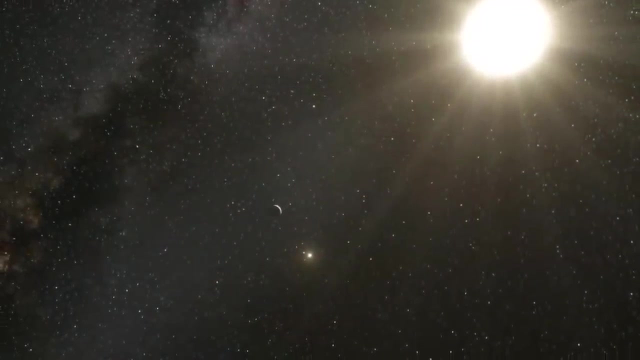 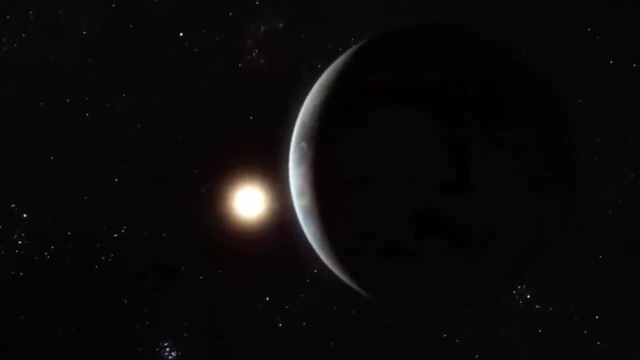 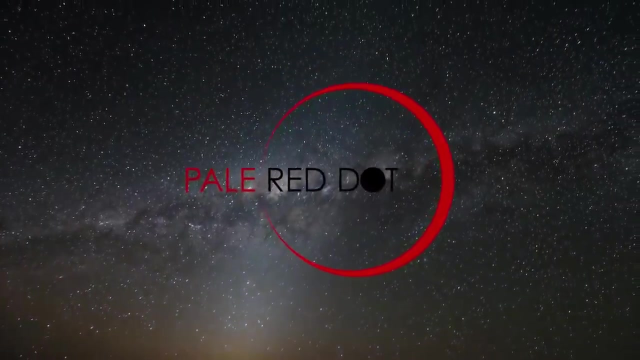 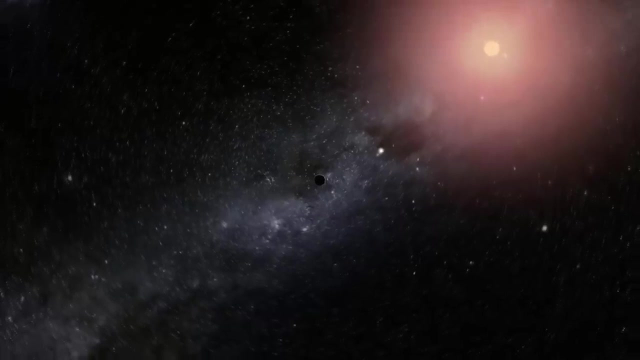 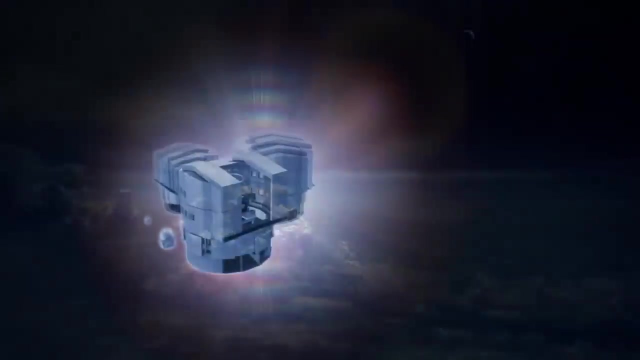 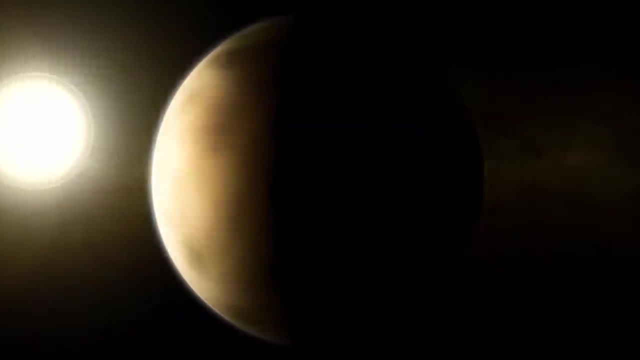 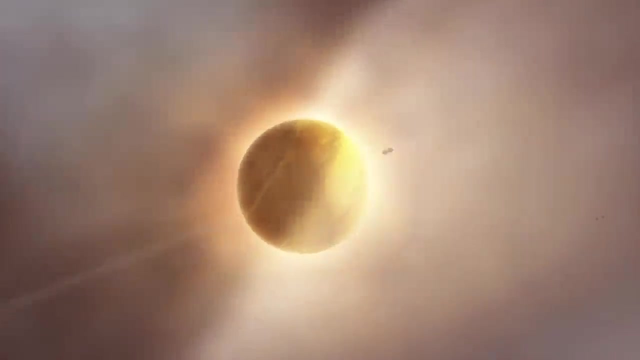 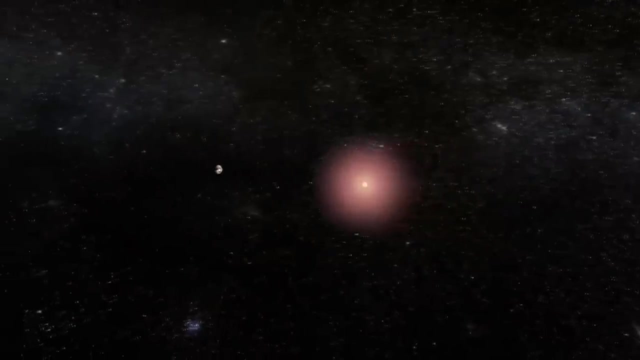 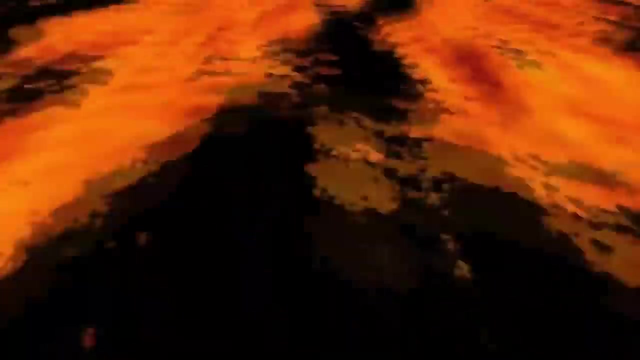 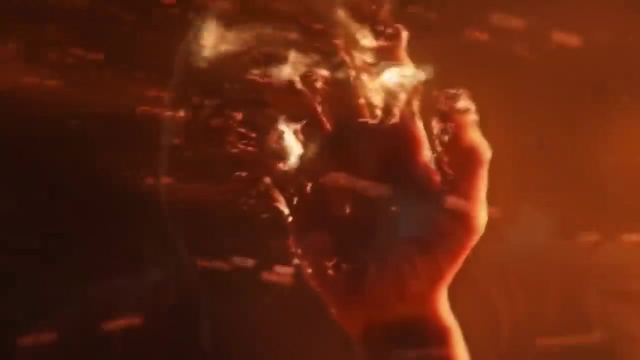 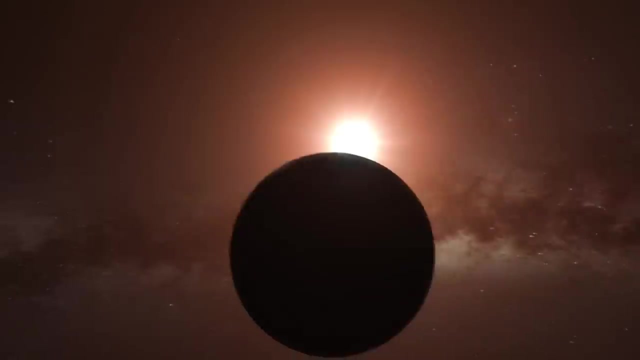 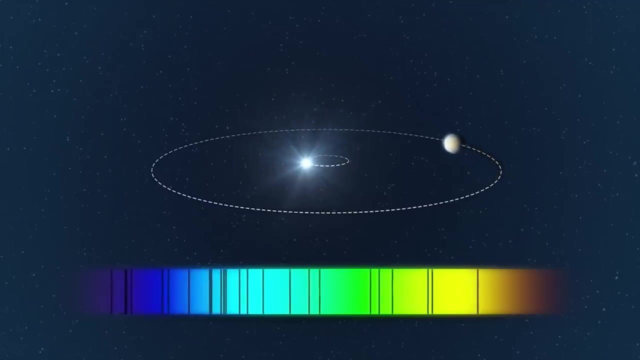 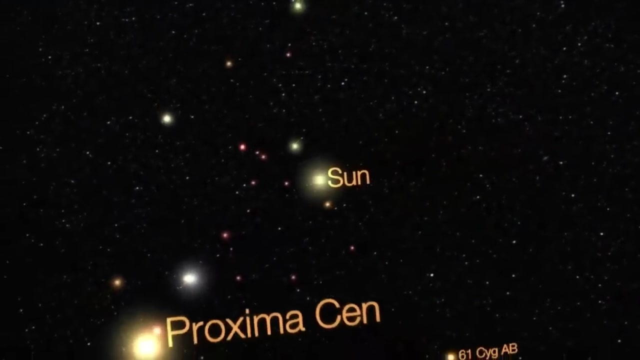 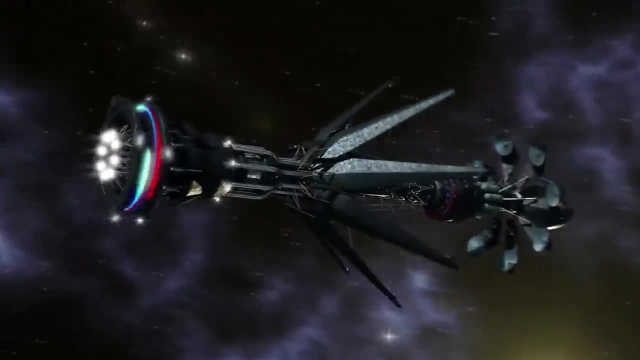 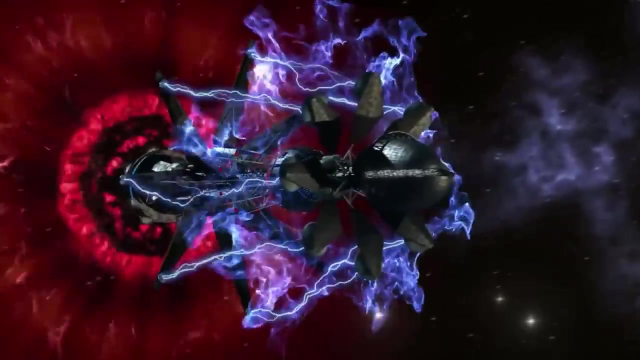 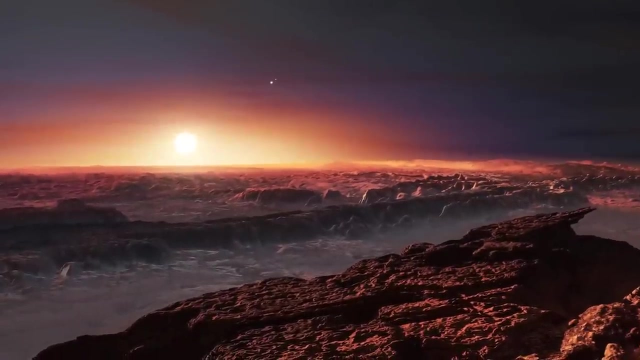 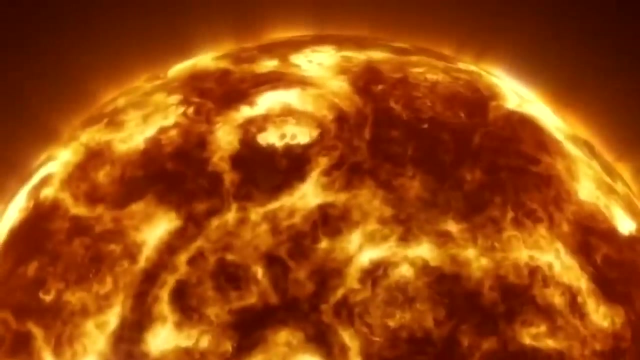 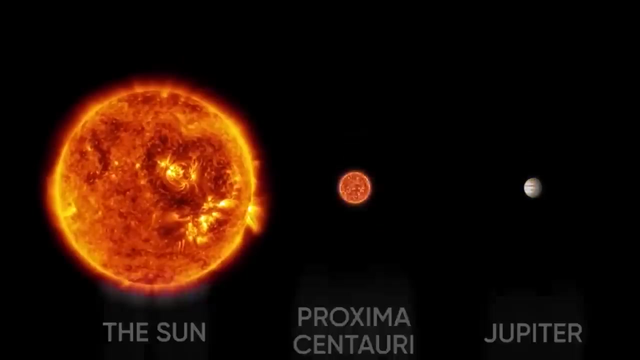 Transcription by ESO, translation by: — Transcription by ESO, translation by: — Transcription by: — Transcription by ESO, translation by: — Transcription by ESO, translation by: — Transcription by ESO, translation by: — The star system itself is called Alpha Centauri. 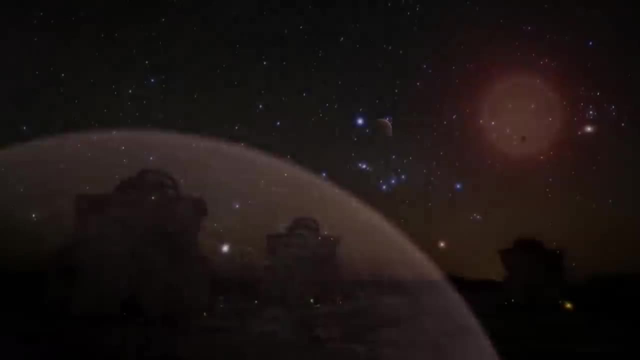 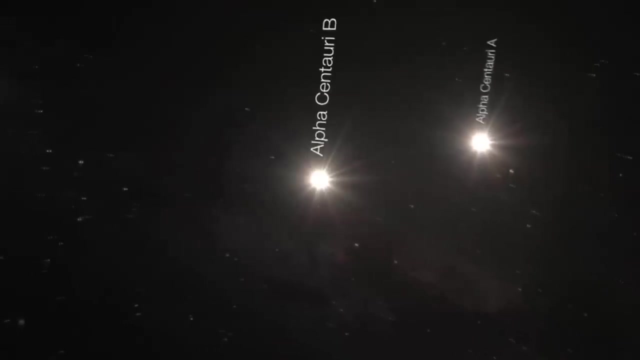 Two stars from Earth seem to us to be a single luminary: Alpha Centauri A and Alpha Centauri B. The planet that we liked for colonization revolves around the third star, Alpha Centauri C, or its other name, Proxima Centauri. 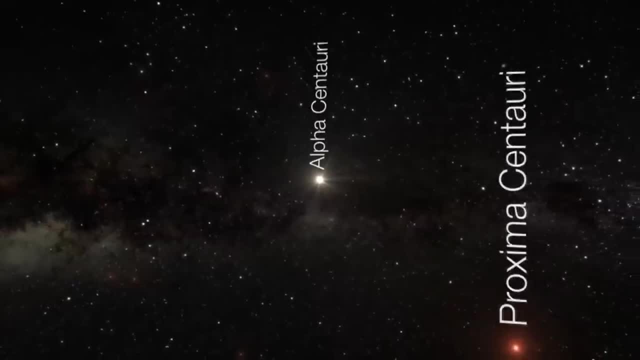 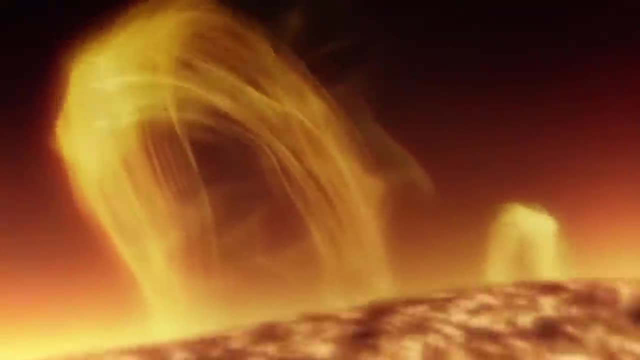 The red star is quite dim, so we can't see it with the naked eye, since red dwarfs emit a small amount of energy. Both stars rotate in an elliptical orbit around a common center of mass, and their orbital period is almost 80 Earth years. 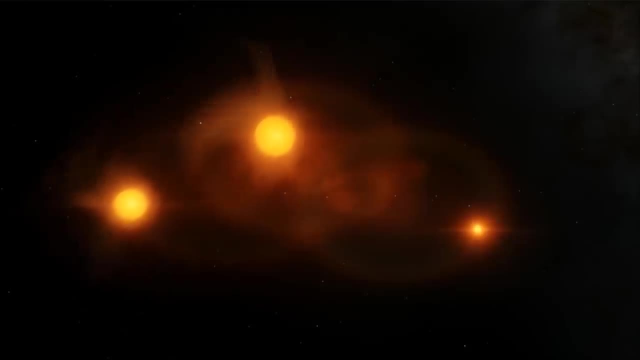 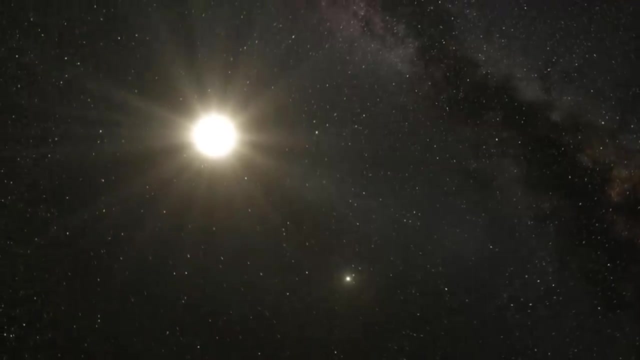 In order to get enough heat needed for life, the planet must be much closer to a star, like a dim red dwarf. In the case of Proxima Centauri B, everything is true: It is located at a distance of 7.5 million kilometers from its luminary. For comparison, there are as many as 150 million kilometers between the Sun and the Earth. It takes only 11 days for a complete revolution around the star Proxima B. Such a close proximity, on the one hand, is acceptable for the existence of water, but on the other hand, it can be. 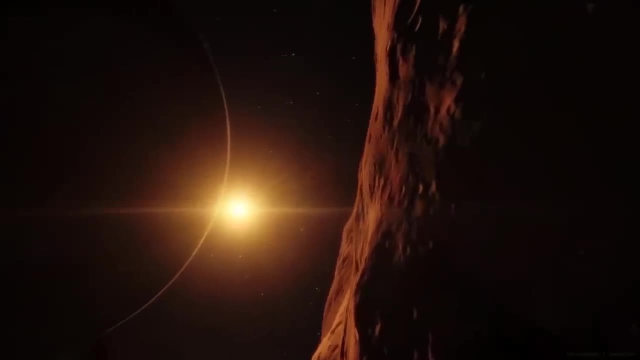 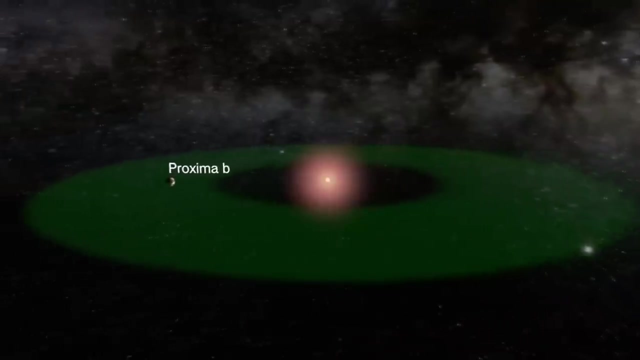 quite dangerous. If we talk about water, then it can exist only from the illuminated side, since, due to the tidal capture, the planet is turned to its luminary with only one side, so that local killer whales have to move their flippers around. 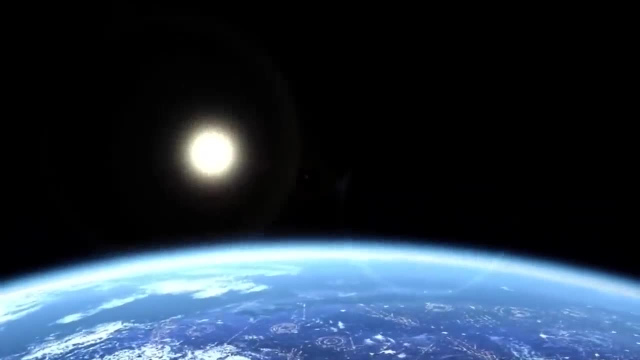 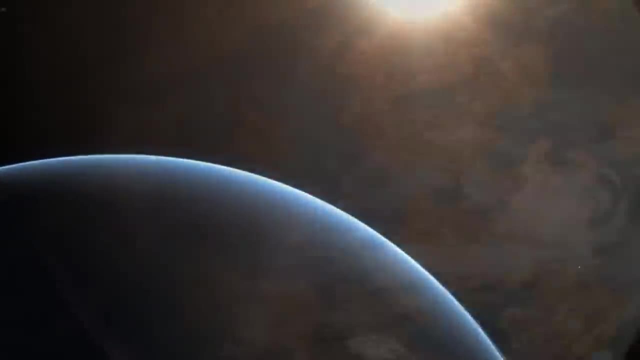 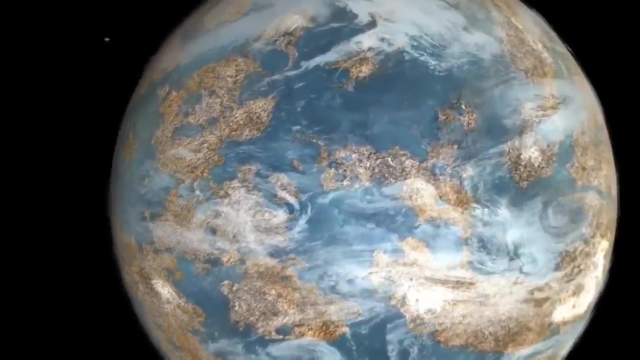 However, there is an opinion that there is still a rare change of day and night on Proxima B due to the elongated orbit, since, at its extreme points, the tidal influence of luminary weakens. It turns out that a day on this planet is almost two-thirds of its year, that is, by 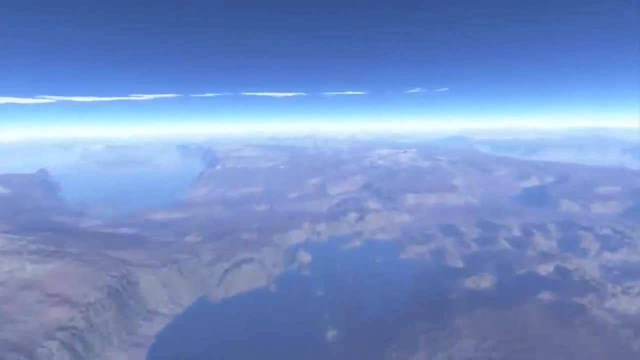 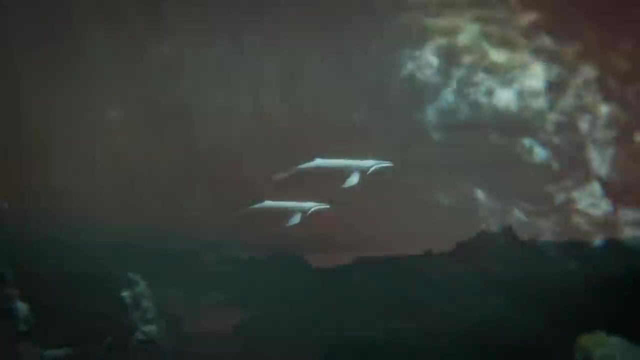 Earthly standards, they last about a week. And what about the possibility of the existence of any lifeforms on Proxima B? There is a hope for this. Theoretically, life is still possible on the planet, even with such powerful flashes of. 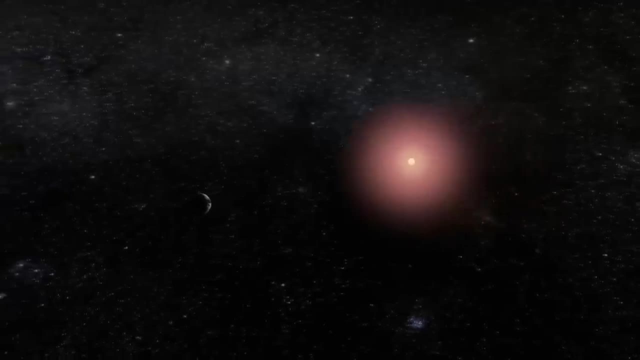 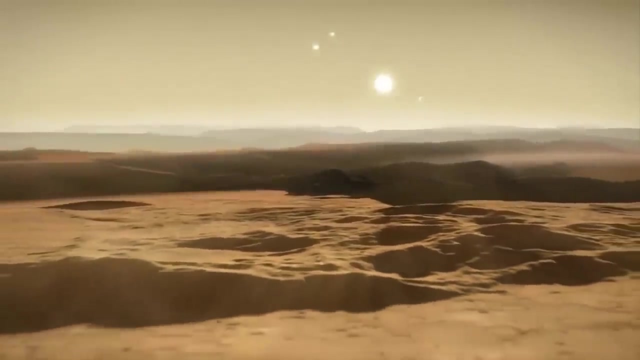 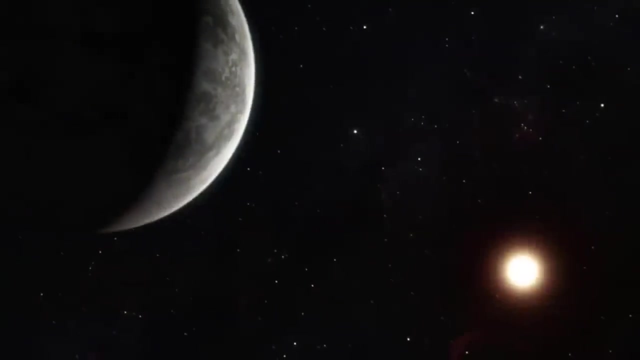 ultraviolet radiation. According to astrobiologists, some living creatures are able to hide from the deadly UV radiation using natural shelters. For example, they can exist underground or deep underwater. If living organisms on the planet have mastered this method of energy conversion, then it 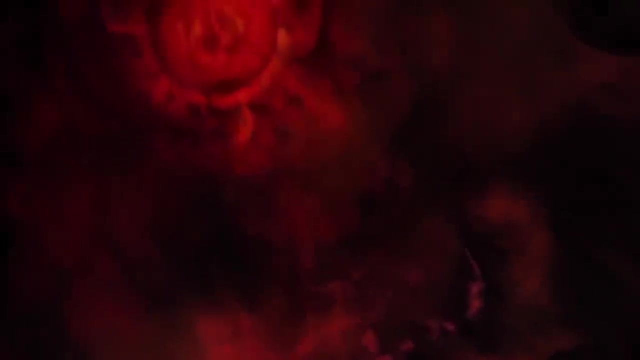 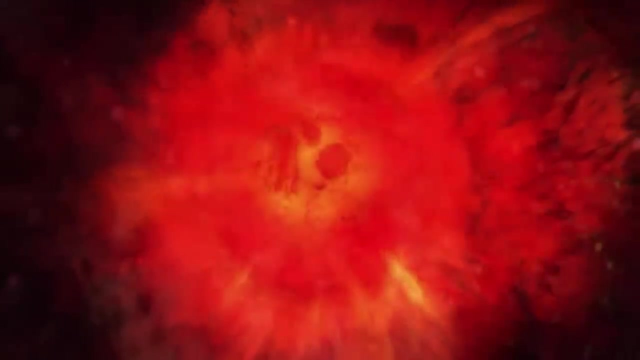 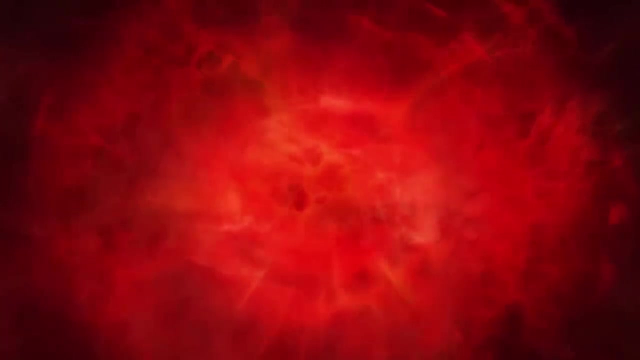 can glow very strongly at certain wavelengths, Perhaps even in the visible range. Such a powerful glow can be seen even from the ground. It is not surprising that the neighboring and so diverse system is of great interest Because of cosmic standards. it is just around the corner. 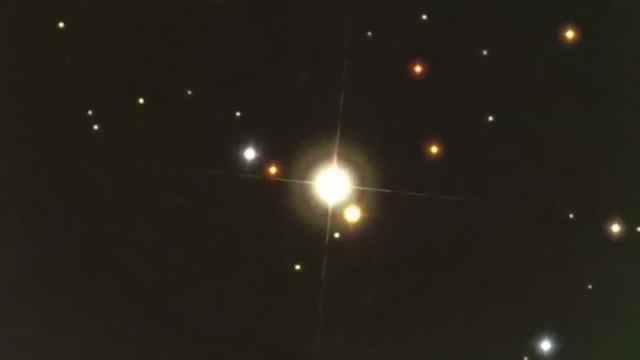 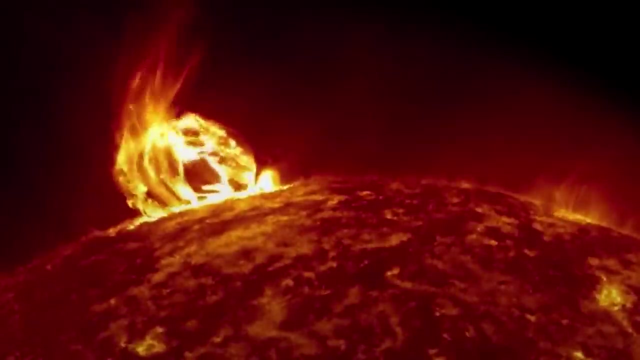 That is why, at the moment, there is quite a lot of interest in the incredible Breakthrough Starshot project. The goal of the project is really fantastic – to send a flotilla of interstellar ships to Proxima Centauri in the coming decades. 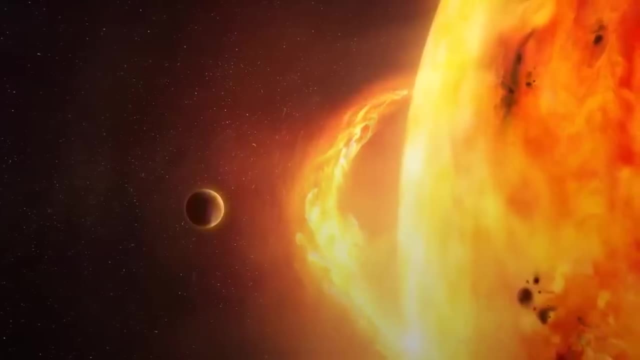 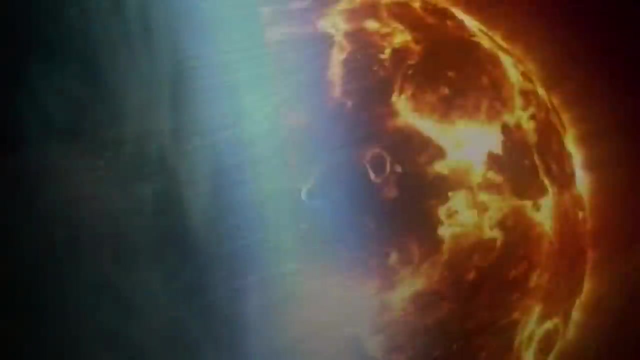 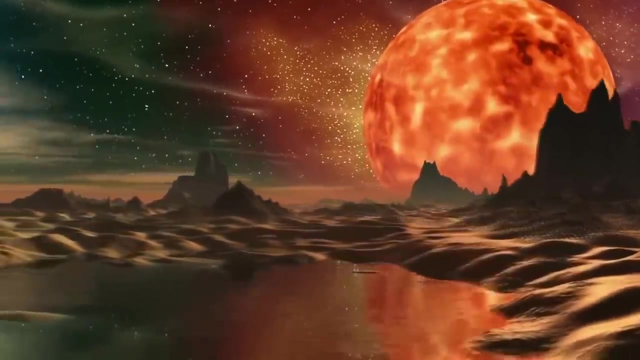 This is the goal. Miniature probes are even called, appropriately, Star Chips are not to be confused with a snack. It is assumed that the thousand or even tens of thousands of such vehicles, weighing no more than one gram, will be delivered to the near-Earth orbit and sent on a flight to Proxima. 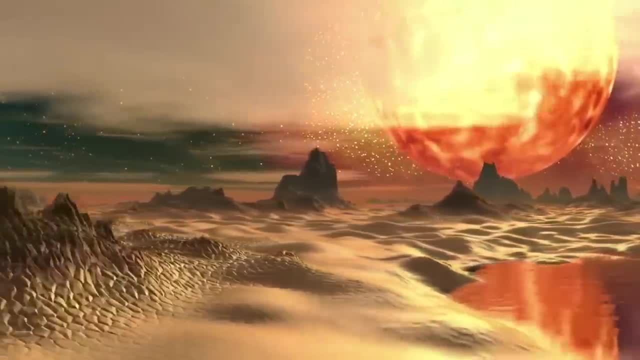 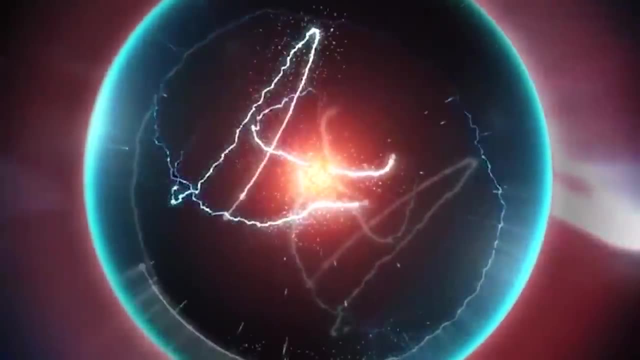 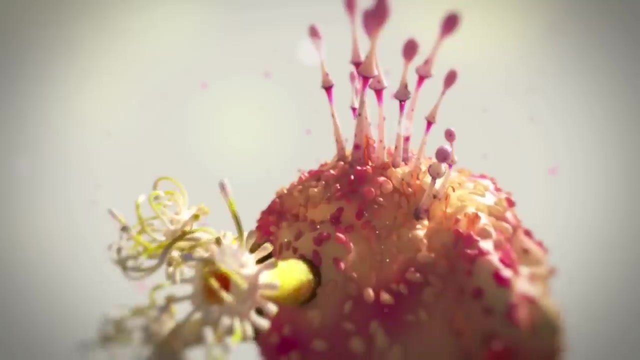 Centauri. The probes will deploy solar sails measuring four and four meters. The ultra-thin foil will reflect the incident radiation from the ground, accelerating the flight like a sail inflated by the wind. The push of the devices will be given by the beams of an array of lasers located on the 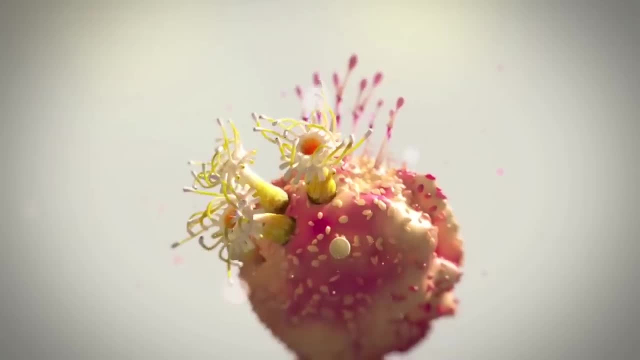 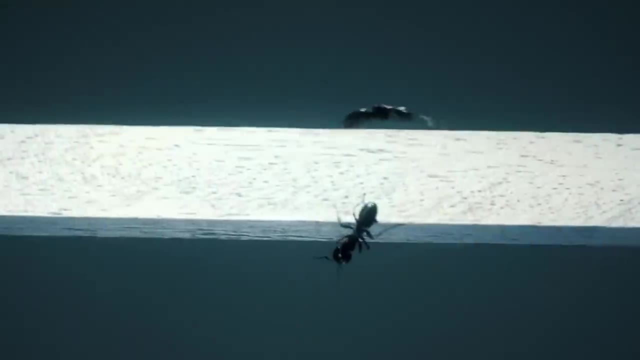 ground. This will be a ground-based phased array of laser meters measuring one on one kilometer, So the Star Chips will be able to gain up to 20% of the speed of light, and it will take them about 25 years to fly to Proxima Centauri, if everything goes according to. 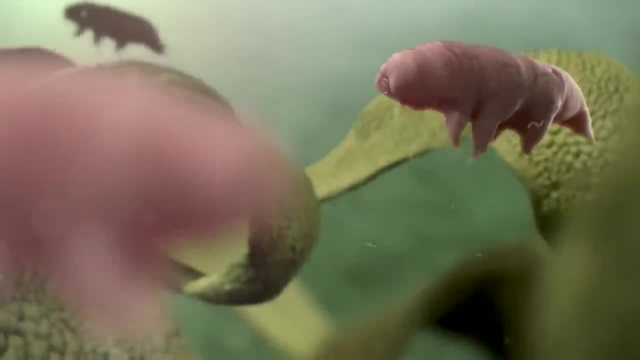 plan Upon arrival, the Alpha Centauri system. the probes will collect up to 20% of the light and it will take them about 25 years to fly to Proxima Centauri, if everything goes according to plan. These probes will also collect the necessary information, photograph the surroundings of 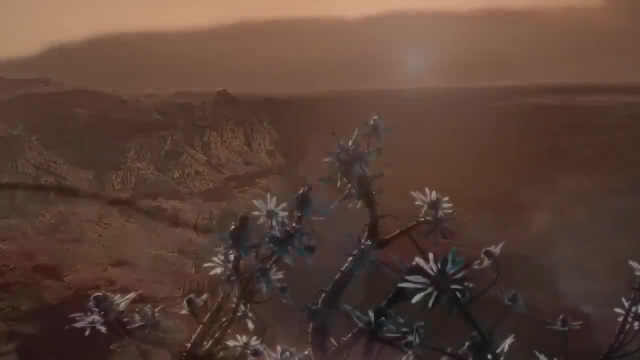 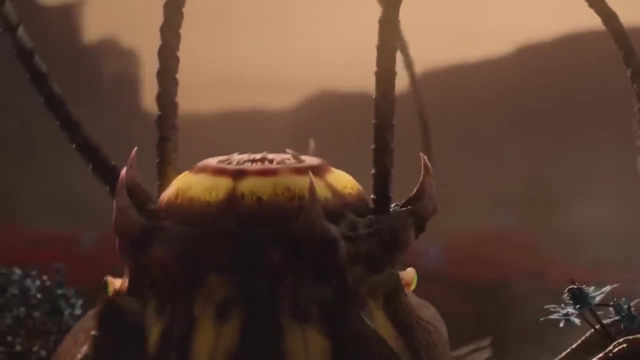 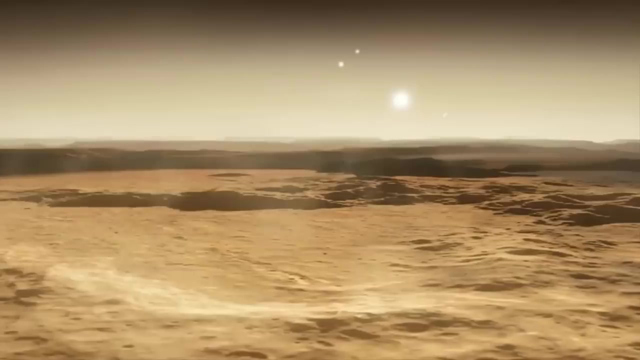 the system and the planet, and in five years this data will need to be accepted on Earth. In conclusion, it is worth noting that climate modeling of Proxima Centauri b gives completely different results depending on a variety of parameters: The speed of rotation of the planet around the axis or its absence, the presence of water. 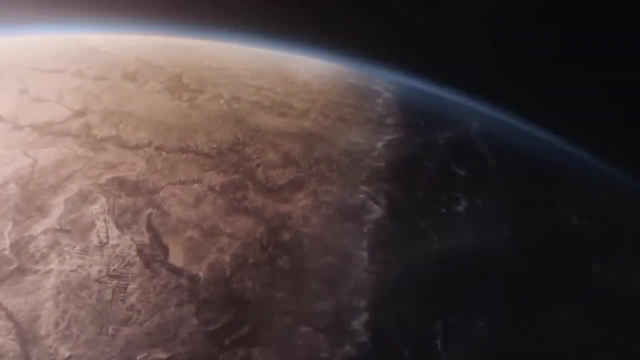 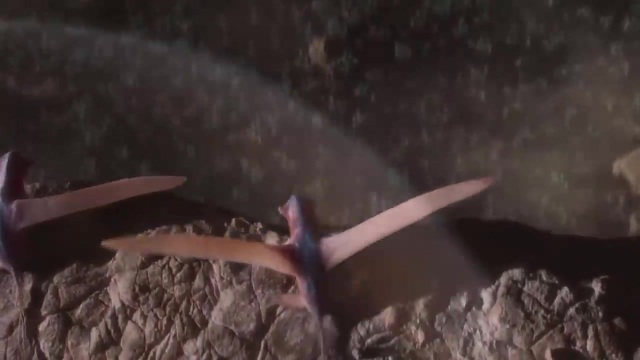 and the degree of its salinity, the location of continents, the density and composition, the atmosphere, etc. Let's hope that further study of it, as well as the flight of the interstellar flotilla of starships, will help us to finally verify the possibility of life on this planet. 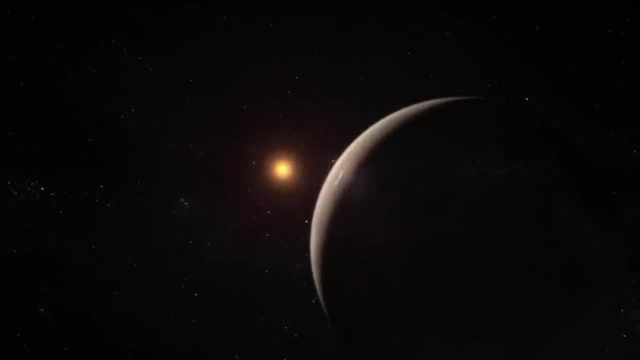 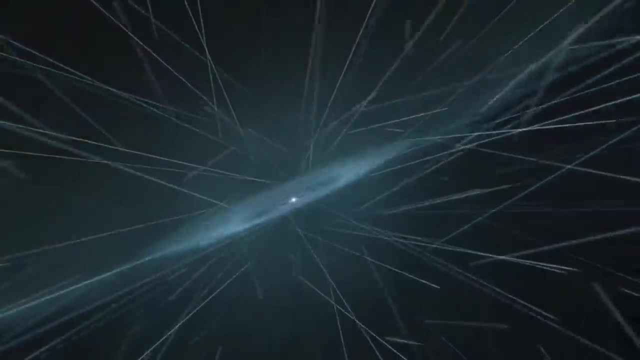 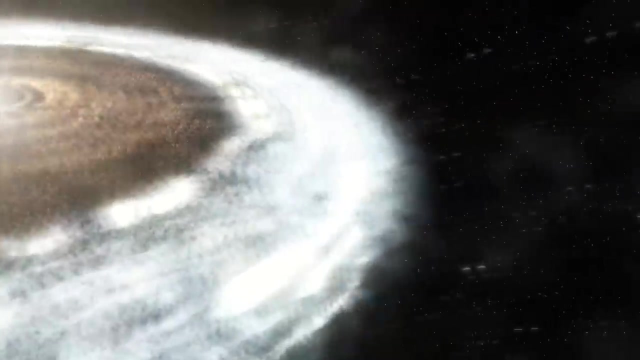 By tradition, we will keep our fists on our feet so that the project has further development. In the meantime, the potentially habitable planet closest to us remains mysterious and completely inaccessible. And what do you think? Does Proxima b have a chance? 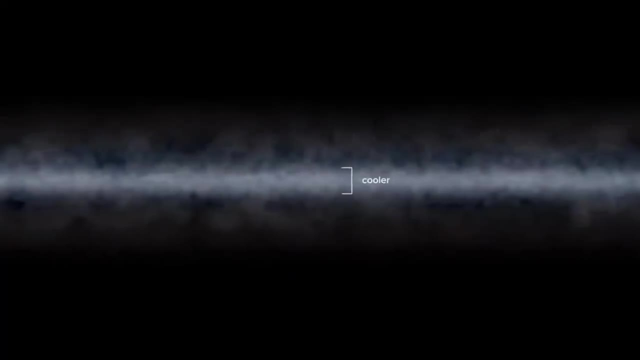 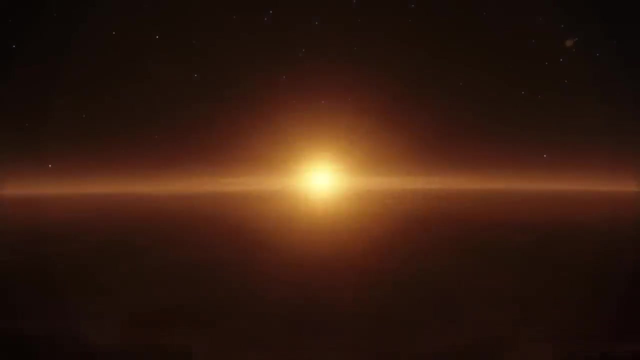 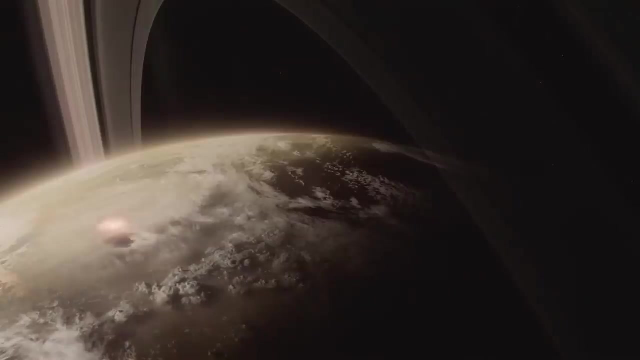 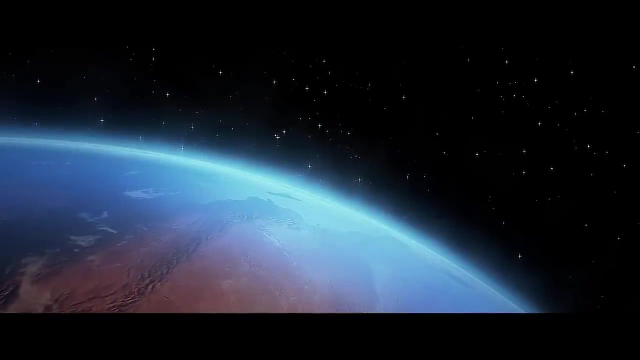 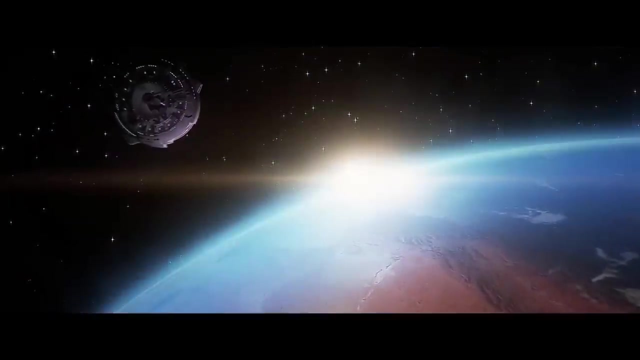 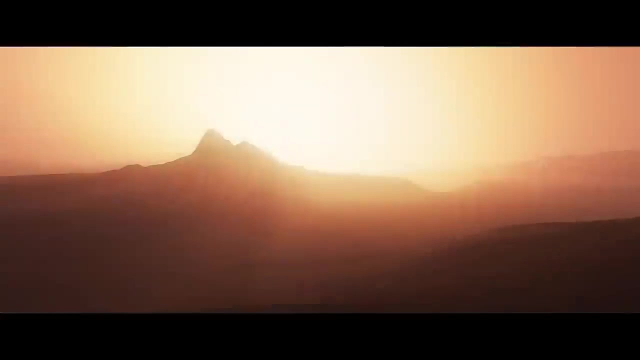 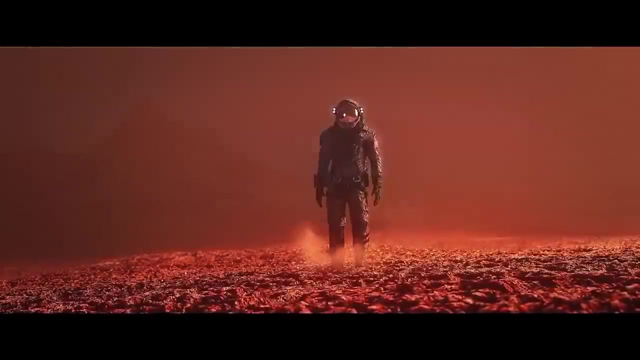 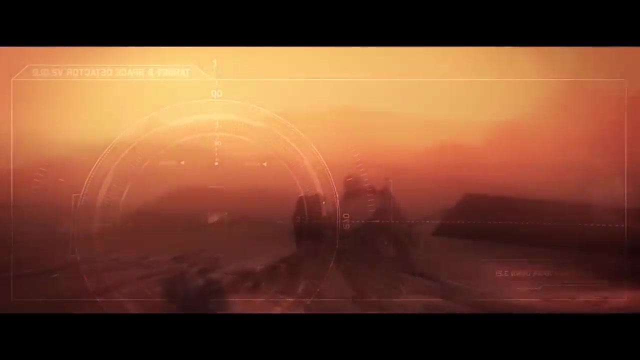 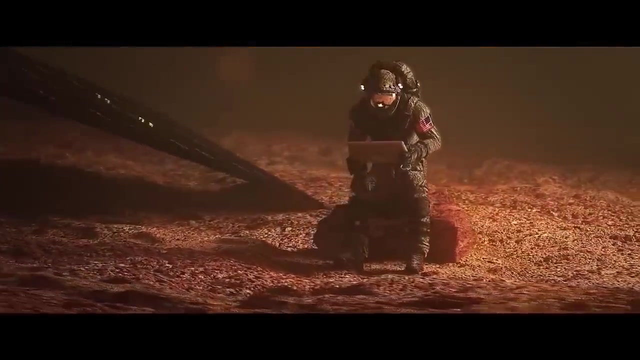 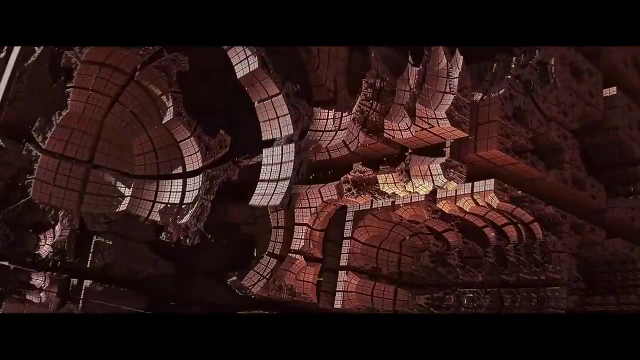 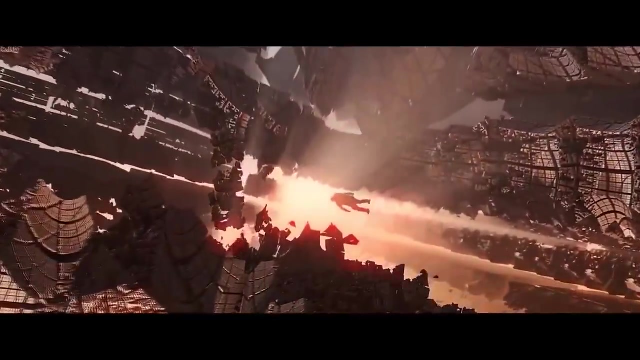 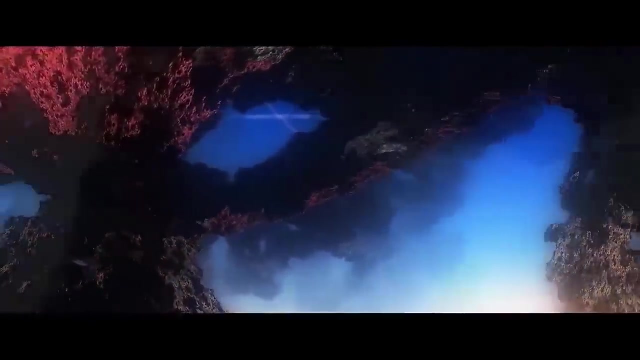 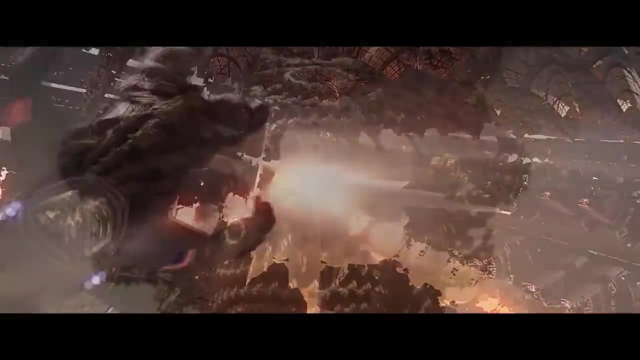 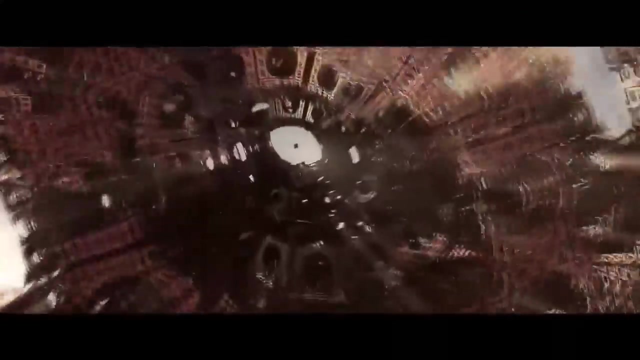 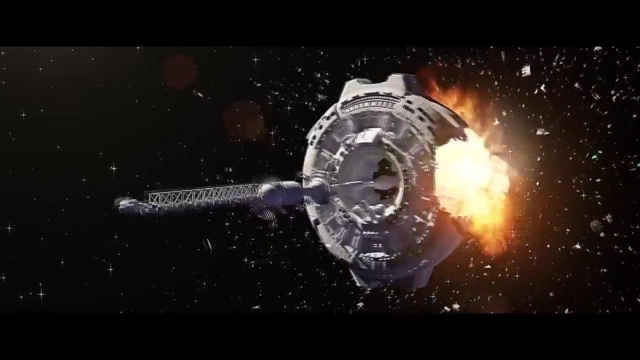 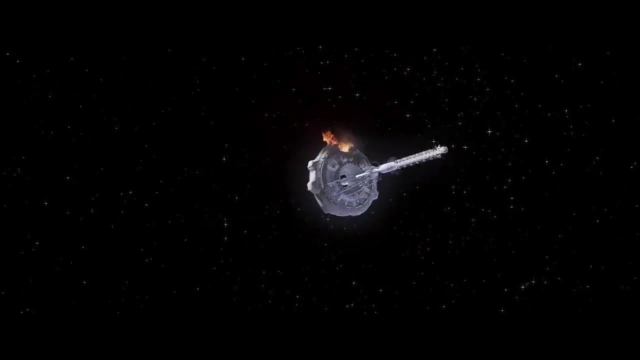 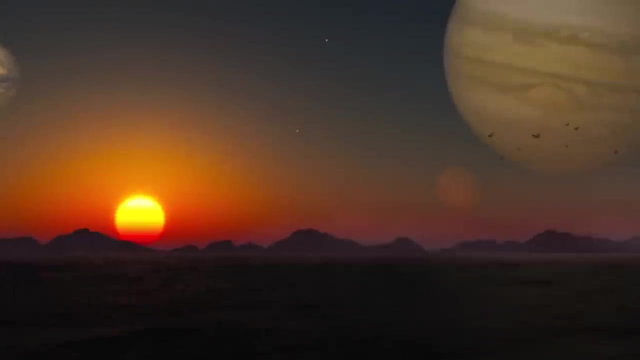 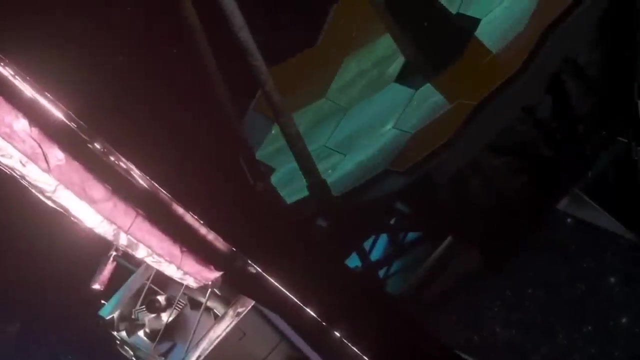 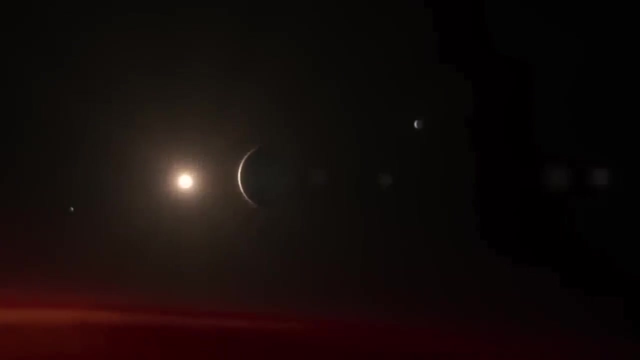 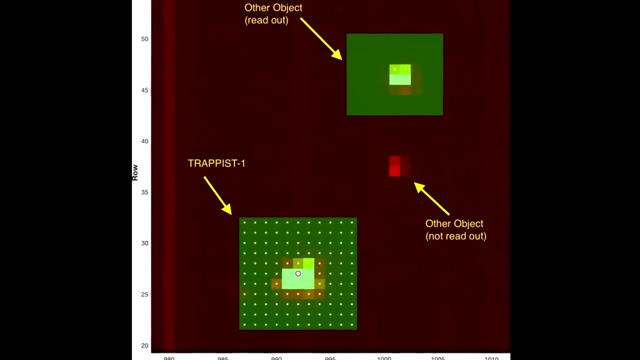 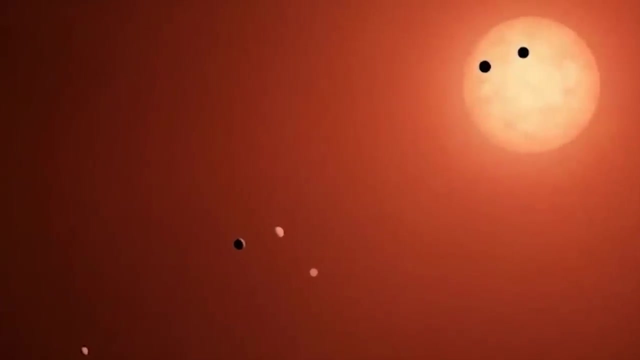 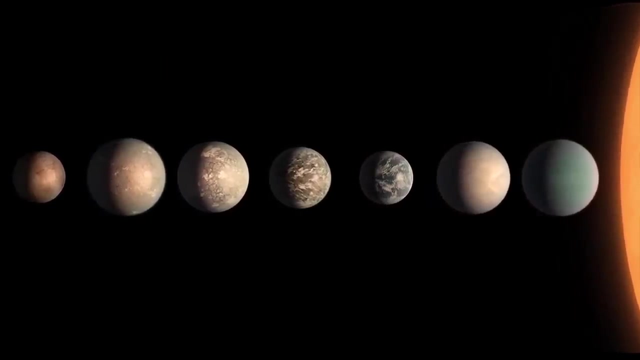 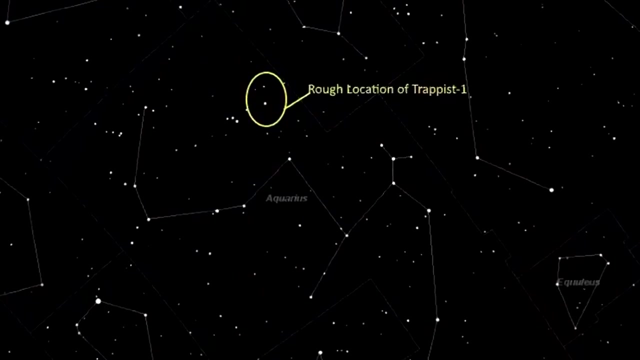 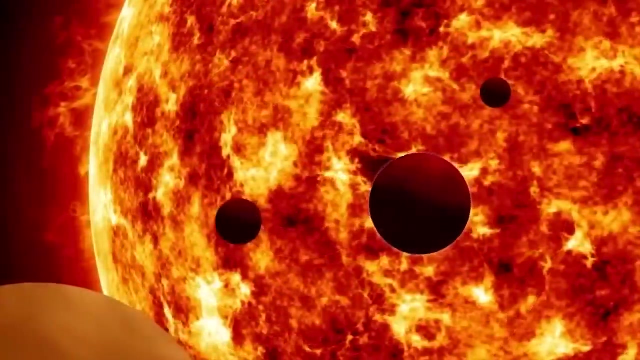 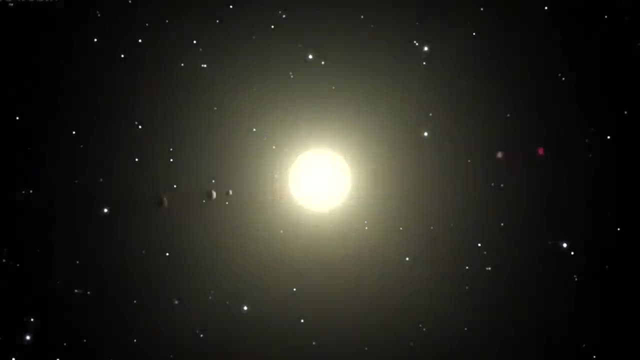 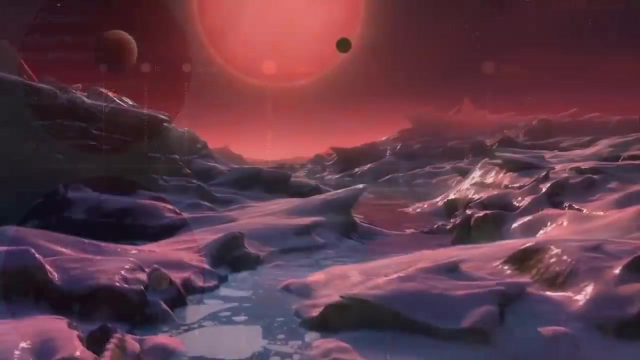 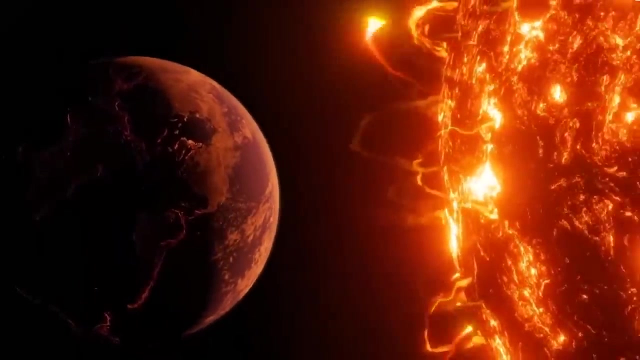 And this is important because Trappist One Worlds are the most optimal worlds available to us today. They provide the first opportunities for humanity to detect signs of biology beyond the solar system. Their initial discovery was made with a small telescope. A little later, exoplanets were discovered with the Trappist-Spitzer and full telescopes. 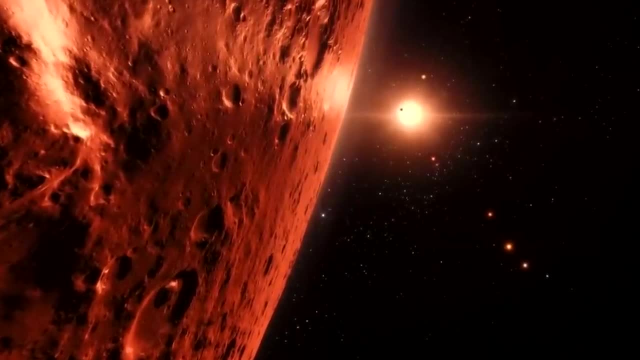 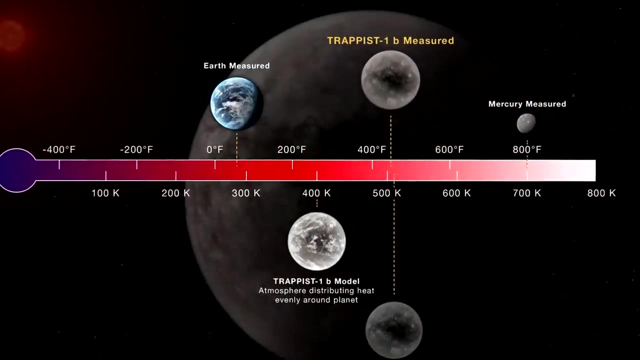 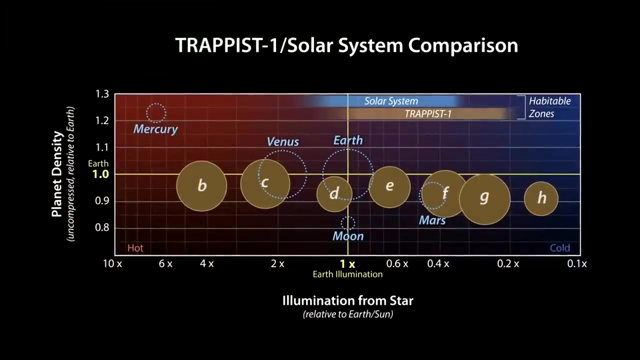 Thanks to the transit signals, it was possible to measure orbital periods and calculate their sizes. The exact transit times of exoplanets also makes it possible to measure their masses, which made it possible to know the density and therefore the properties of the bulk. 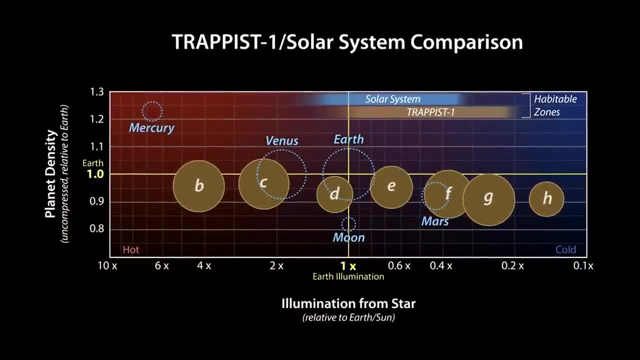 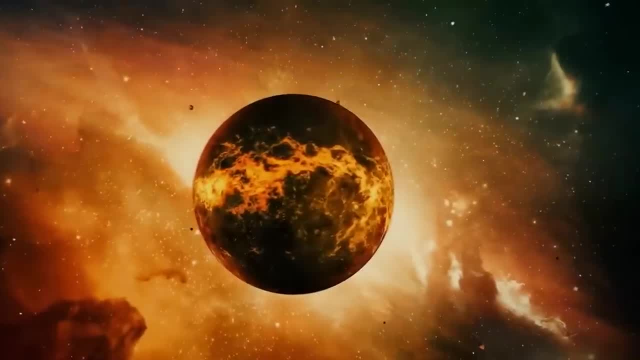 Astronomers have found that exoplanets conform to a rocky composition and that their sizes and masses are comparable to those of Earth and Venus, Relying on data from the distance of exoplanets to their star and the temperature of the star itself. 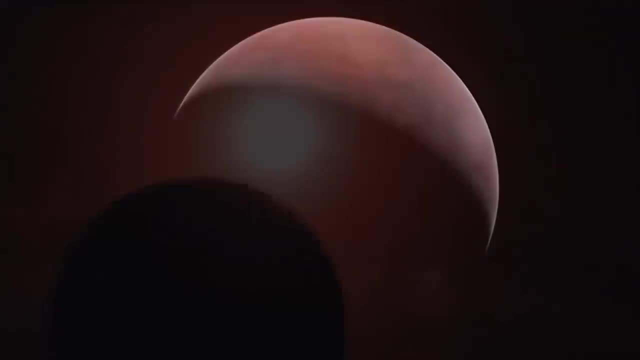 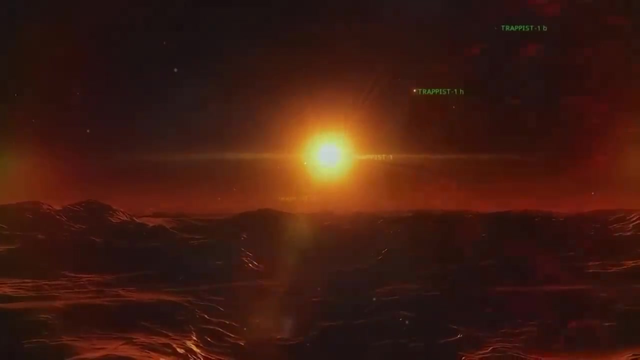 the researchers were able to confirm that the exoplanets are comparable to those of Earth and Venus, Conclude that some of them receive the same amount of light as many of the planets in the solar system, From Mercury to Mars. the James Webb Space Telescope has taken its first look. 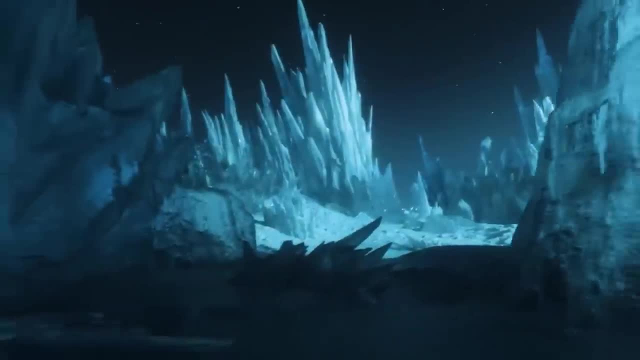 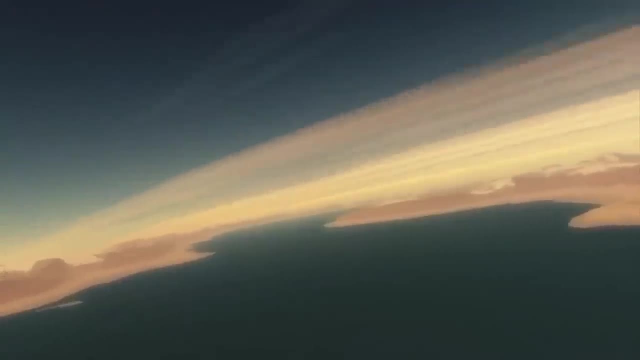 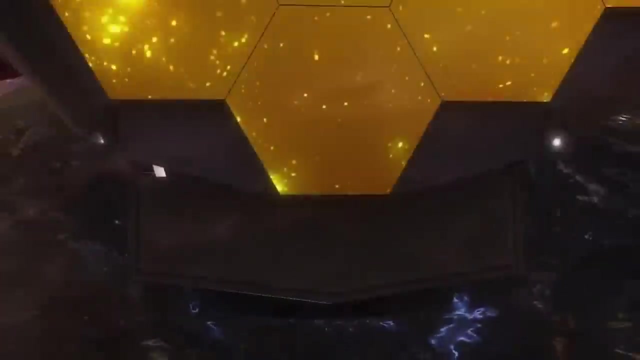 at a long-awaited target: the atmospheres of seven Earth-sized planets orbiting the star Trappist one just 39 light-years from Earth. All seven planets are in or near the habitable zone of their star and could have liquid water in one form or another. For astronomers, this is perhaps the best-known laboratory for studying. 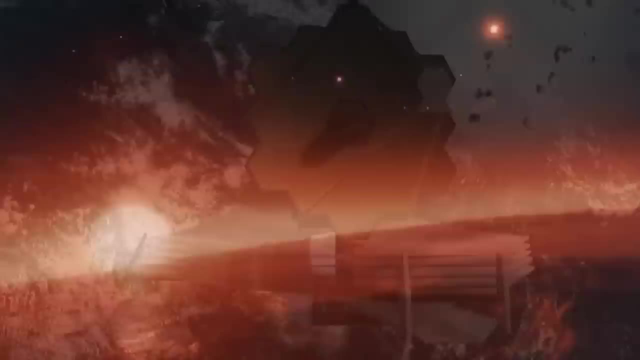 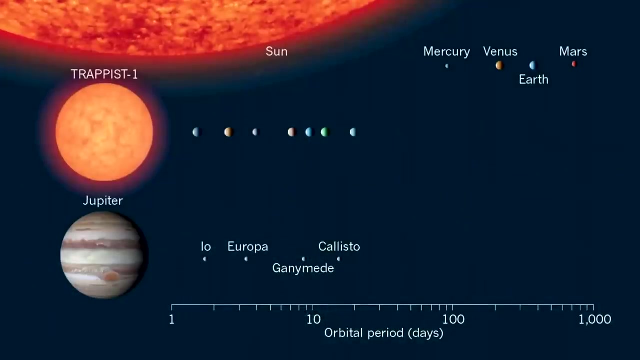 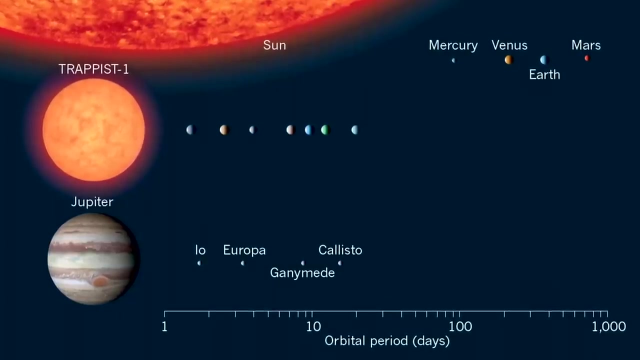 planets outside of the solar system for their suitability… for life. Finally, the James Webb telescope has set its eyes on these distant worlds. At the outset, it is worth noting that the telescope has confirmed that, of the seven known exoplanets in the Trappist – one system- three are in the habitable zone. 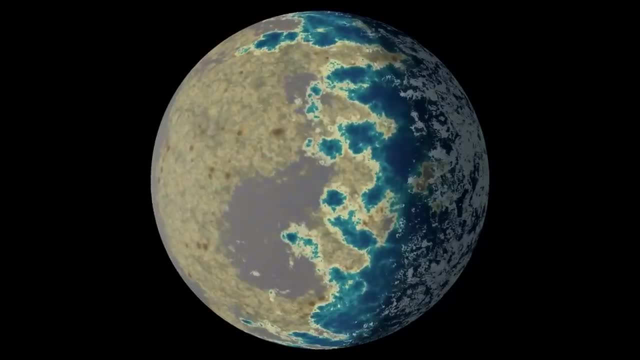 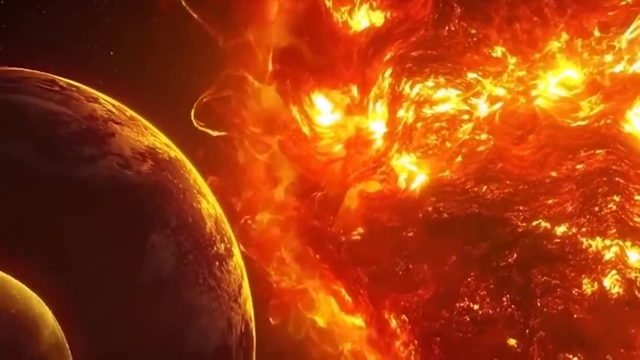 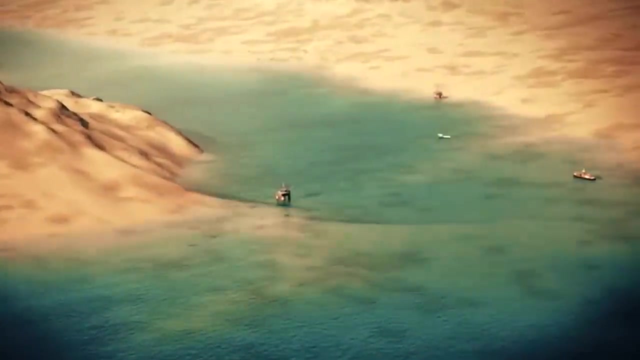 and F are the third, fourth and fifth exoplanets According to the measured density Trappist Oneb. the first, from the star, may either have a small nucleus or, more likely, contain a significant fraction of water or other volatiles in its composition. 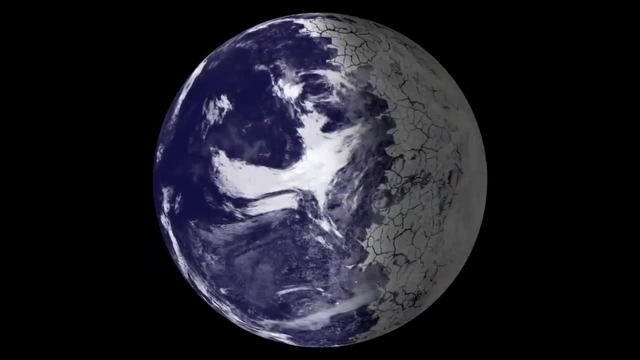 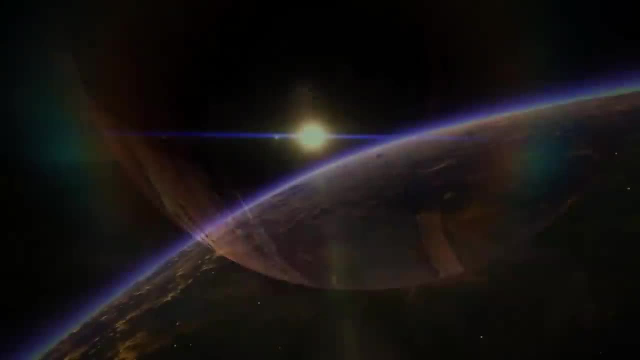 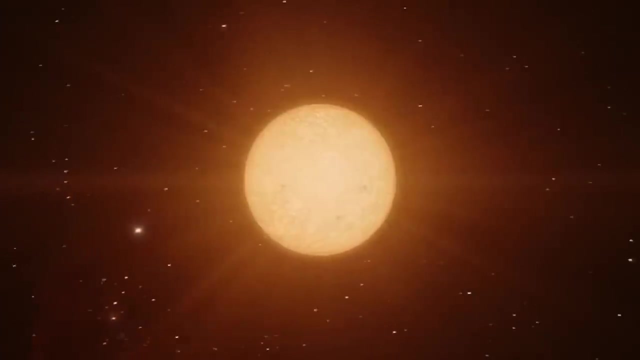 In view of the too-high surface temperatures of the first two exoplanets, the maintenance of water in liquid form there is highly unlikely. The fifth exoplanet, F, has a fairly low density and may be an ocean planet with space tangents in its interior. 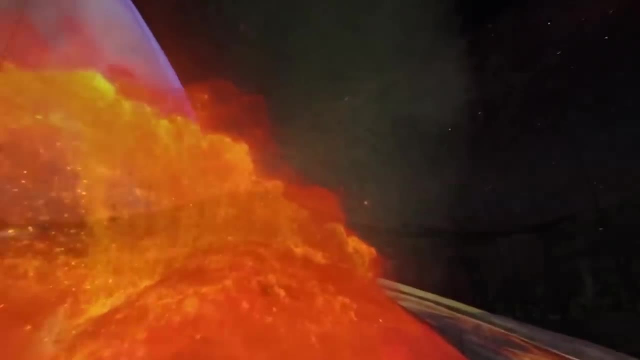 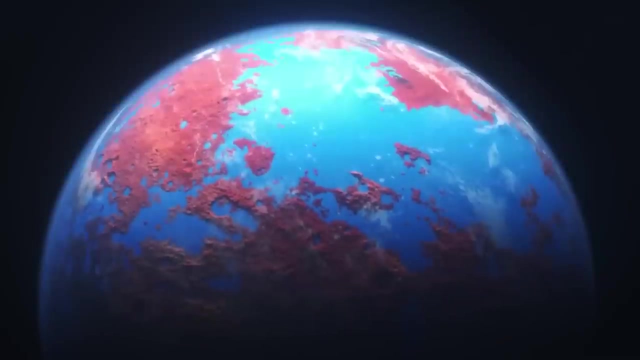 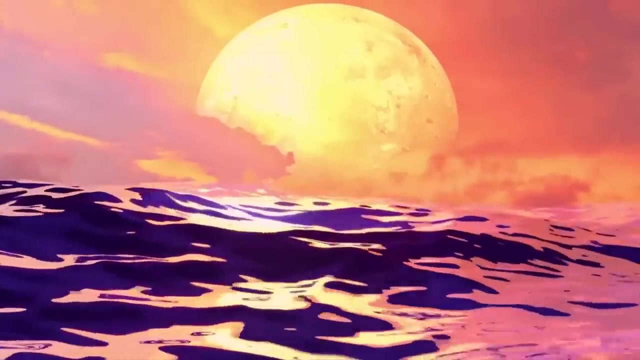 By the way, to date, it is believed that the habitable zone may be wider If we consider volcanic hydrogen as a potential greenhouse gas contributing to the increase in climatic temperature. the telescope also saw some similarities with Centauri Proxima. 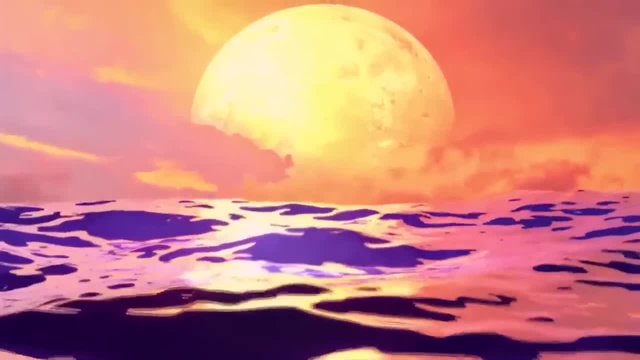 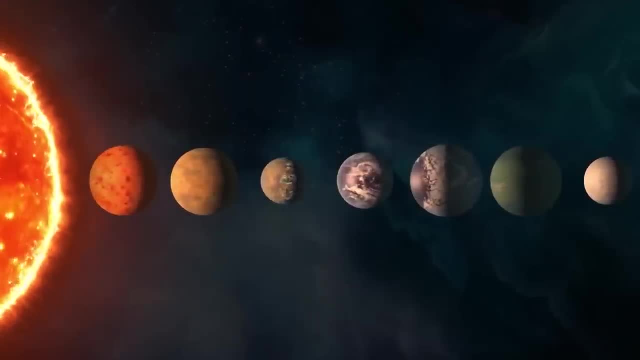 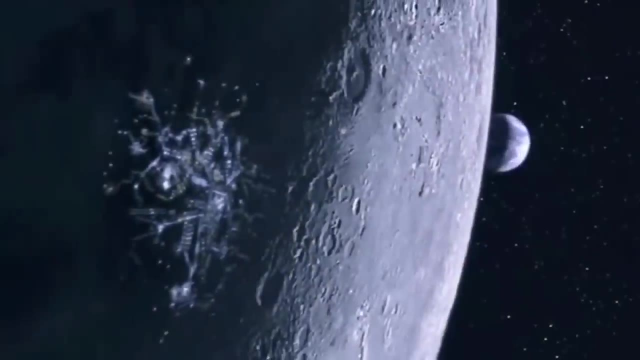 namely that the X-ray emission of Trappist One system approximately corresponds to the X-ray emission of Proxima Centauri, and the ultraviolet radiation produced by hydrogen atoms from the chromospheric layer of the star is already six times less than on Centauri. 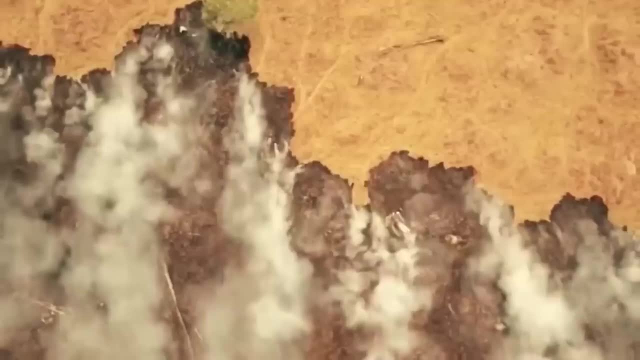 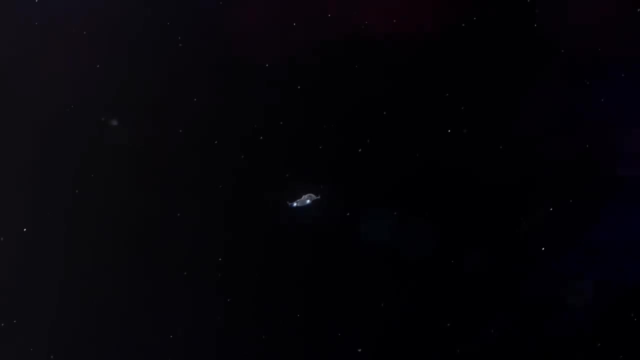 For this reason, the two closest exoplanets to the star, Trappist Oneb and Trappist Onec, could have lost their atmospheres and hydrospheres and hydrospheres- in a time span of two decades. 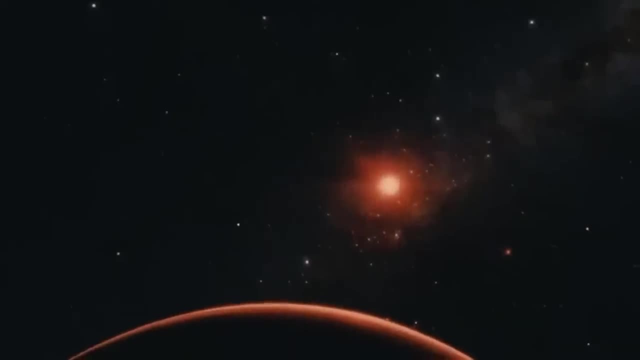 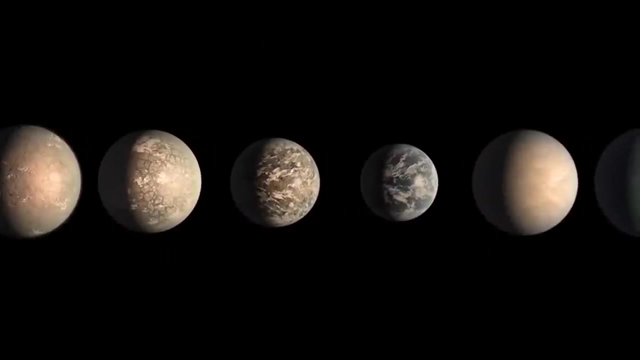 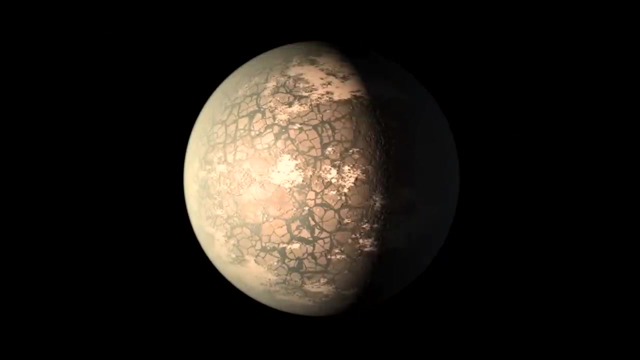 could have lost their atmospheres and hydrospheres and hydrospheres in a time span of two decades to three billion years if their initial masses were similar to Earth's. However, replenishment of atmospheric hydrogen and oxygen may occur through a reaction in which molecules of chemical compounds are broken down by photons. 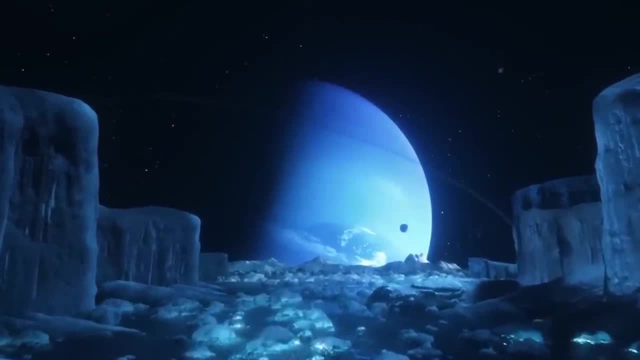 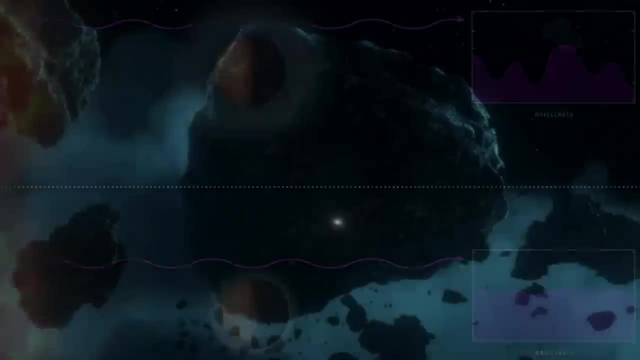 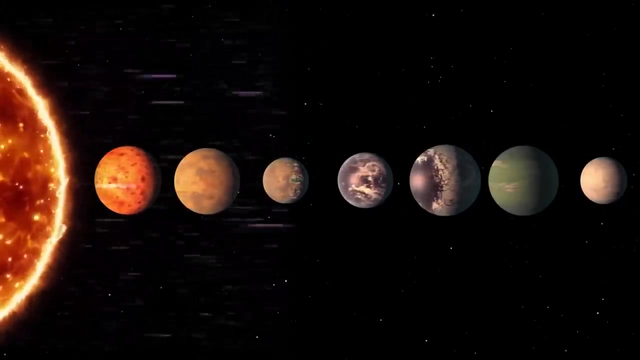 if the planets contain a lot of water in one form or another In their composition. Currently, the James Webb telescope has studied the exoplanet Trappist Oneb in more detail, where signs of a high-density atmosphere of the closest planet to the star. 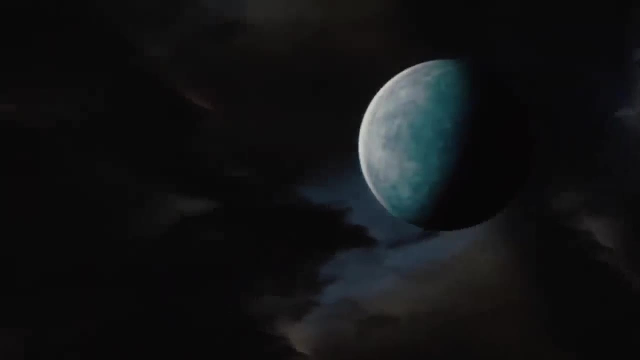 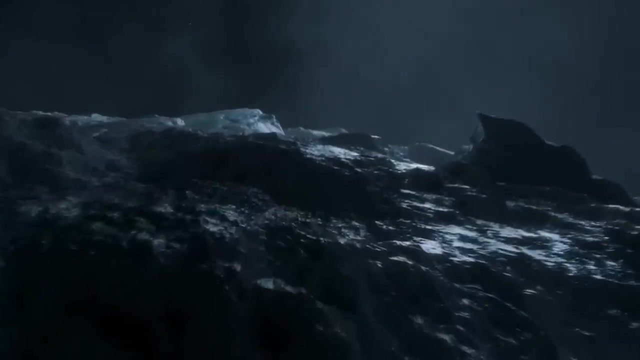 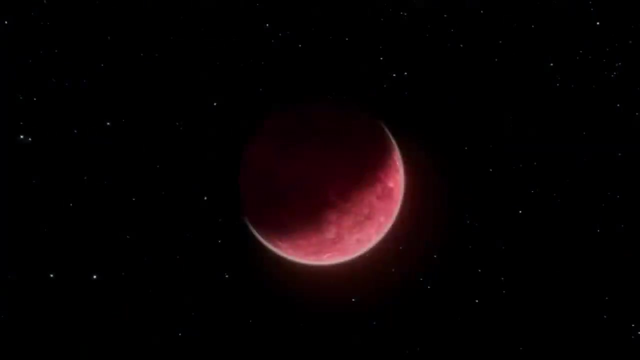 are not detected or optically thin. Further observations showed that this exoplanet receives four times more radiation than Earth from the Sun and is in tidal capture. The temperature of the day side of the planet was estimated with a maximum of 260 degrees Celsius. 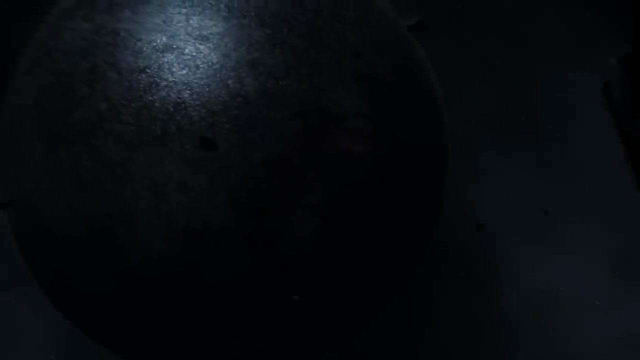 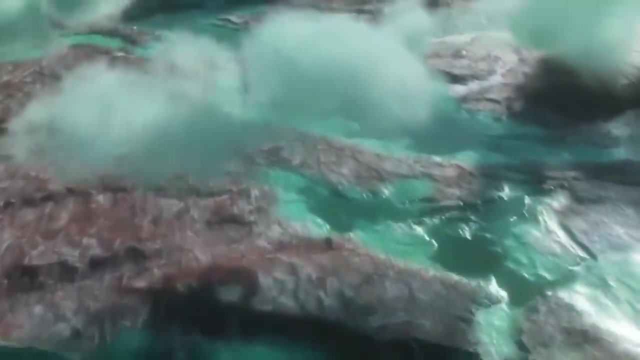 according to telescope data and most likely, the heat is not being distributed from the day side to the night side to the night side. Also, in the new study there's already data from a second rocky exoplanet, Trappist-1ec. 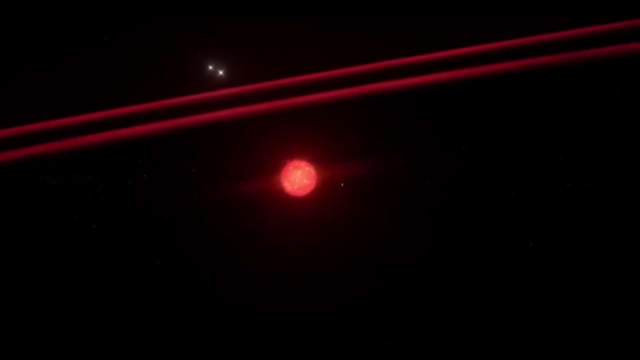 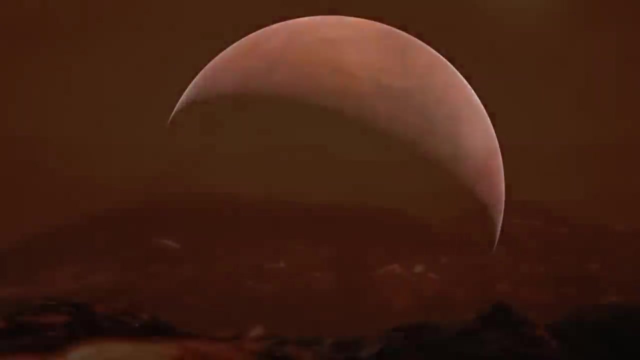 which is also in a tidal lock. The planet is interesting because it could be, in fact, a twin of Venus, since it's about the same size and receives the same amount of radiation from its star, but still not as harsh, because it has a daytime temperature. 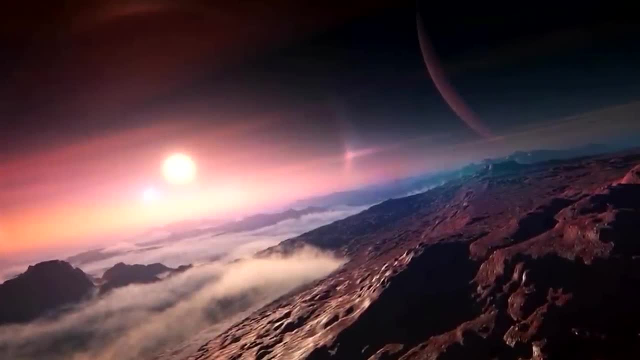 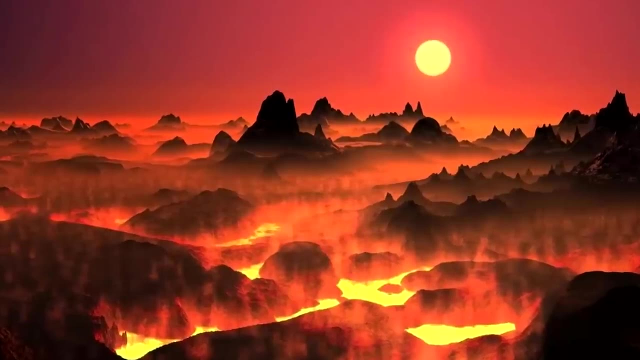 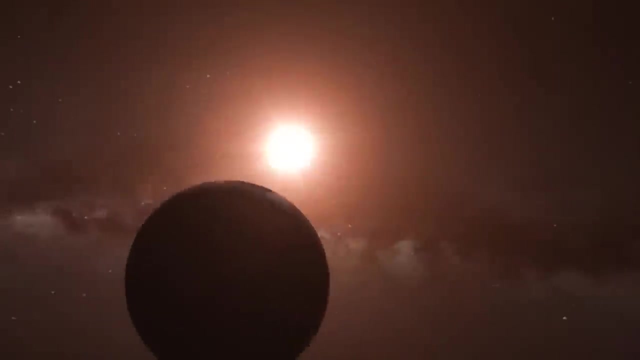 of about 160 degrees Celsius, And yet it still gives you an aggressive tan. although these first measurements do not provide definitive information about the nature of Trappist-1ec, They help narrow down the range of possibilities. The results are consistent with the exoplanet being essentially a rock. 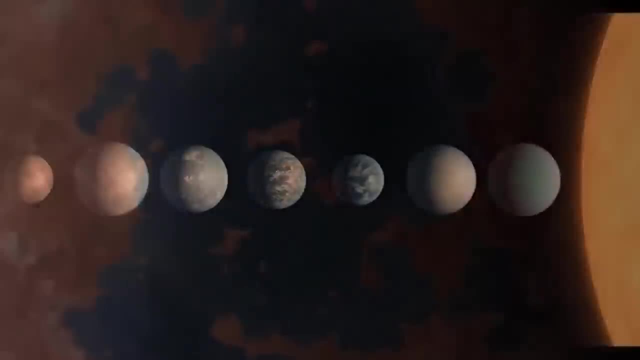 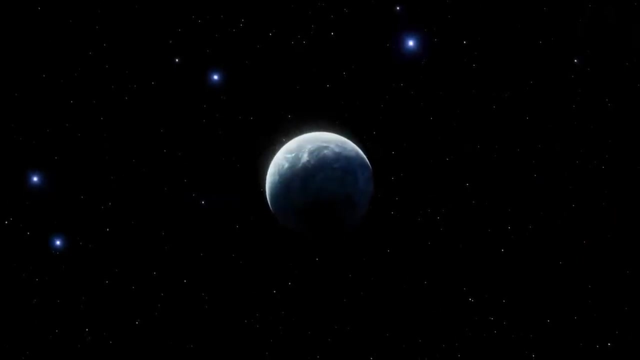 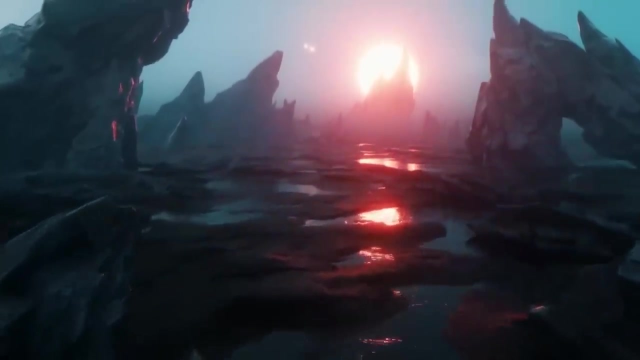 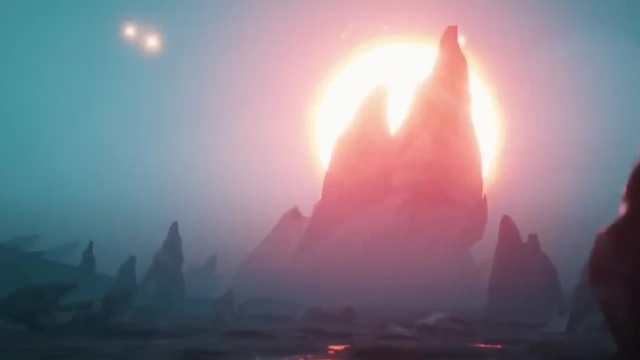 consisting of caves and rocks, with no atmosphere and no living aliens, but still not as harsh, because it has a daytime temperature of about 160 degrees Celsius, And yet it still gives you an aggressive tan, although these first measurements do not provide definitive information about the nature of Trappist-1ec. 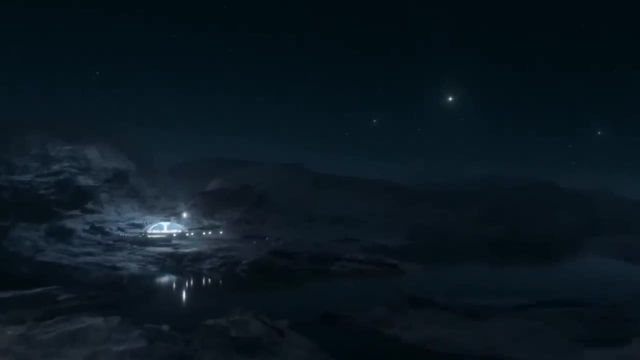 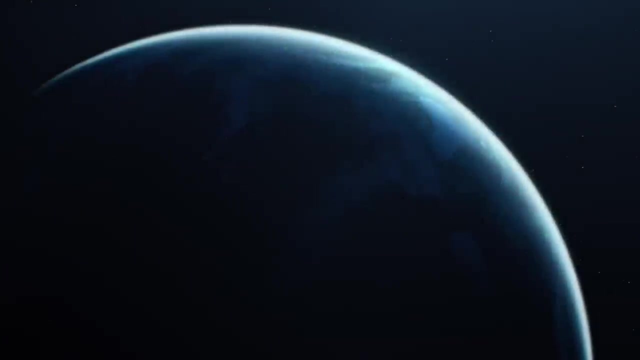 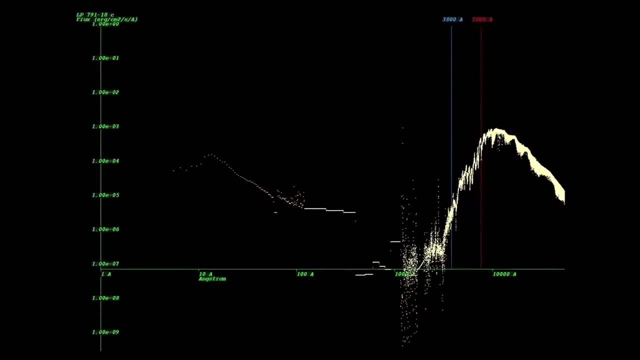 They help narrow down the range of possibilities. The results are consistent with the exoplanet being essentially a rock consisting of caves and rocks, with no atmosphere and no living aliens. The James Webb telescope is struggling currently studying galactic nebulae and black holes, but it also has another important goal. 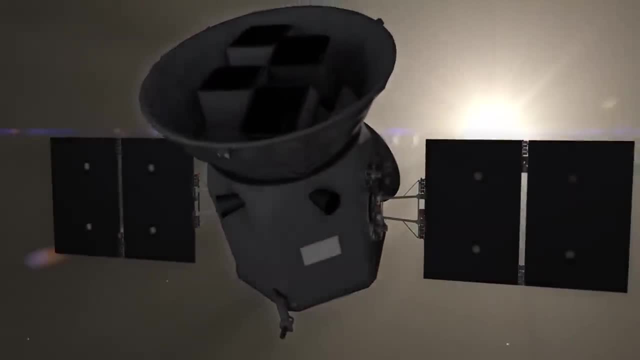 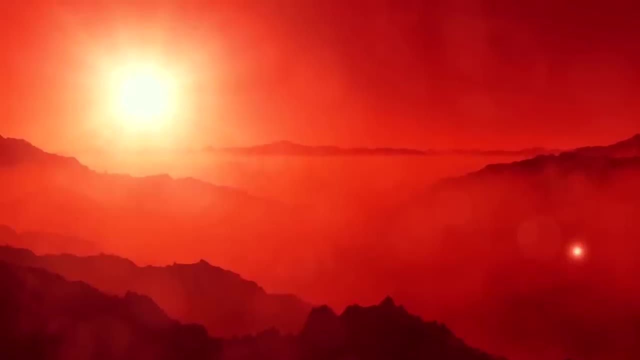 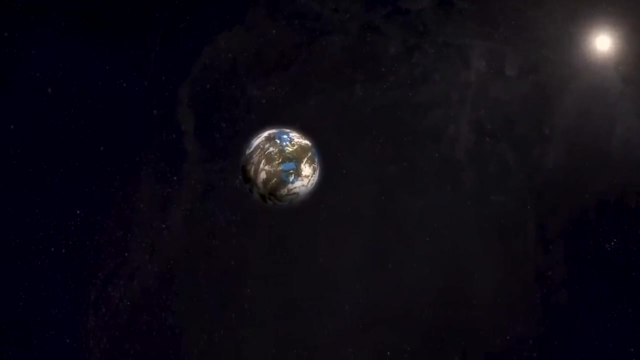 The star system LP 791-18, is 89 light-years away in the constellation Cratera and has at least two planets. The system was originally found by ground and space telescopes TESS and Spitzer. By observing the orbit of the Earth-sized planet, it was found that 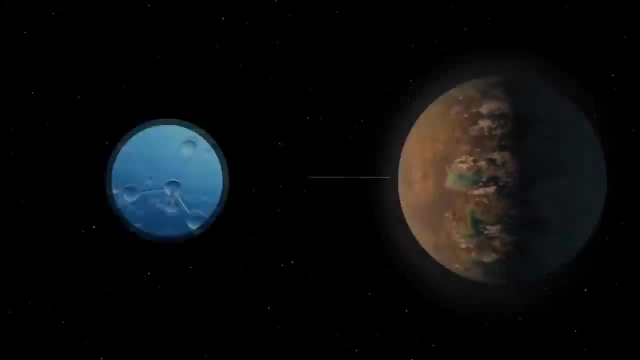 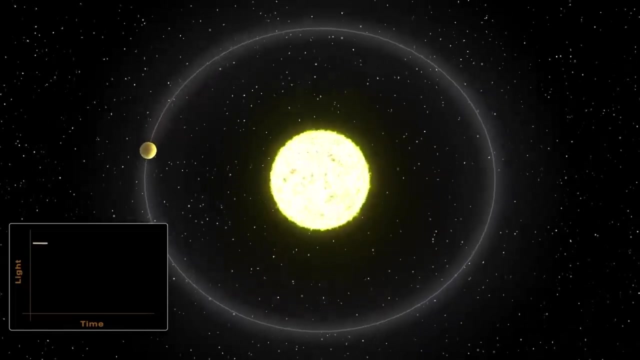 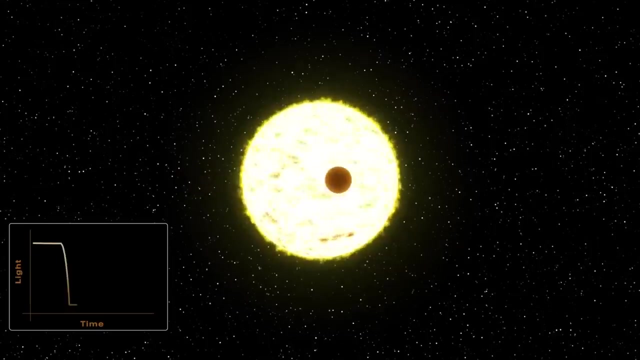 the surface has volcanic activity, which could lead to the existence of an atmosphere thanks to which water can condense. Moreover, the planet is on the inner edge of the habitable zone, which is neither too hot nor too cold for water in liquid form to exist not only in the atmosphere, but also on the 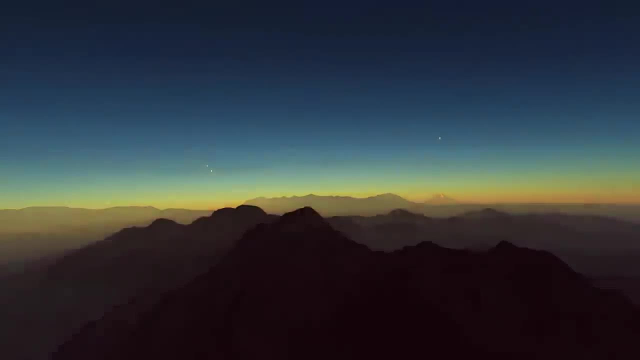 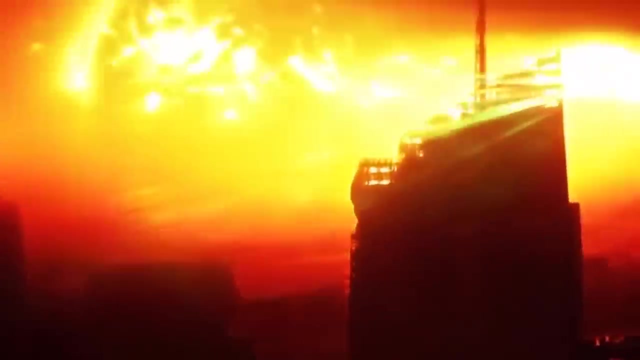 surface. In the surface, the planet is located on the inner edge of the habitable zone, which is neither too hot nor too cold for water in liquid form to exist, not only in the atmosphere, but also on the surface. In the same star system there is another planet, LP 791-18,, a more massive and larger gas giant. 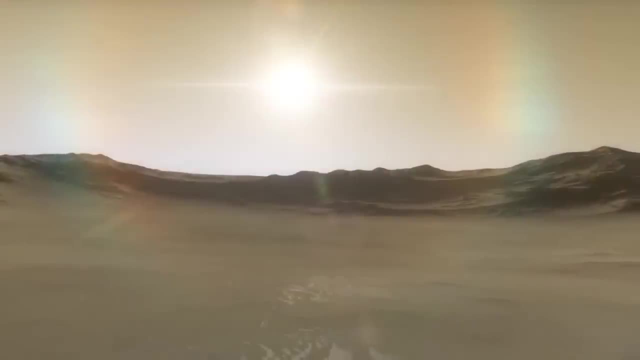 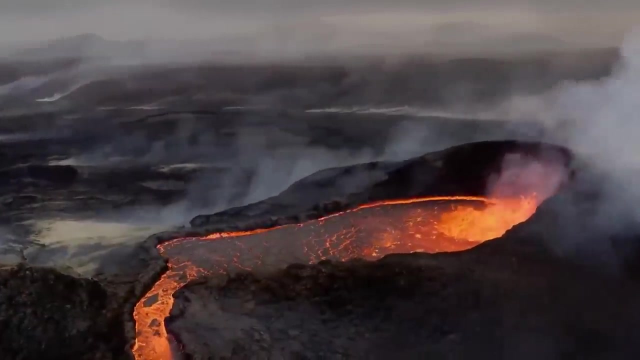 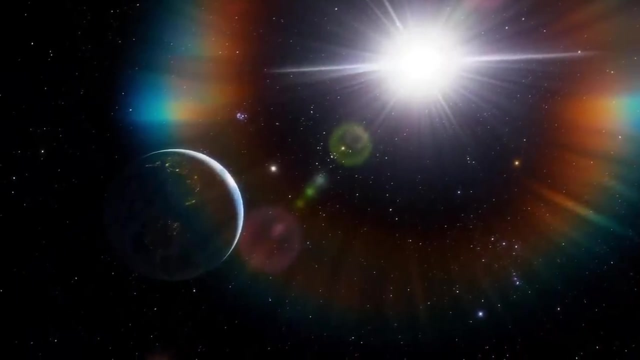 which in turn exerts a significant gravitational force on the Earth-like planet. The gravitational force also slightly deforms both the planet itself and its inhabitants, because of which it has observed high volcanic activity. Similar processes occur on one of the moons of Jupiter. 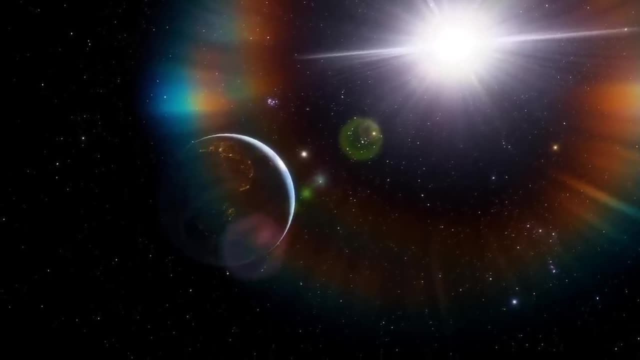 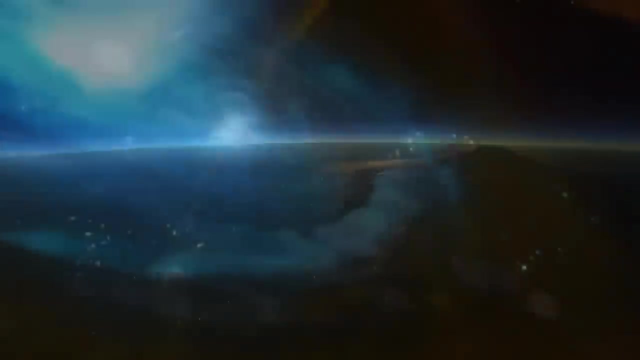 Researchers have already received approval to study the atmosphere of LP 791-18 with the James Webb Telescope, thanks to which it will be possible to learn more about the planet. The James Webb Space Telescope is now practically the world's premier space observatory. 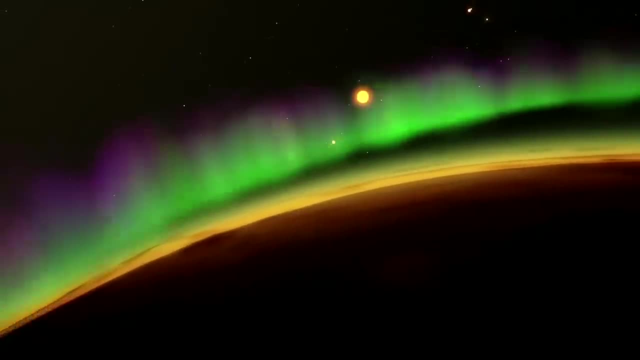 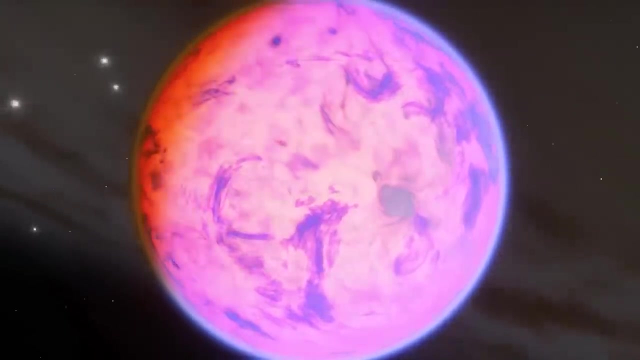 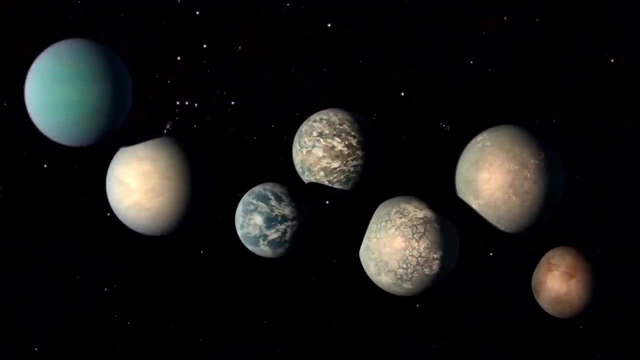 allowing us to peer into distant worlds around other stars, explore mysterious structures and learn more about the origins of the universe and our place in it. So far, nearly six thousand exoplanets and four thousand star systems have already been confirmed, with several thousand 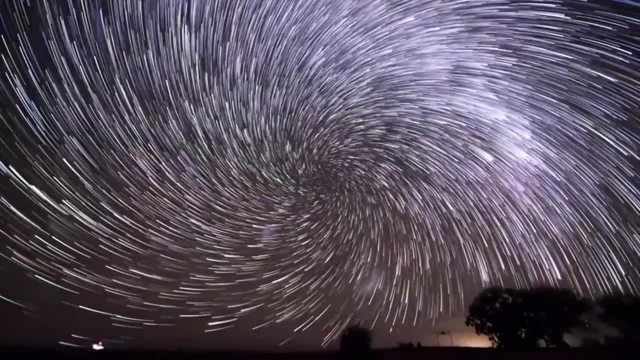 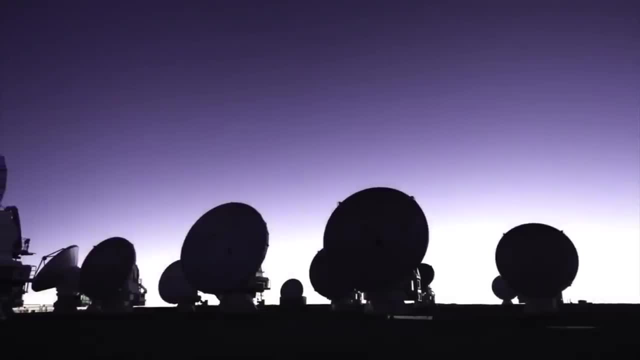 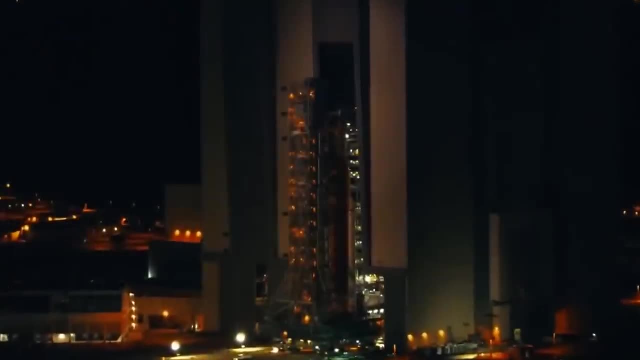 more candidates awaiting verification. Of course, the public's attention is focused on planets that are as Earth-like as possible. We have not given up hope of finding intelligent life in space, However. the bulk of distant worlds look very strange to us. There are often conditions there. 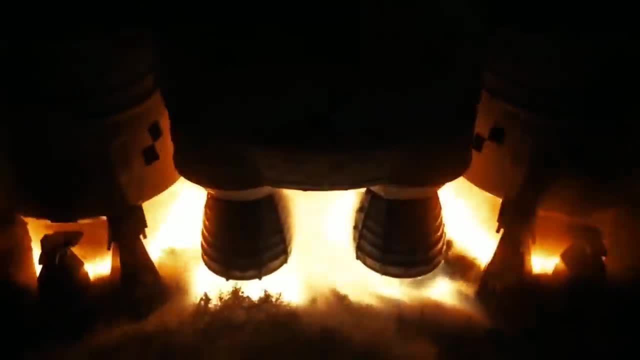 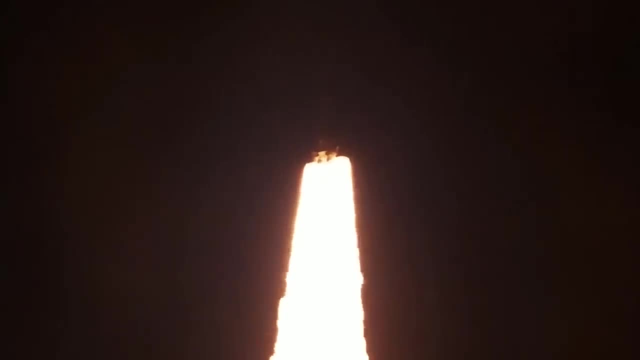 that we can't even imagine. After all, science fiction writers have long advised us that the universe is a very complex and complex universe. Science fiction writers have long advised people not to fixate on our carbon-based form of life. There may be much in the universe beyond our 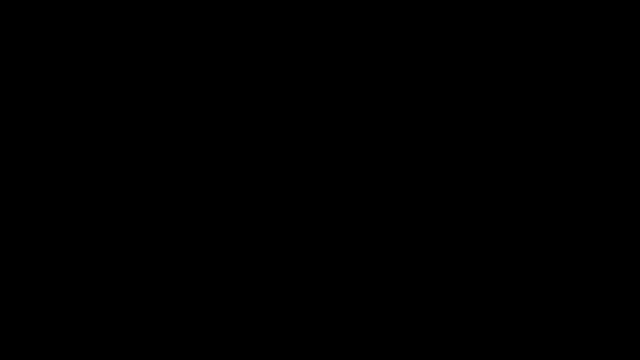 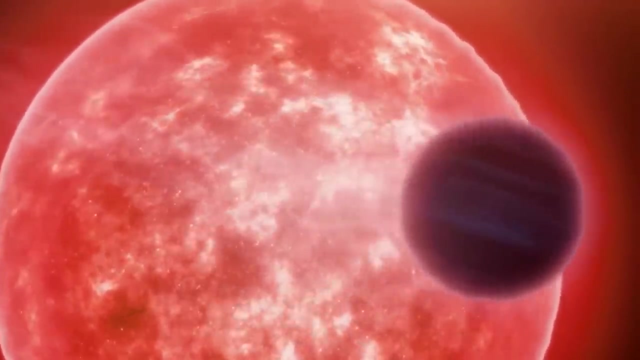 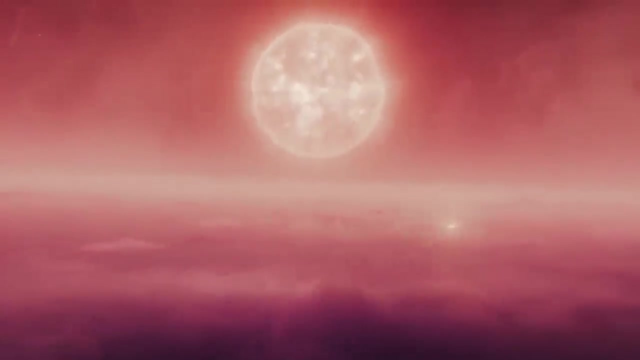 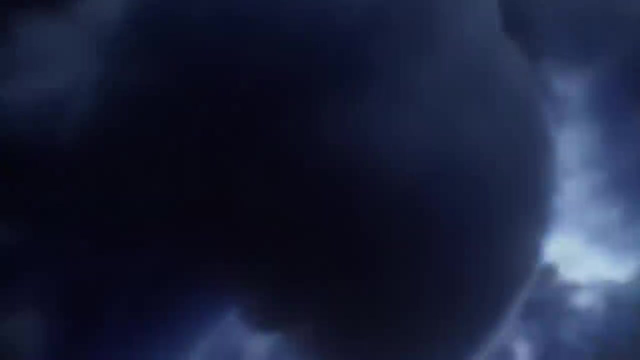 understanding, but science exists to push those boundaries. However, for many scientists, science is simply a false narrative, which is just a false lie. The universe and the other planets are not just worlds, but are different universes of some form, For instance, the two planets that exists in space called the stars on. 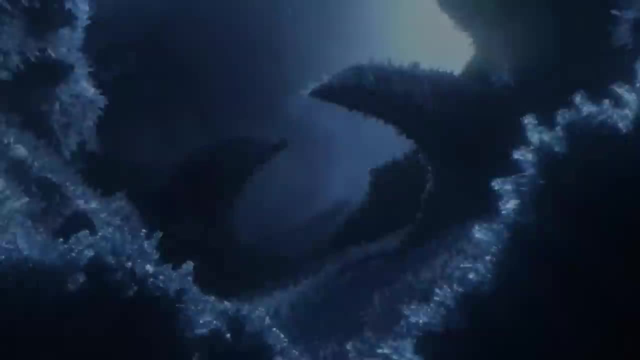 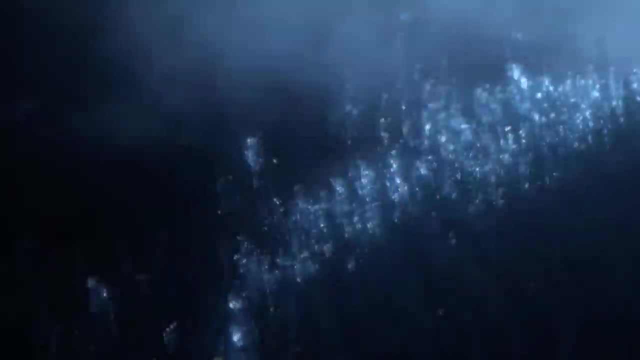 the right are Вс, which have a little doubt about their origin and their originality. Thus they are the same as the star and have no idea that the star is the same as the star in the Universe. But science has so far foiled the existence of the universe's. 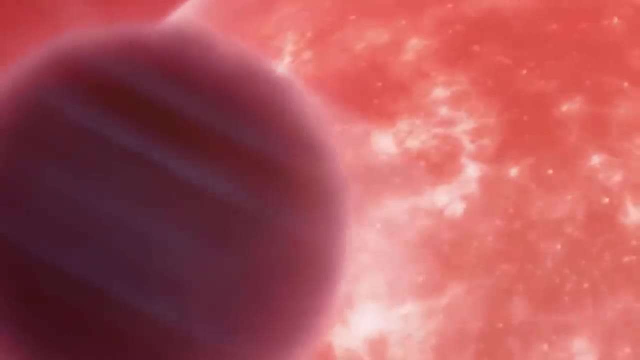 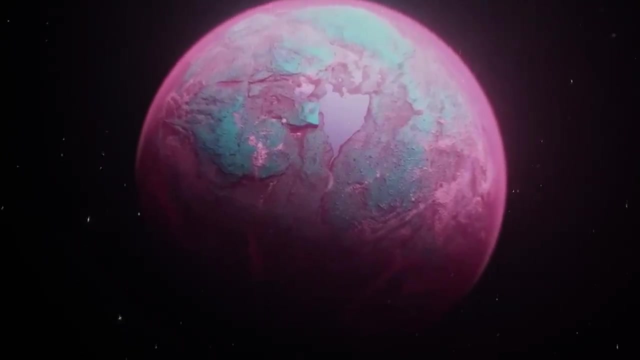 actors. as a result of their confusion and confusion, they have been deceived by the image of their own existence. For example, the sun beats the stars, or the stars are the same as the sun because it is the same planet, and公a and the stars are the same. 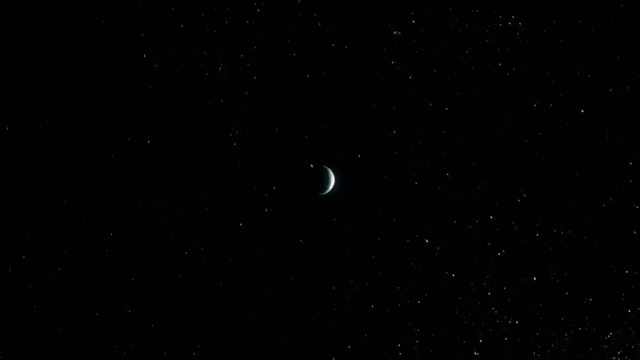 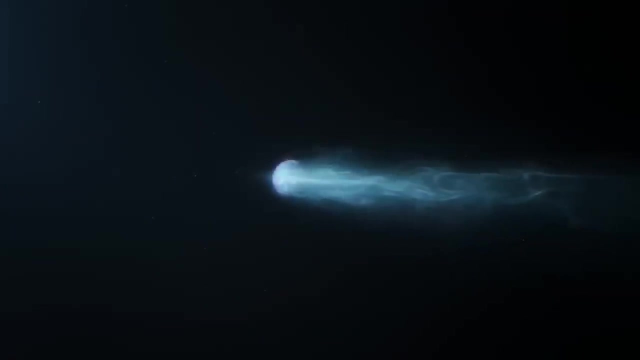 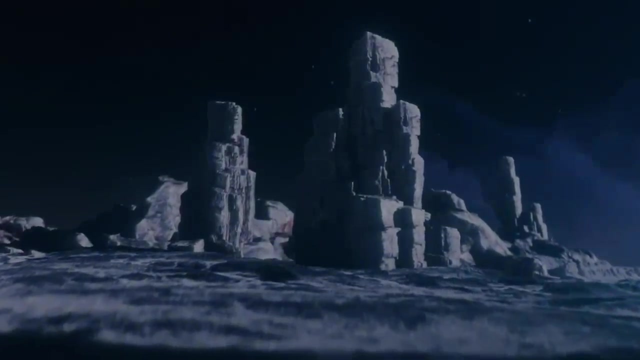 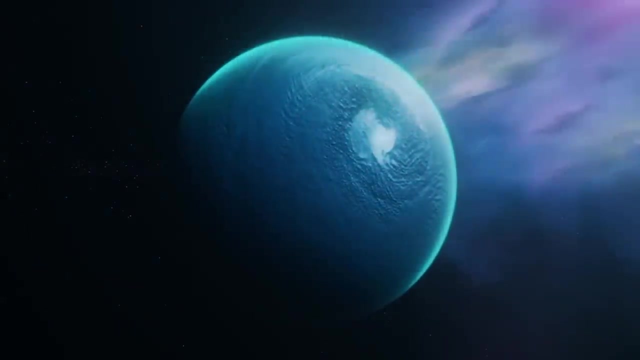 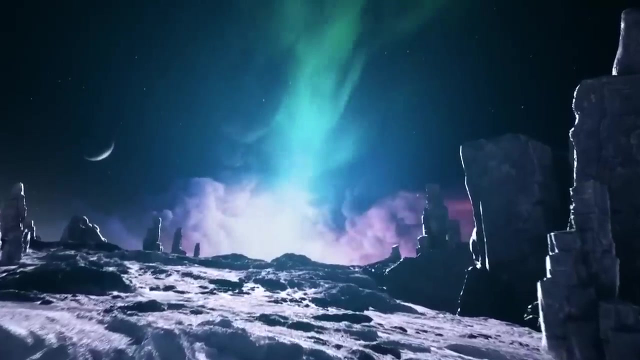 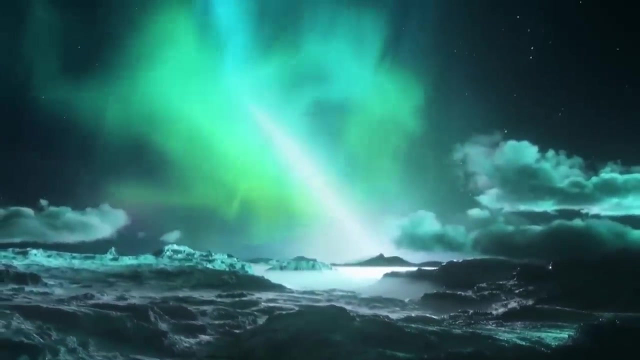 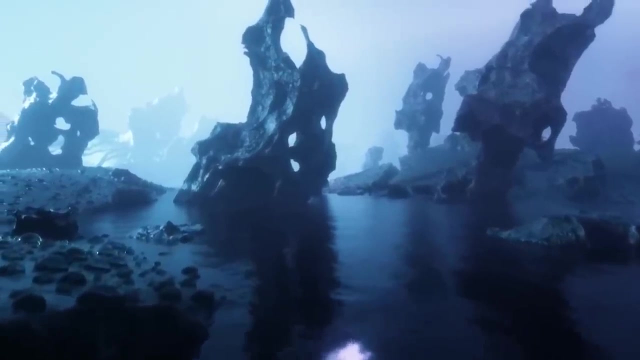 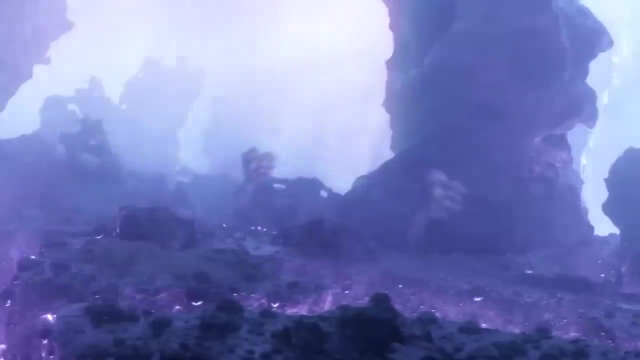 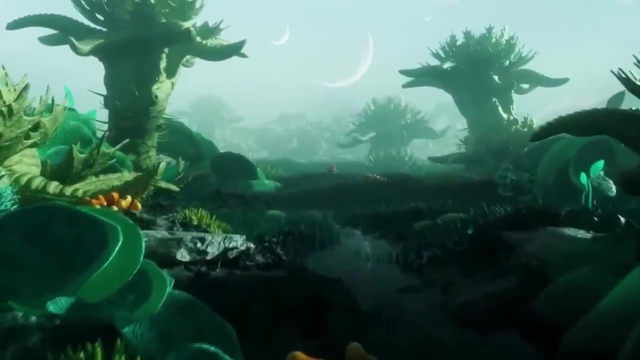 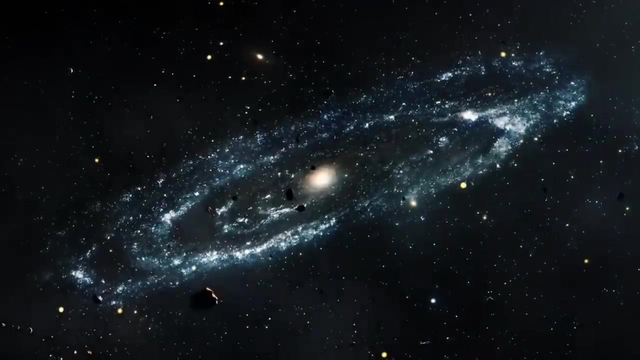 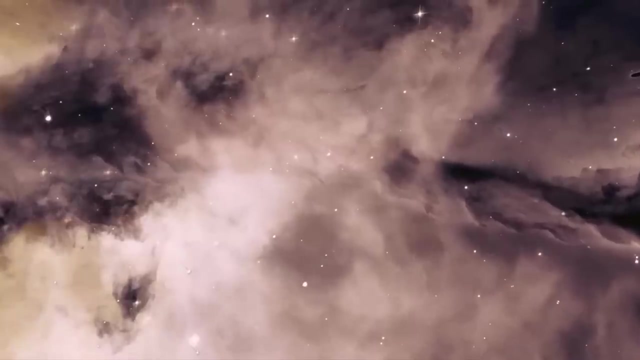 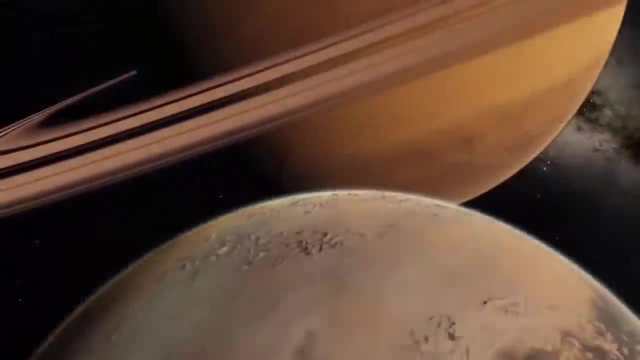 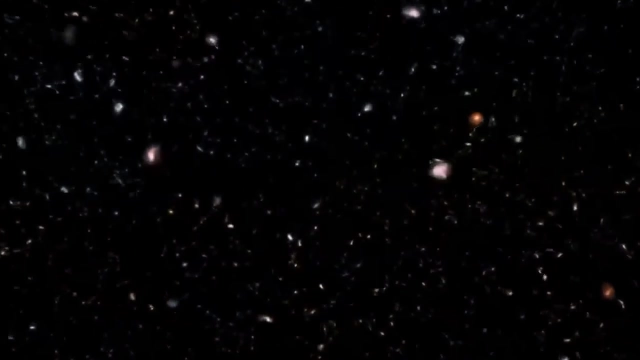 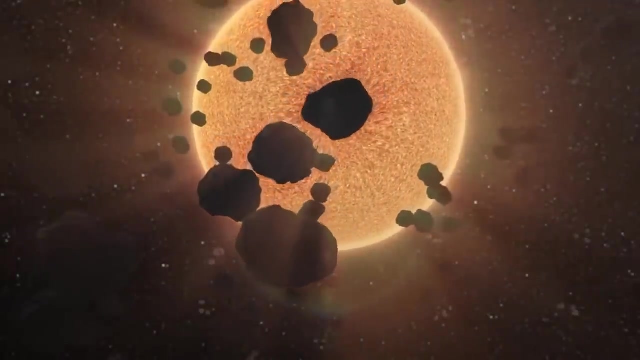 as the sun, and so are the stars, and so are the stars, and the stars are different. We'll be right back. We'll be right back. We'll be right back. We're happy today to join us on this heavenly journey that reveals the subtleties of the most mysterious hero of the universe. 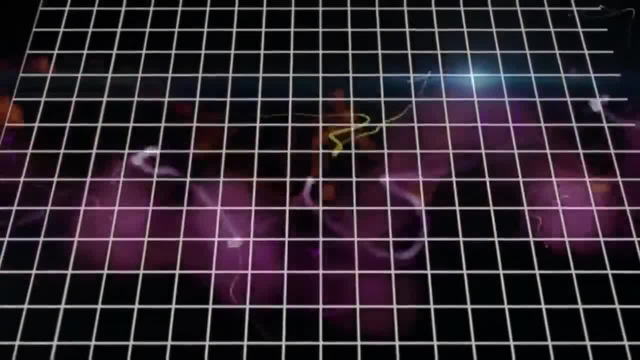 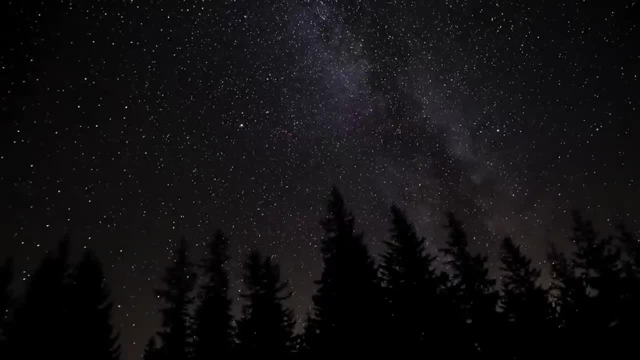 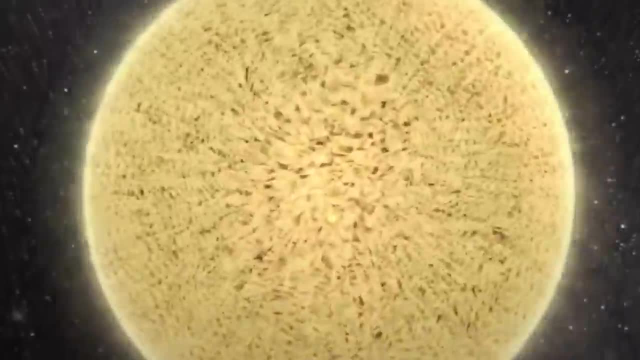 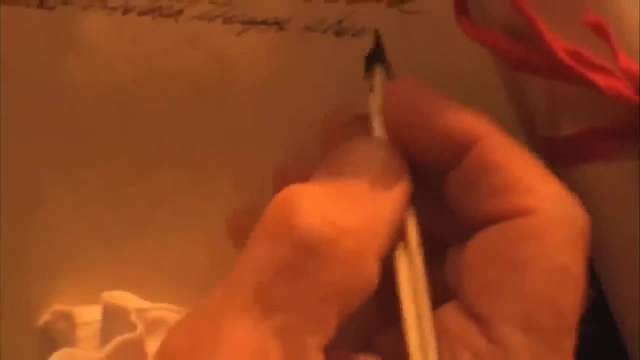 Gravity Universal, fundamental interaction between material bodies. It is a fundamental force in nature that acts on every object in the universe, whether tiny or massive. To fully understand this concept, it is necessary to turn to the history of our understanding. The concept of gravity was pondered by the sages of different countries and eras. 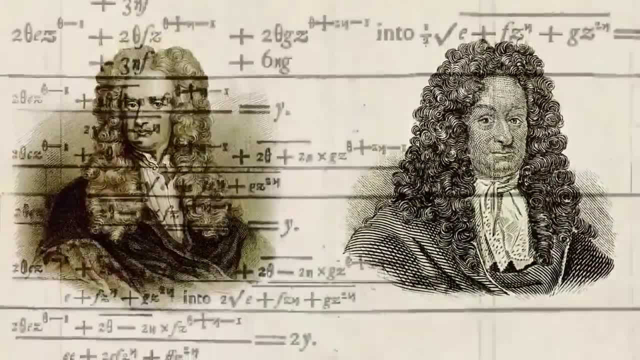 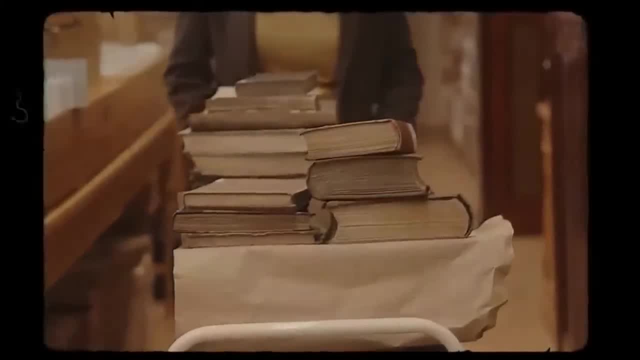 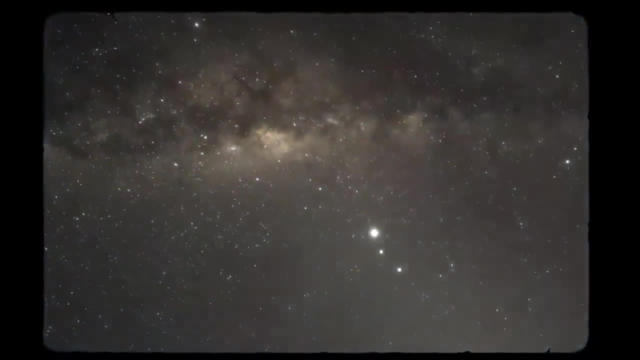 They were accurate and not very true and fabulous. But over time, Sir Isaac Newton's law of universal gravitation and Albert Einstein's general theory of relativity have become the foundations of our knowledge of gravity today. Yes, Newton's law of universal gravitation. 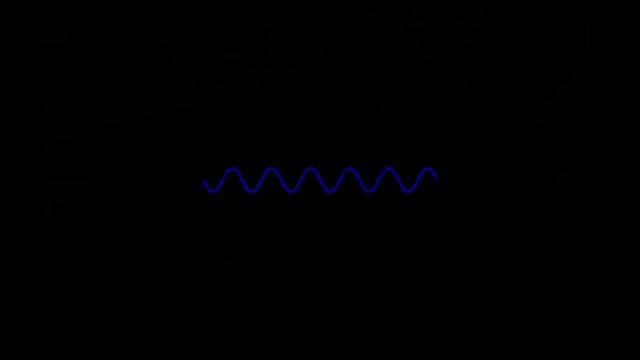 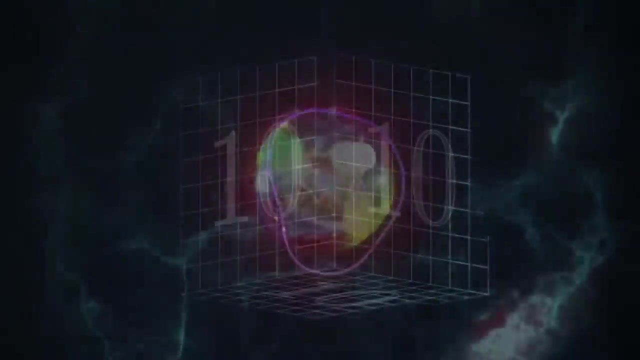 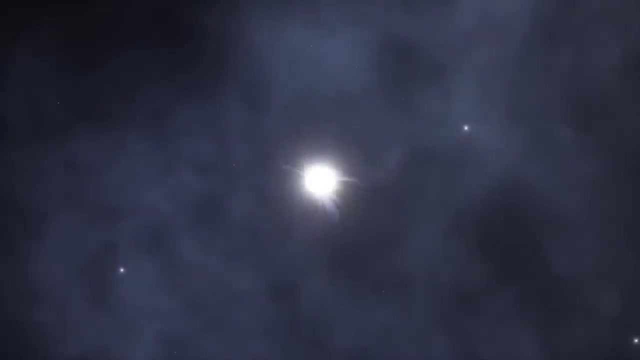 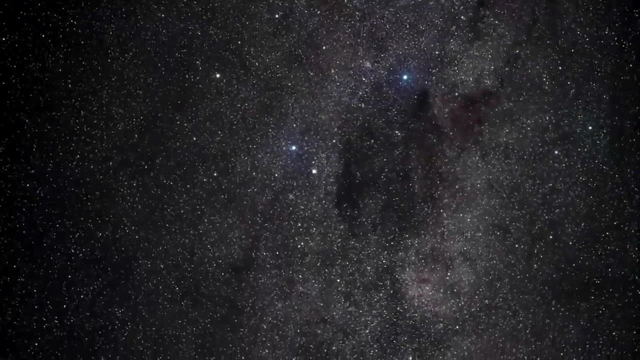 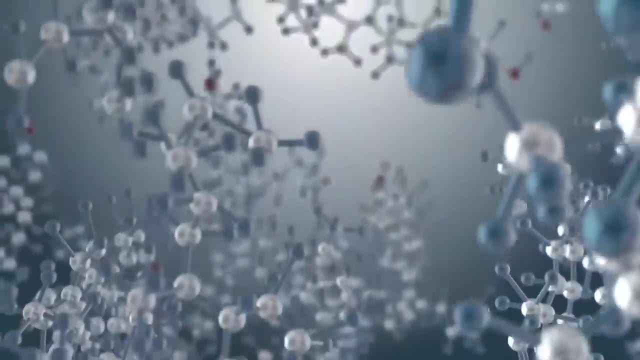 However, Einstein, in his general theory of gravity, said that the force of gravity is greater than the force of the object. However, Einstein, in his general theory of relativity, suggested that gravity is not just a force acting between masses. Instead, it is a curvature of spacetime caused by the presence of a mass of energy. 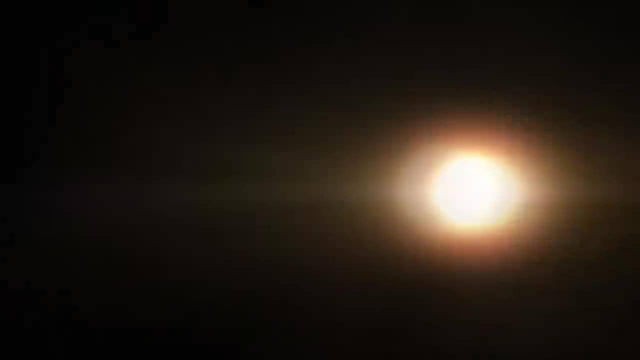 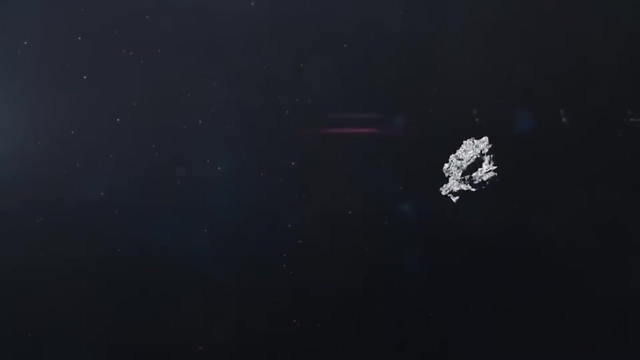 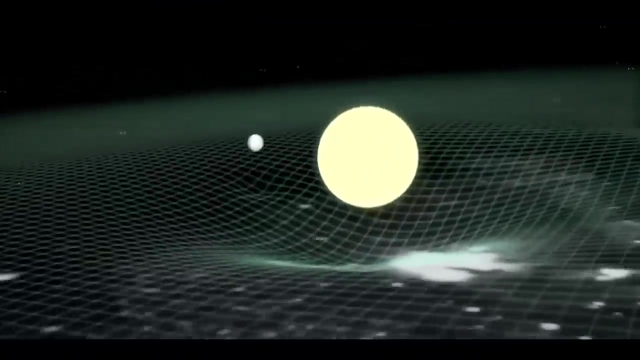 From this point of view, objects such as planets and stars move and are influenced by the curvature of spacetime, which leads to the fact that we perceive it as a gravitational force. So what is gravity Power? But it depends where, For example in Newton's mechanics, there is certainly a force. 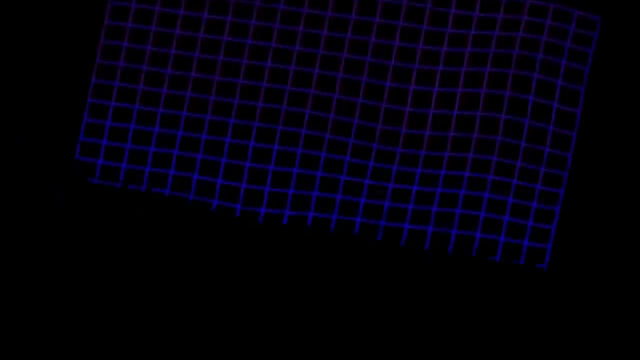 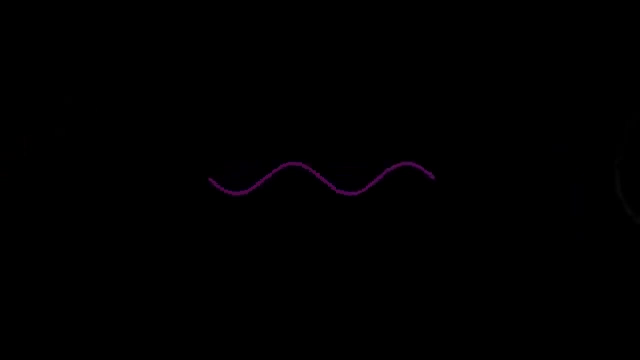 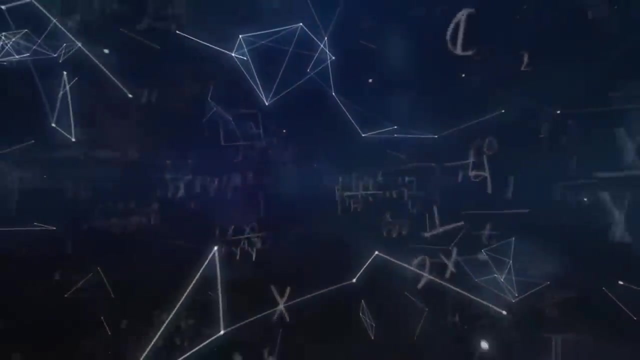 In classical theoretical mechanics one can consider a certain gravitational field that is there. every point in space has such a characteristic as the potential of the gravitational field. Through the potential it is possible to calculate the force that will act on a body with a particular mass placed at this point. 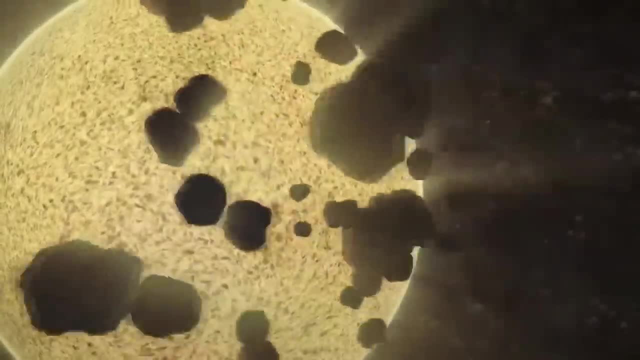 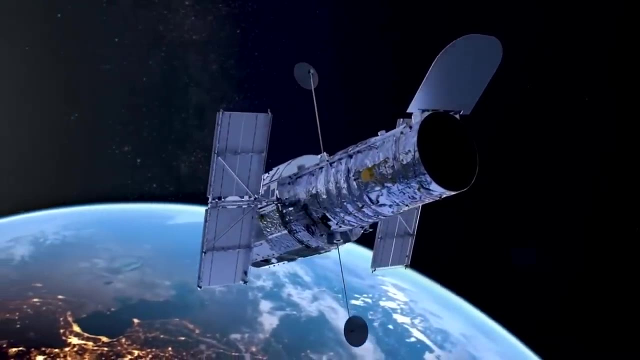 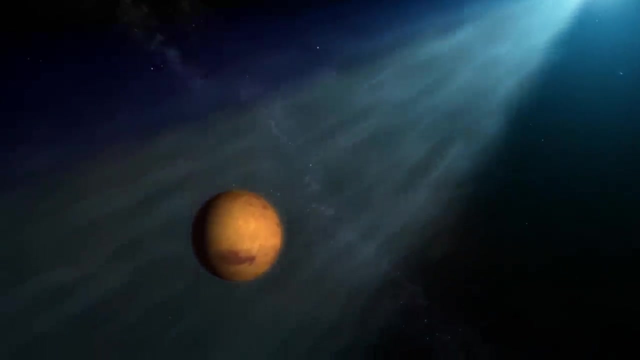 And you can also calculate the trajectory of a body in a gravitational field with a potential known to us. This means that tasks, for example, to launch an Earth satellite or calculate the period of the comet's revolution, are successfully solved with this approach. 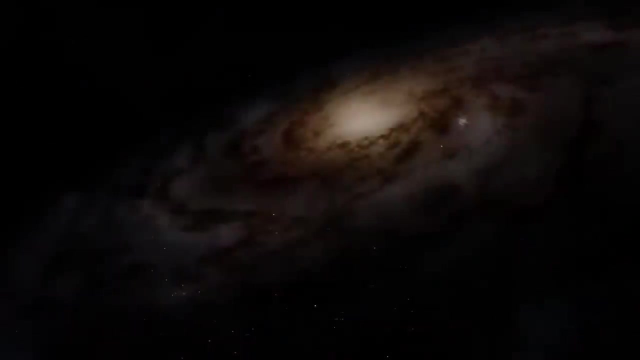 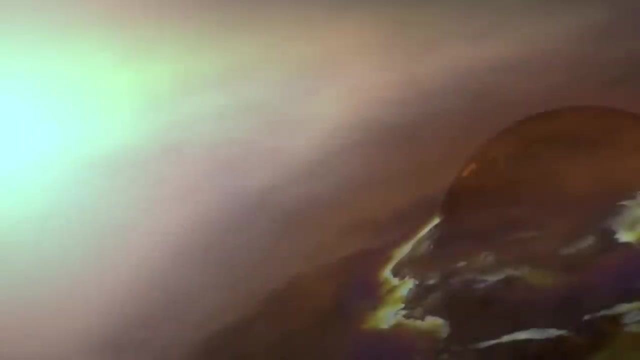 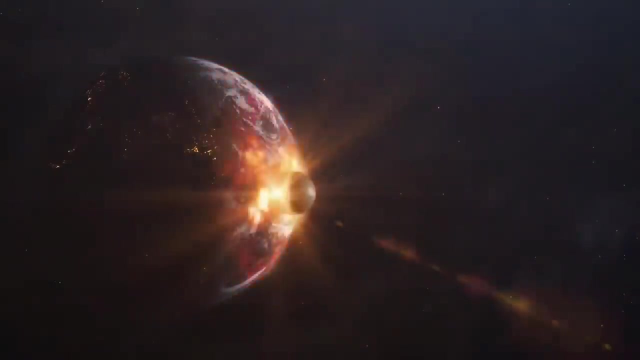 So you may well consider gravity a force in a number of cases, But there is no gravitational field in the general theory of relativity. In Einstein's theory, gravity is not a force. We have to use it where we need high accuracy of calculations or where we have very large 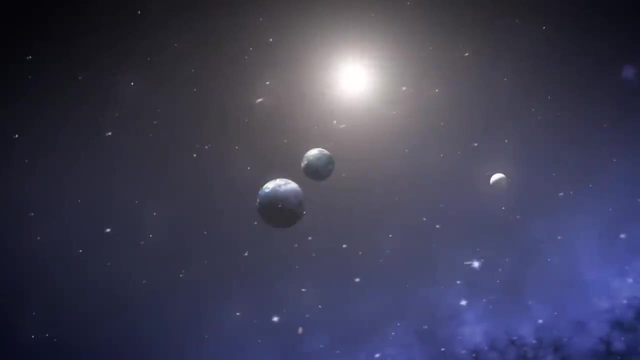 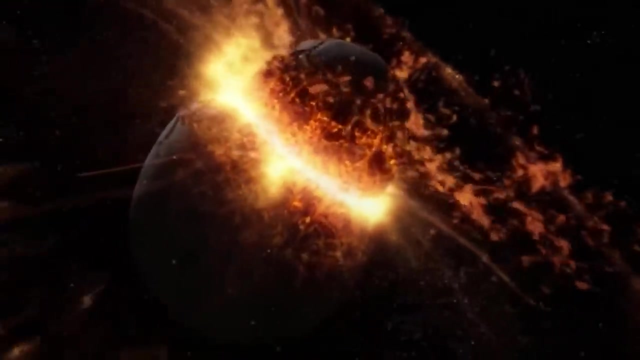 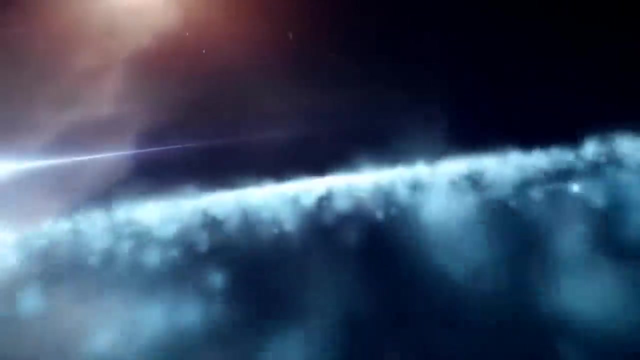 compact masses, for example the fusion of neutron stars. In other words, gravity in the approximation of small velocities compared to the speed of light and weak gravitational interaction is described by Newton's theory of gravity or described by Einstein's general theory of relativity. 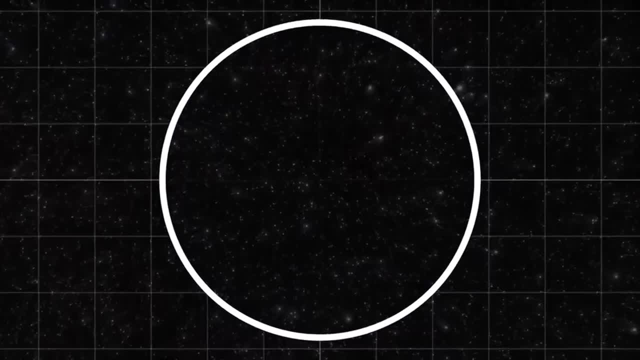 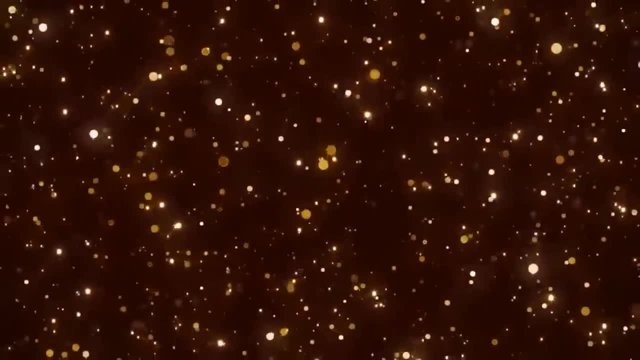 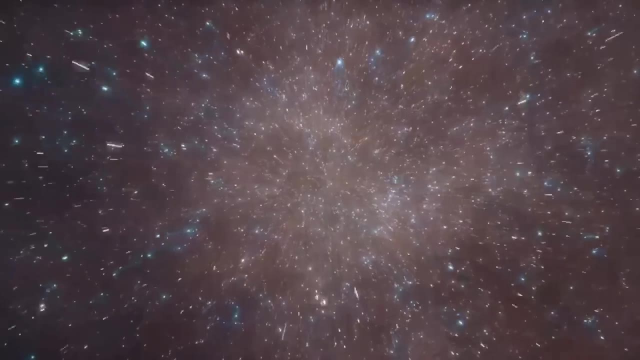 But in the quantum limit. the gravitational interaction is supposedly described by the quantum theory of gravity. Well, now a new hypothesis has been put forward, That if the three fundamental forces have a corresponding quantum theory, then there must also be a particle behind gravity. 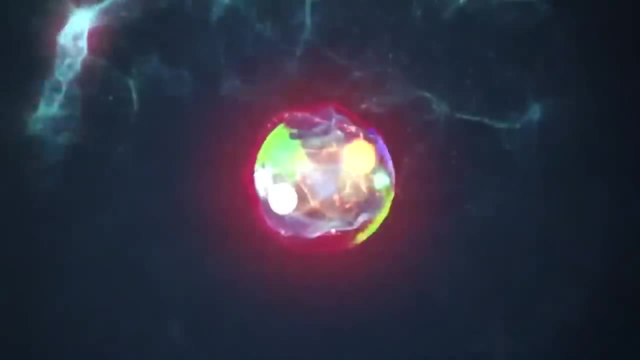 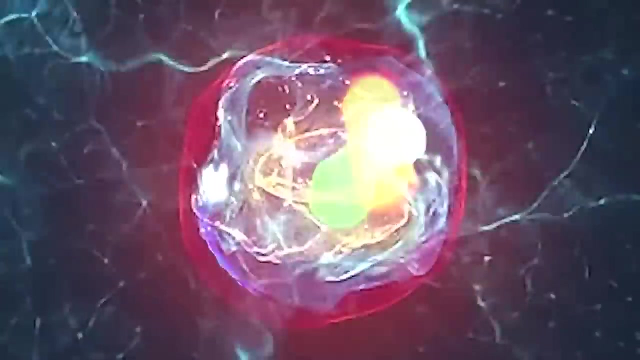 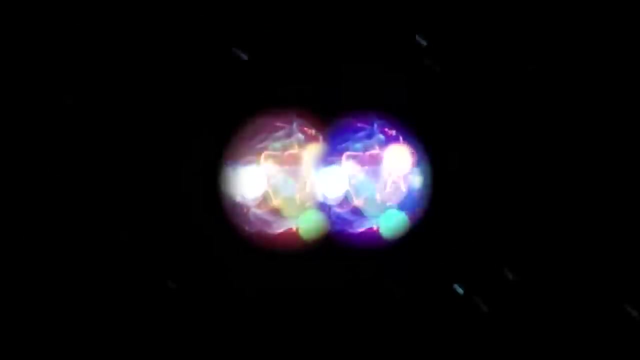 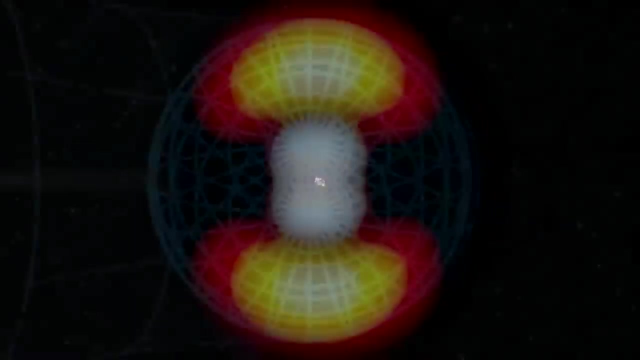 In an attempt to combine gravity with quantum theory, there is a hypothetical particle called the graviton, the carrier of gravity, The gravitational interaction, In fact a quantum of the gravitational field. without electric and other charges, The particle supposedly always moves at the speed of light. 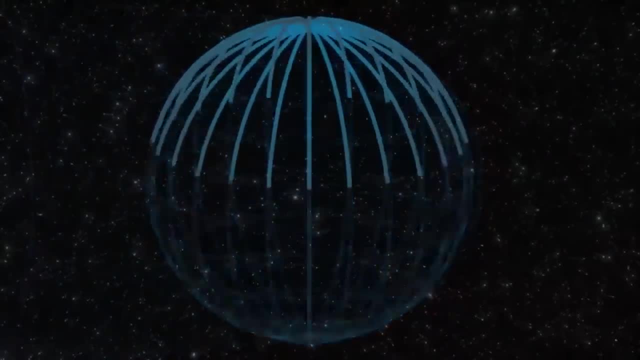 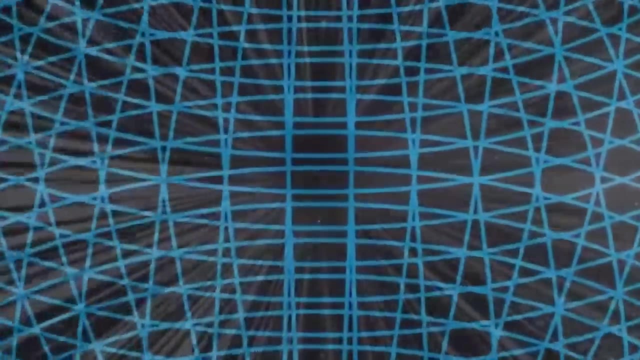 And although gravity is strong on a cosmic scale, it is quite weak on a small scale, So weak that when a magnet attracts a paper clip, the paper clip overcomes the gravitational force of the entire planet And moves at a speed of light. And moves in the direction of the magnet. This means that one graviton, if it exists, must be very weak, And to measure it you need a detector the size of Jupiter. But still there is a theory that assumes the existence of a graviton. 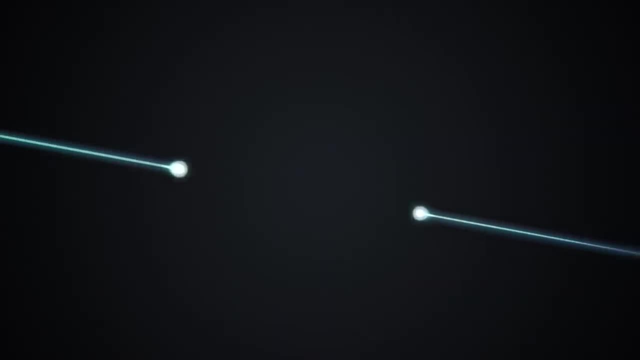 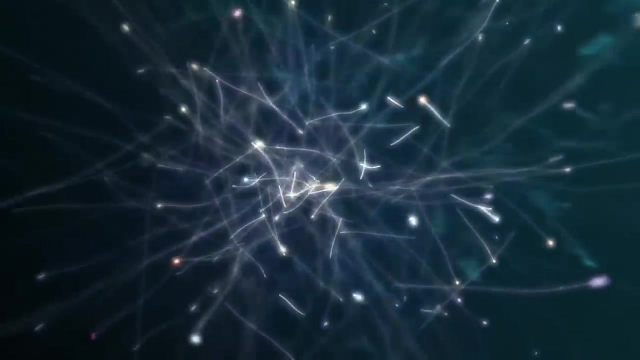 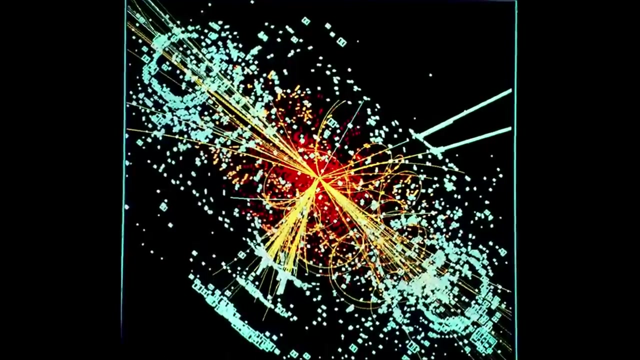 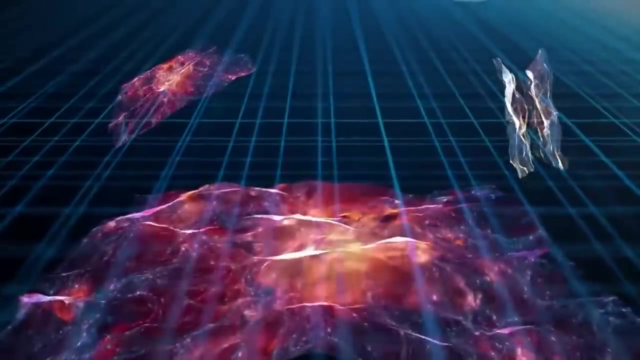 After a decade of silence due to mathematical inconsistencies, the same string theory was revised and refined, A promising contender for the creation of a quantum theory of gravity. The fact is that, in string theory, mathematical calculations point to a universe with ten dimensions. However, these spatial dimensions are too small to see. 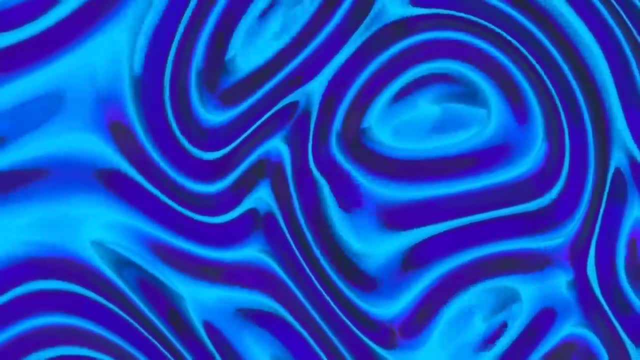 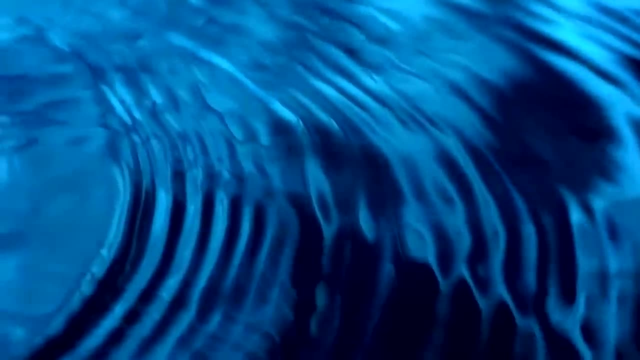 And, as we know, gravitational waves carry information about their origin and about the nature of gravity. Moreover, today we can even listen to a signal about gravitational waves transformed into sound, For example, When two black holes were formed. When two black holes were formed. 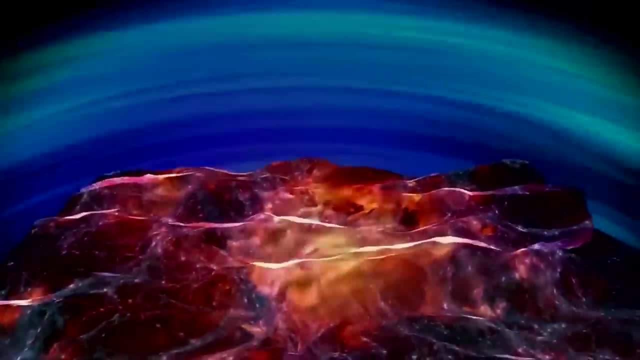 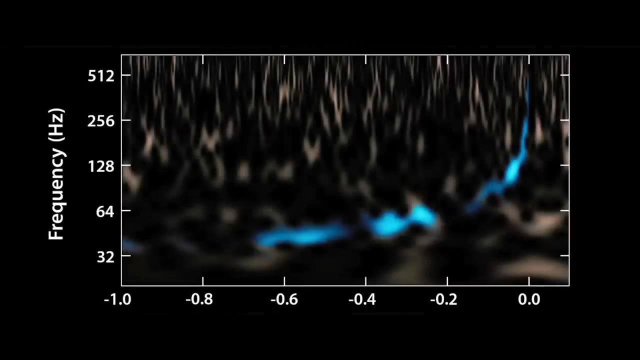 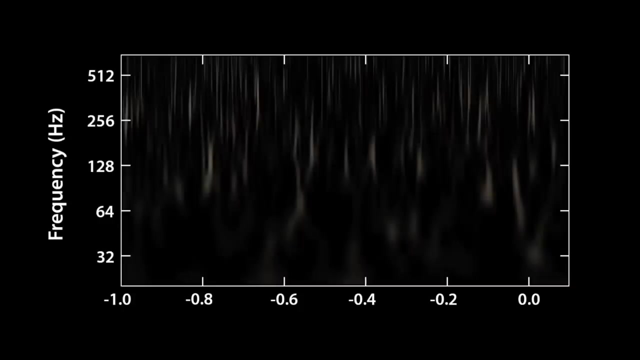 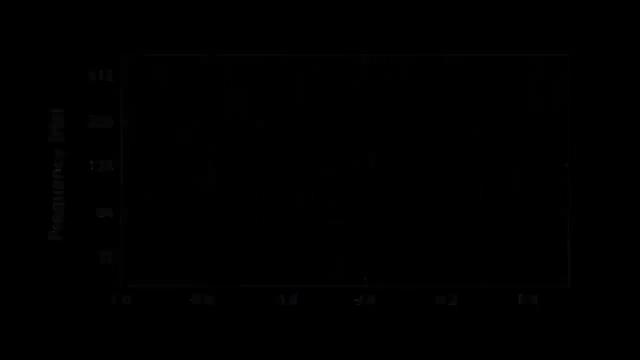 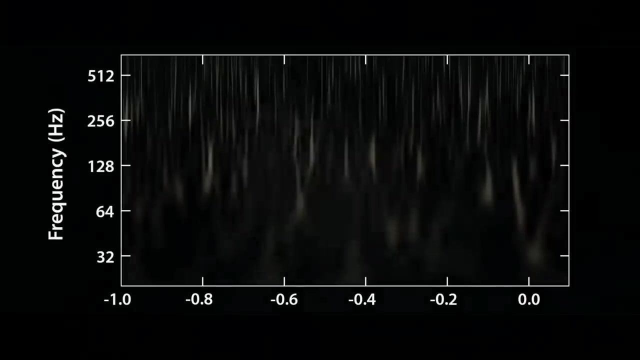 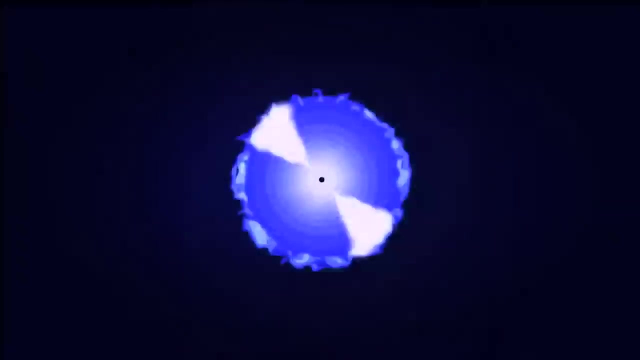 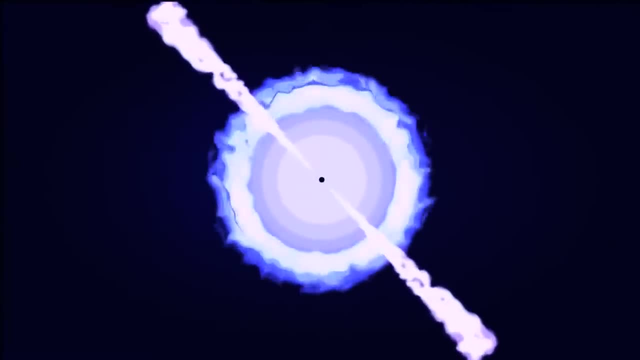 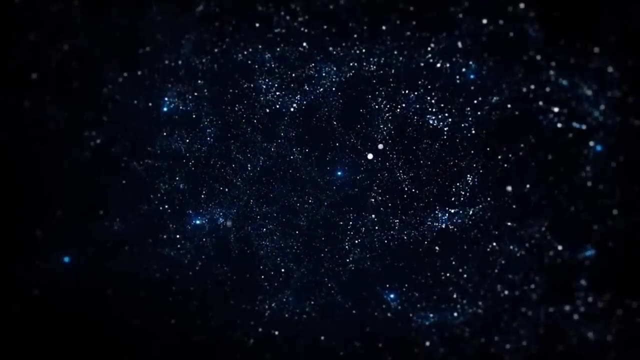 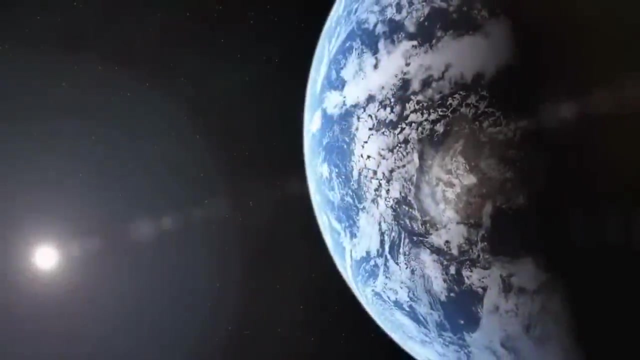 result of the curvature of space-time under the influence of massive objects. The existence of the graviton particle still remains insurmountable, since science has not yet provided experimental evidence of its existence. Despite this gravity, whatever it is, it is. 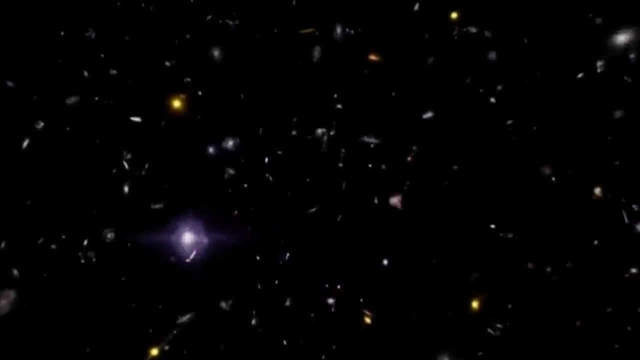 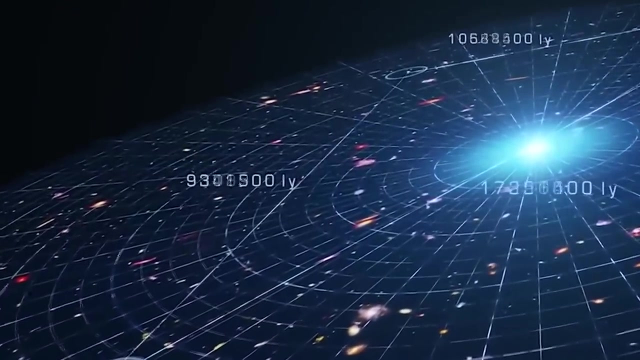 We see it and it affects us and the entire universe as a whole. Its importance is difficult to overestimate. Firstly, it is the formation of celestial bodies. Gravity is responsible for the very existence of celestial bodies, such as stars, planets. 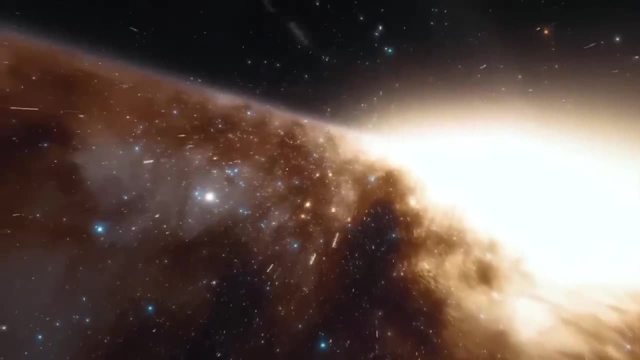 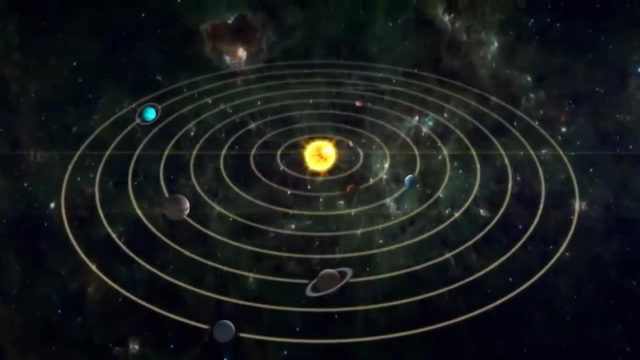 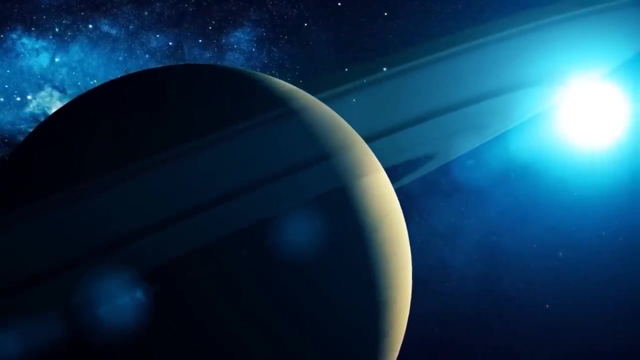 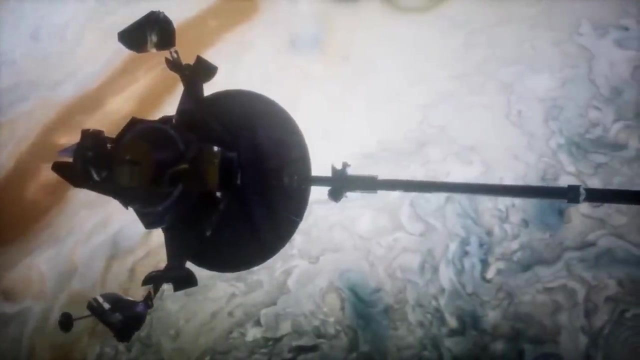 and galaxies. It compacts dust and gas, initiating nuclear reactions that ignite stars. Secondly, gravity is responsible for the harmonious orbits that define our cosmic neighborhood. The gravitational pull of the sun keeps our planet and other celestial bodies in the solar system and does it in their places. 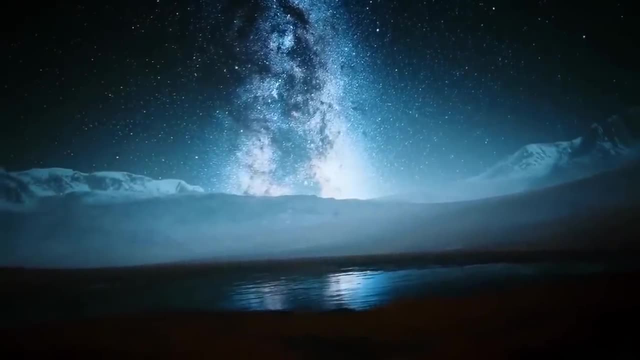 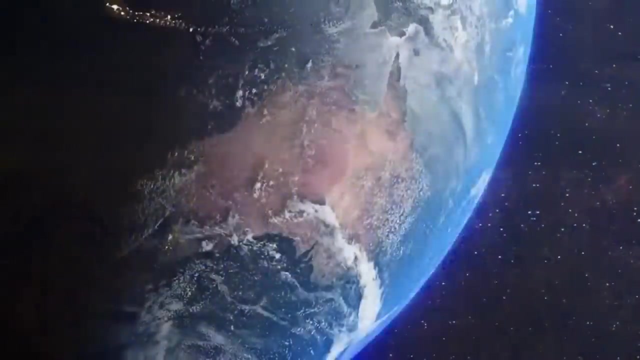 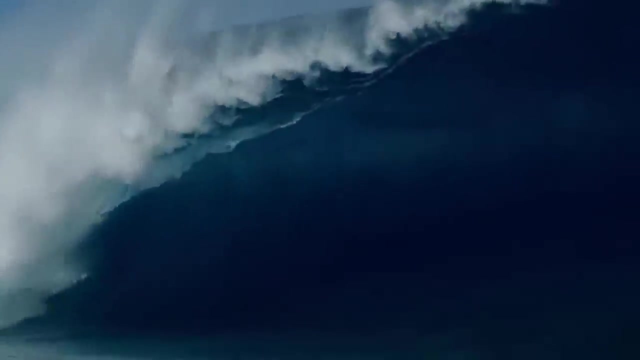 Thanks to this delicate balance, the earth maintains an optimal distance from the sun, receiving the necessary amount of energy to support life. Thirdly, the tides of the earth. Lastly, the tides of the ocean on our planet arise mainly as a result of the gravitational 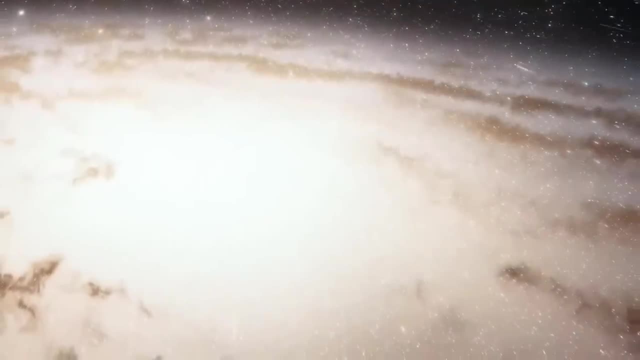 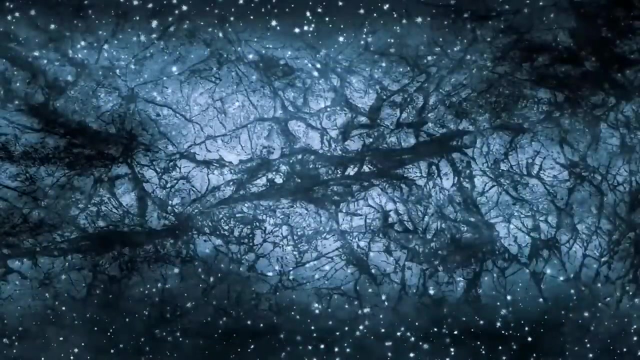 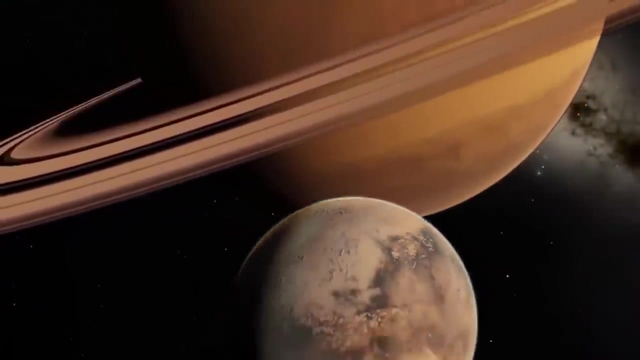 dance between the earth, the moon and the sun. And fourth, gravity holds galaxies and clusters of galaxies together, ensuring that celestial bodies do not fly into the depths of space. This cosmic glue supports the structure and integrity of the vast and impressive formations that define our universe. 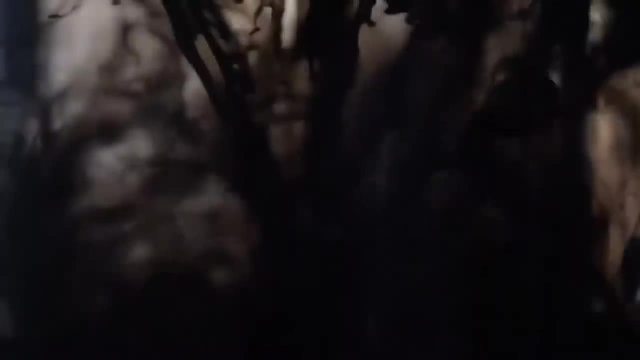 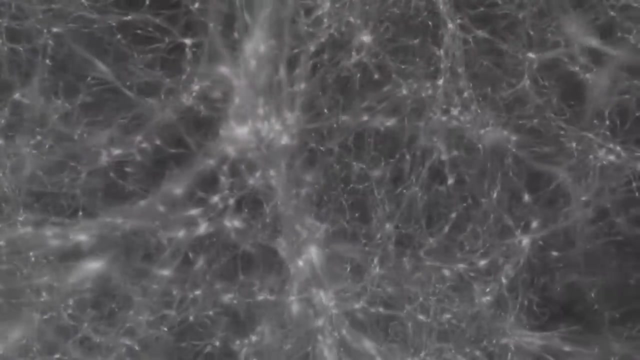 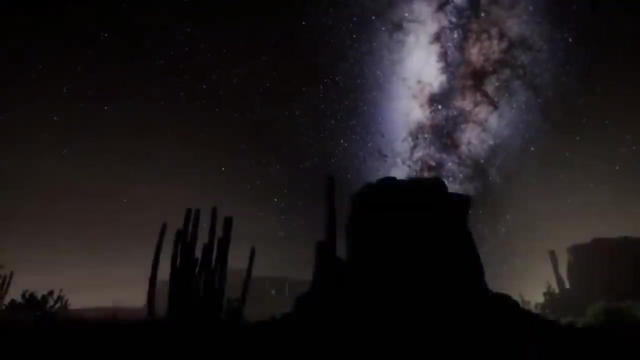 Studying and understanding the nature of gravity may, in the future, shed light on the mysterious dark matter, an invisible form of matter that does not interact with light or other electromagnetic radiation. However, its presence can be judged by its gravitational attraction to visible matter in space. 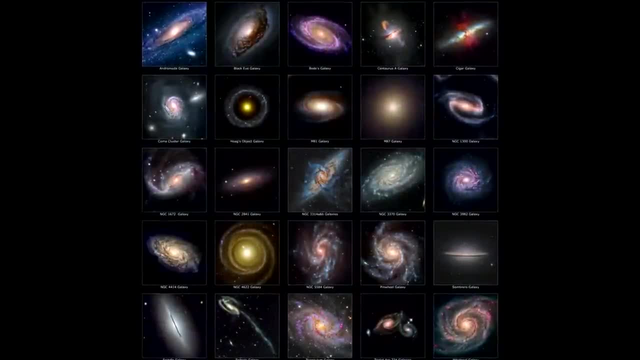 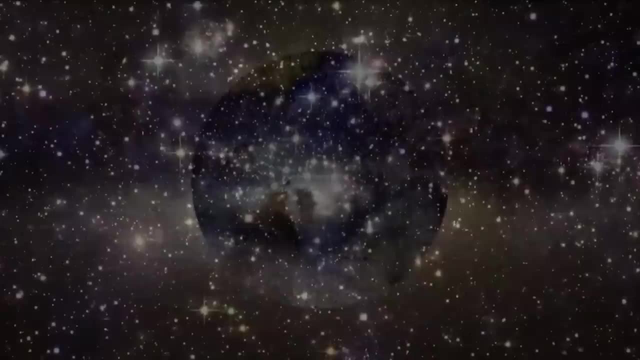 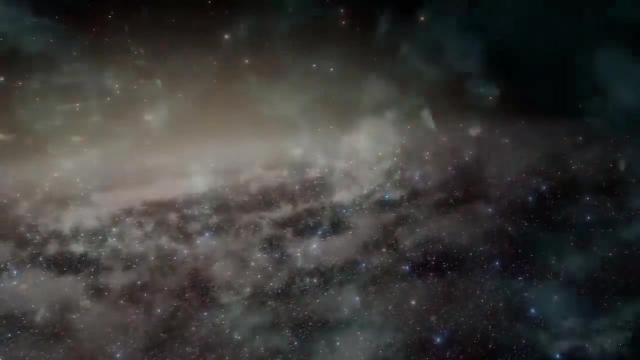 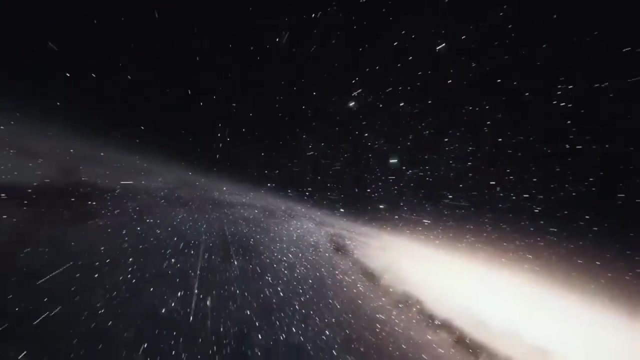 Measurements of the rotation curves of galaxies and large-scale structures in the universe show that there must be much more matter than what we observe in the form of luminous stars and gas. It is believed that this excess mass consists of dark matter, which affects the movement and distribution of galaxies and galaxy clusters through gravitational forces. 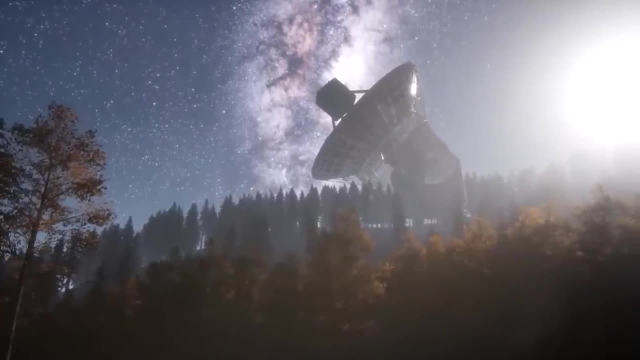 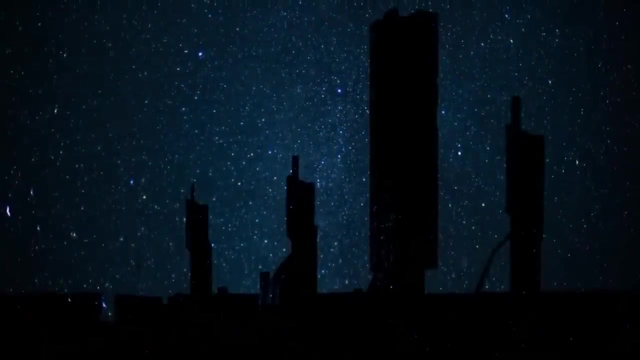 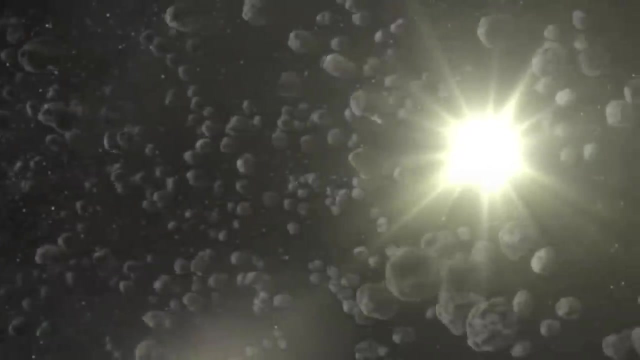 Thanks to technological progress in the study of gravitational waves, humanity has new tools for studying the elusive characteristics of gravity. Ultimately, unravelling the mysterious force of gravity will help us better understand our place in space and shed light on reality as we know it. 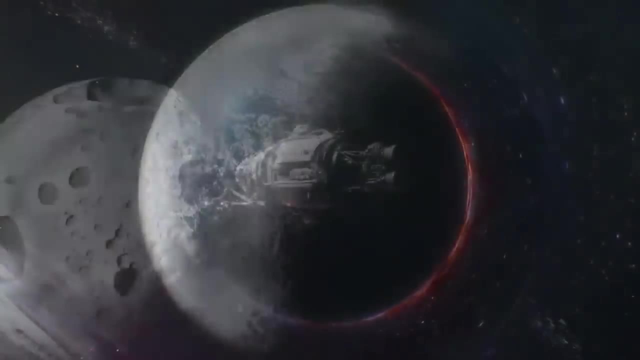 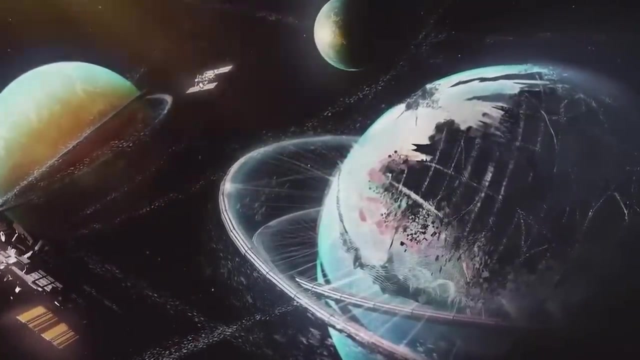 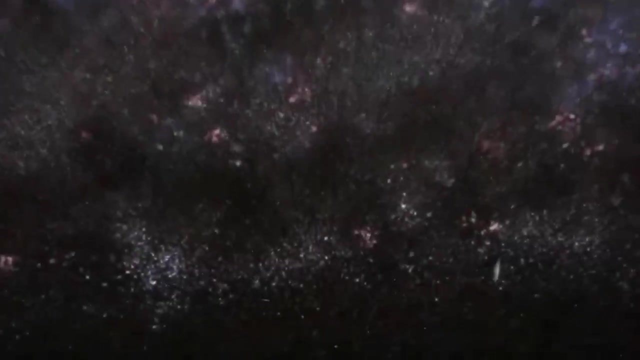 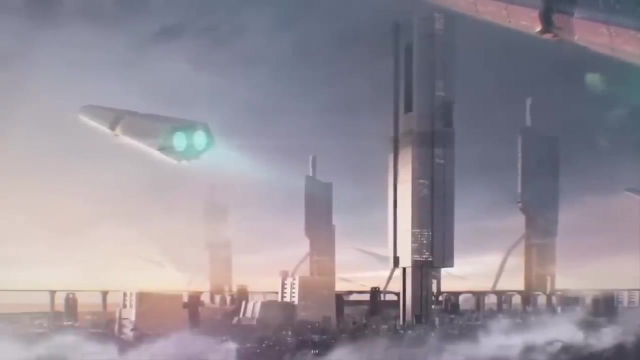 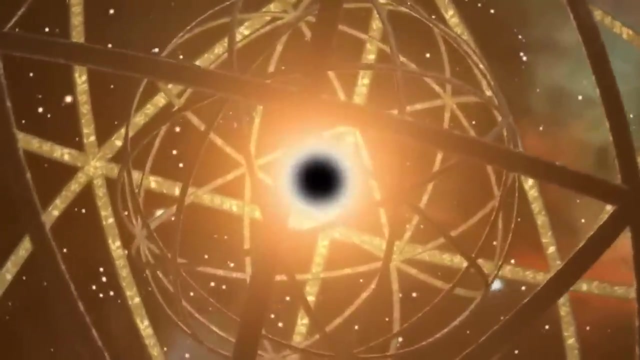 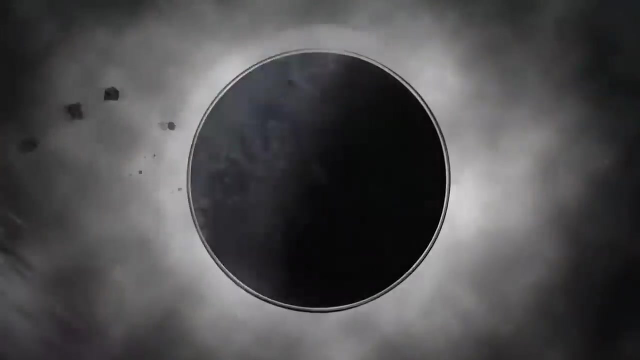 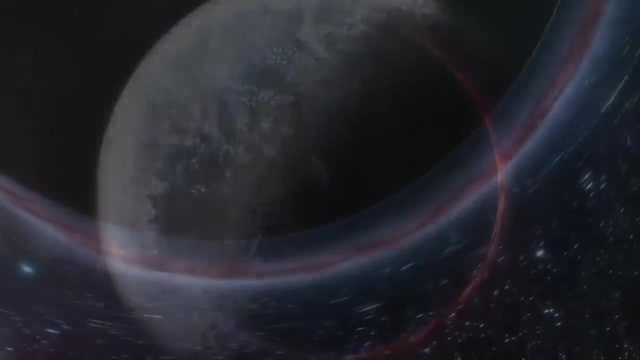 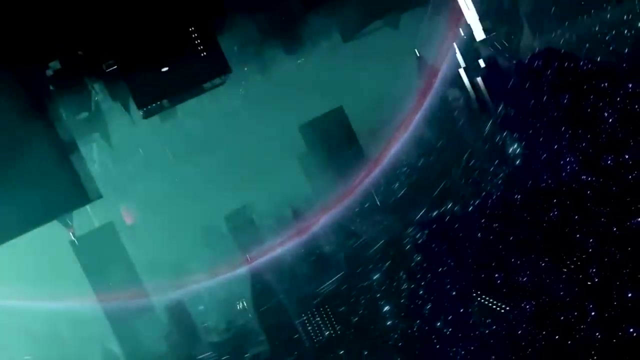 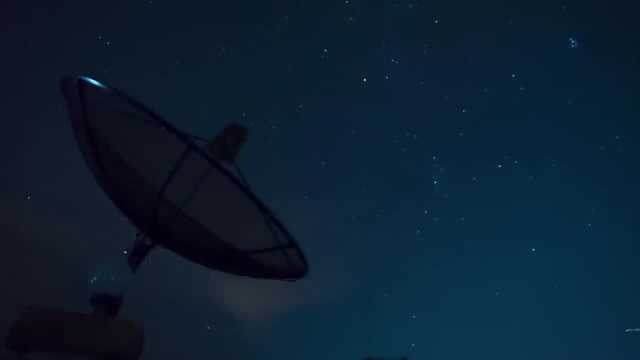 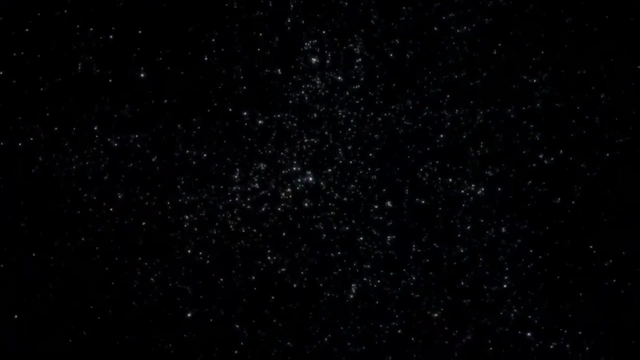 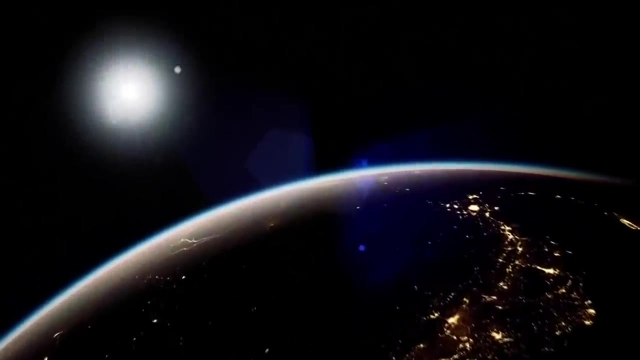 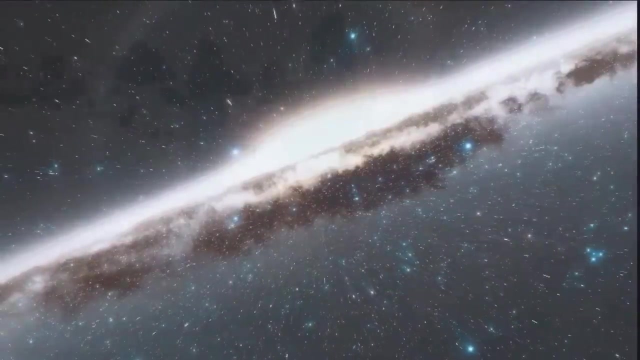 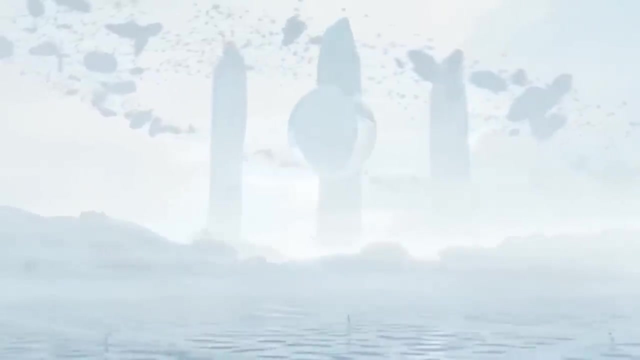 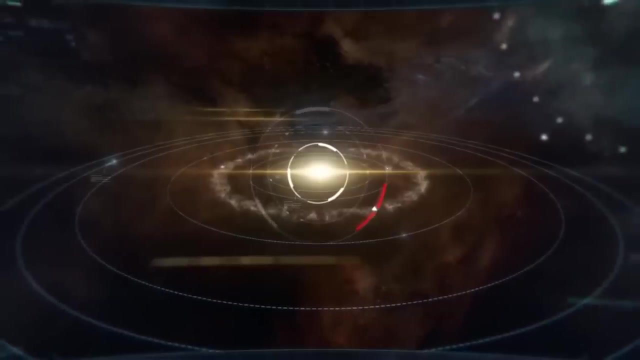 Tonic, The Earth Elementary Scientific Institute, kenzo University of Michigan. Osho Imperial University, University of Chicago. Thank you, Thank you. In the mysterious valleys of space where the stars twinkle against the dark mantle of night, a huge galaxy is hiding which attracts the eyes of astronomy lovers, dreamers and writers. 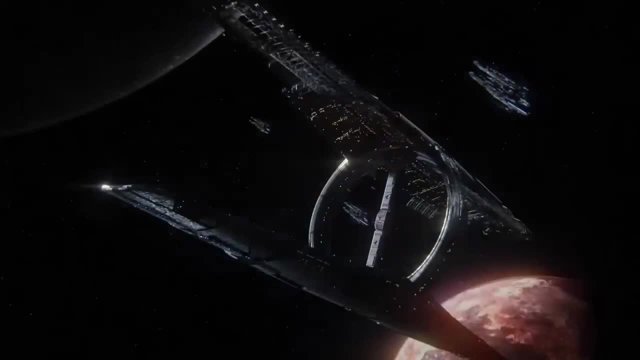 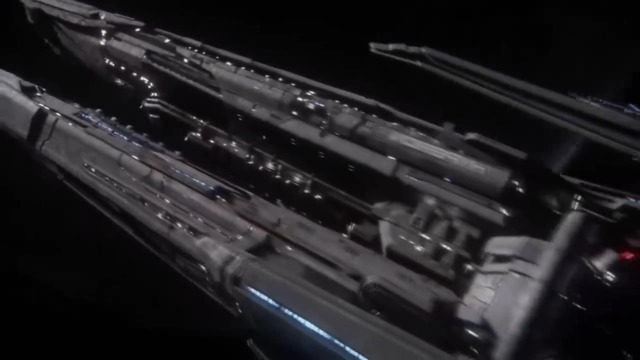 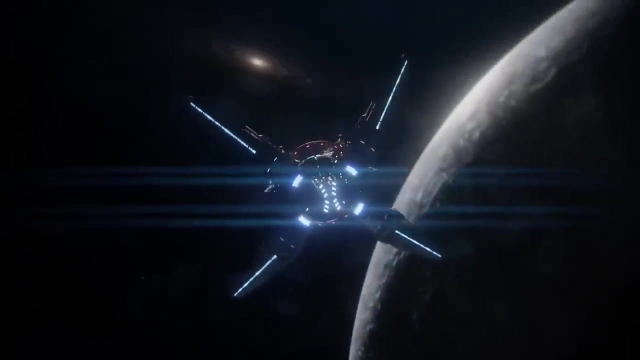 This galaxy is named Andromeda And today we will make a grand journey to her heart, to the very center of the galaxy. An alluring adventure, mesmerizing with bright colors and the promise of new discoveries, begins right here: Andromeda Galaxy or M31.. Our nearest stellar neighbor. 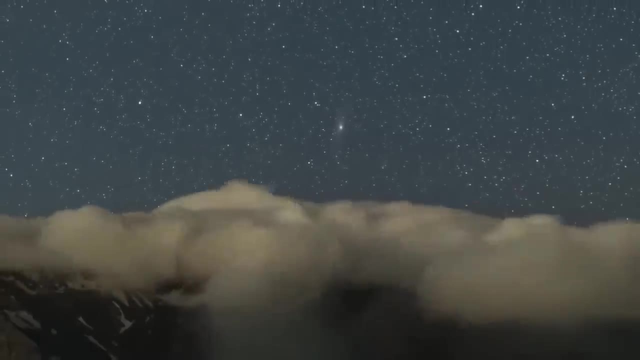 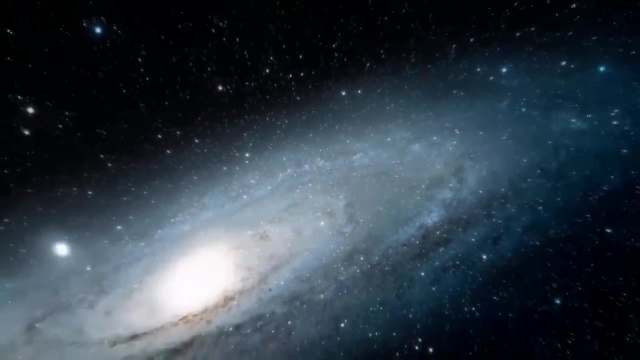 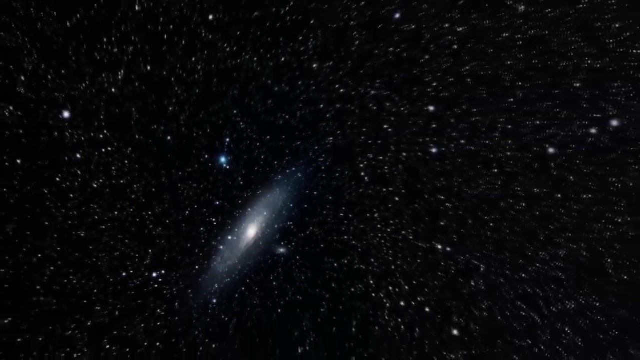 On a clear night, it can be seen in the sky with the naked eye. It is located at a distance of about two and a half million light-years from Earth and its diameter is approximately 200,000 light-years. And although it seems incredibly far away, but in fact it is not so at all. 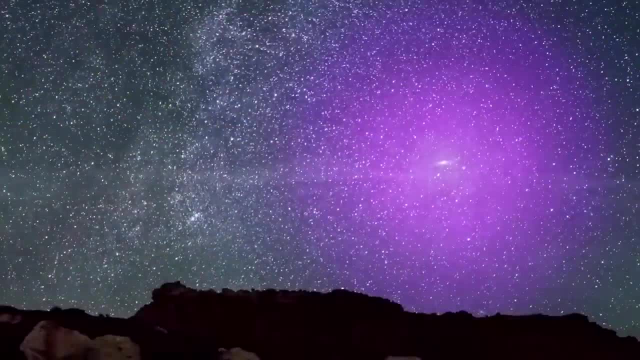 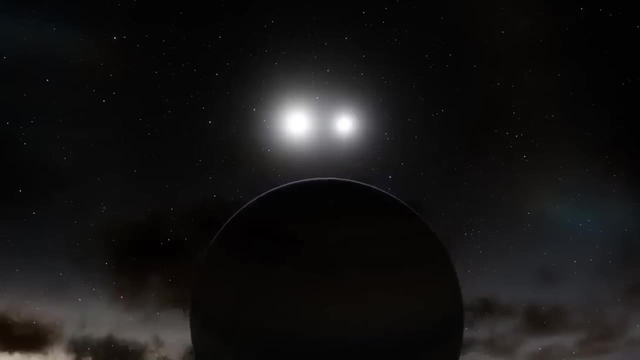 If this halo could be seen without magnifying glasses, in the visible spectrum it would be three times larger than the constellation Ursa Major and create the illusion of a second core. The age of the blue stars surrounding the black hole does not exceed 200 million years. 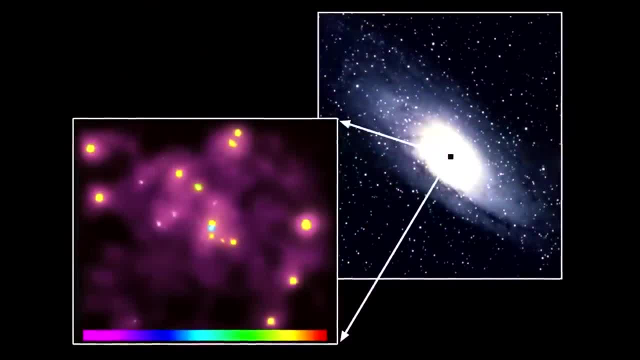 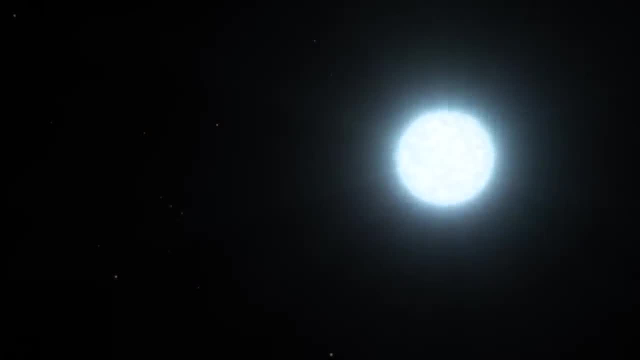 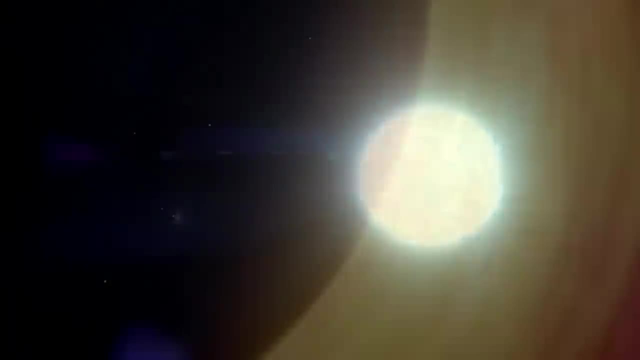 so they must have been formed near the black hole as a result of a sharp burst of star formation. Massive blue stars are so short-lived that they would not have enough time to migrate to a black hole, if, of course, they formed elsewhere. Researchers are trying to understand how apparently young stars formed so deep inside. 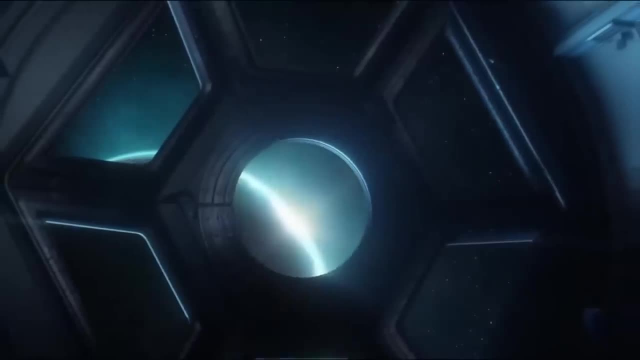 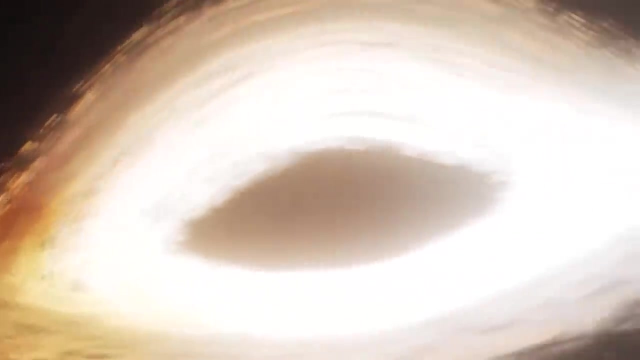 the gravitational grip of a black hole, and how did they survive in such an extreme environment at all? As we delve deeper into the mystery that is the black hole at M31, its enormous size, power and complexity are revealed, giving us amazing insights into its fantastic role. 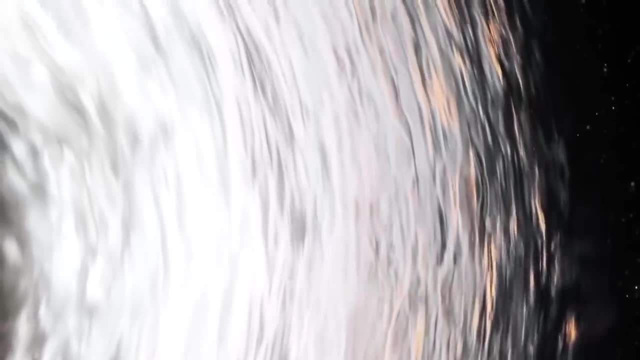 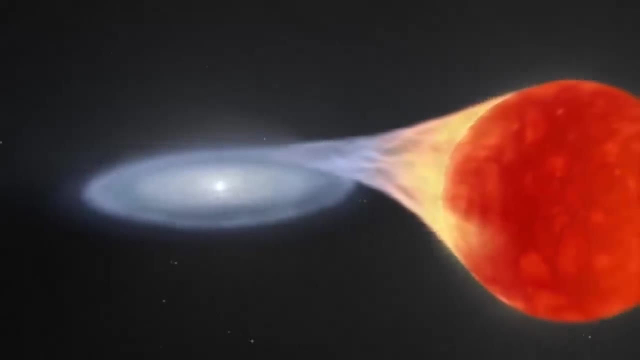 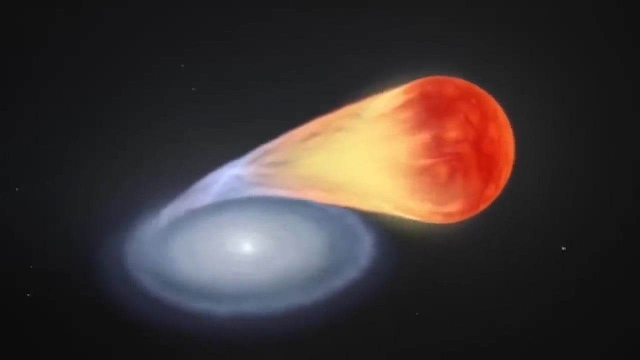 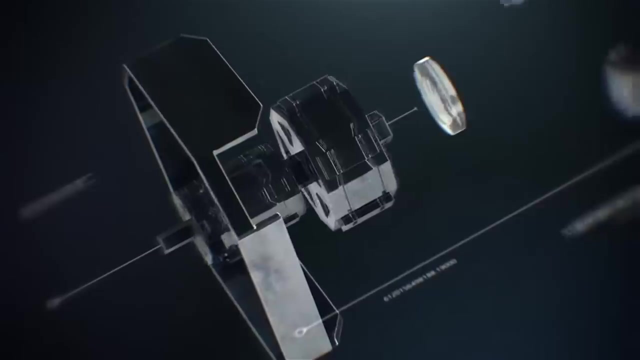 in shaping the cosmic landscape. Its irresistible gravitational force not only attracts stars, gas and dust, but also forces them to move in an orbit and spiral to the event horizon, an invisible boundary where nothing, not even light, can escape its capture. As technology advances and our ability to explore the universe expands, the supermassive 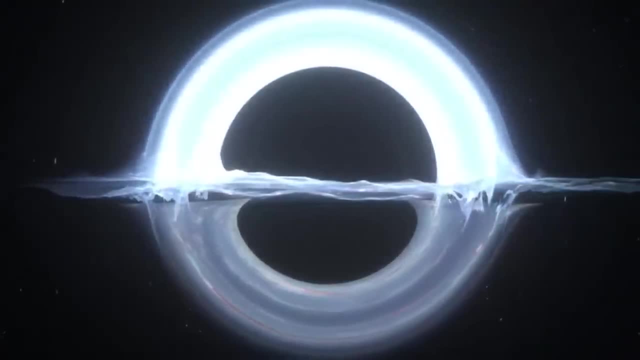 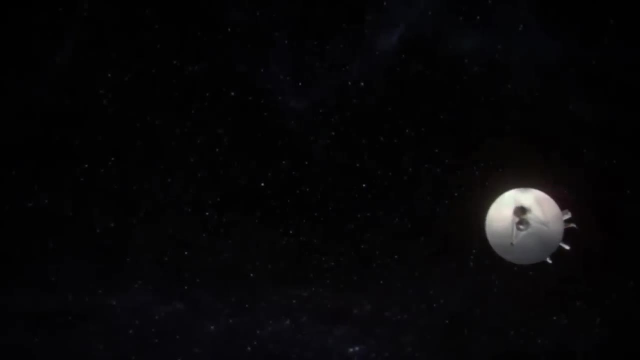 black hole at the center of the Andromeda galaxy will become an even more exciting object for scientific research As we continue to unravel its mysterious. wherever it may centers, we can see that it tries to unravel its mysteries. this cosmic miracle will undoubtedly be a beacon of knowledge. 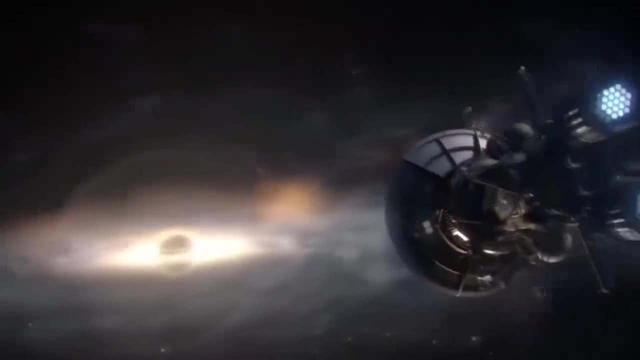 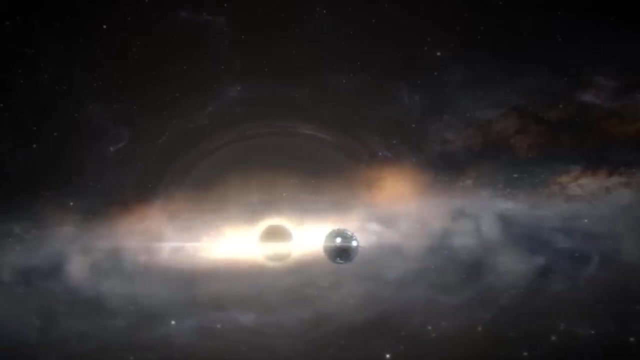 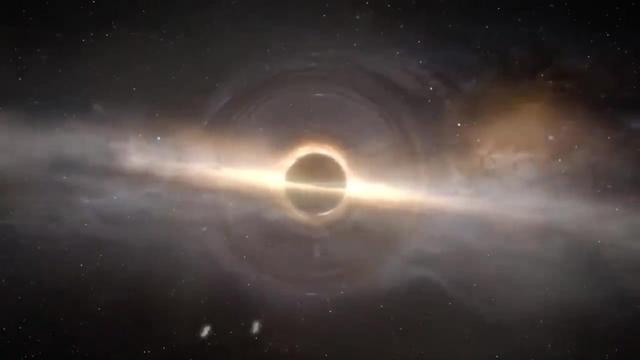 for many generations of astronomers and enthusiasts. But our goal is to dive into the black hole of this galaxy, possibly by sending an umbrella there A moment and the device disappears from the radar. Nice try, It seems. our journey has come to an end. Today we crossed the vast expanses of space in the 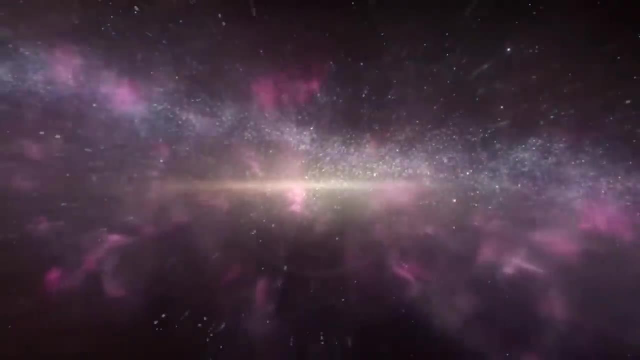 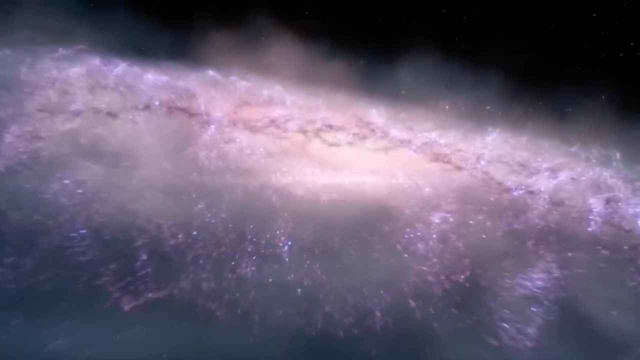 Andromeda Galaxy, encountering wonders that are difficult to imagine: Supernovae emitting unearthly light, nebulae swirling like heavenly smoke, newborn stars emerging from their gaseous manger and, of course, a huge, supermassive black hole playing the main part in the symphony. 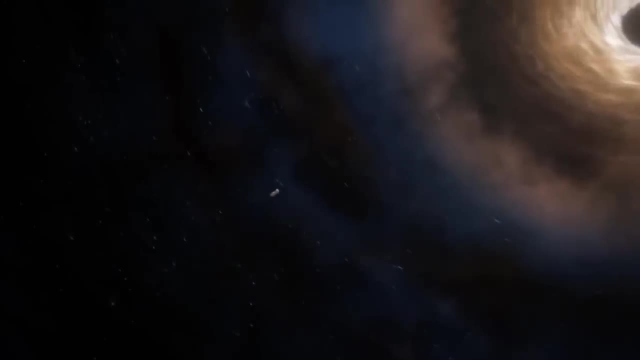 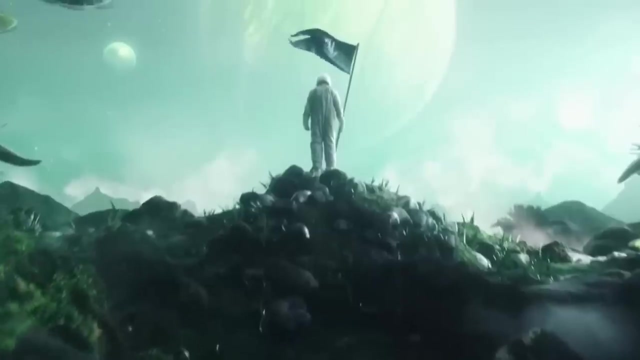 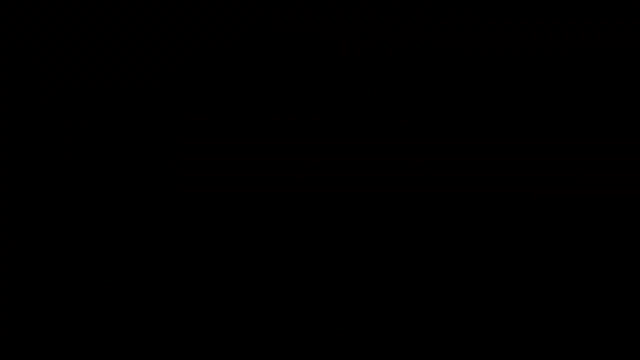 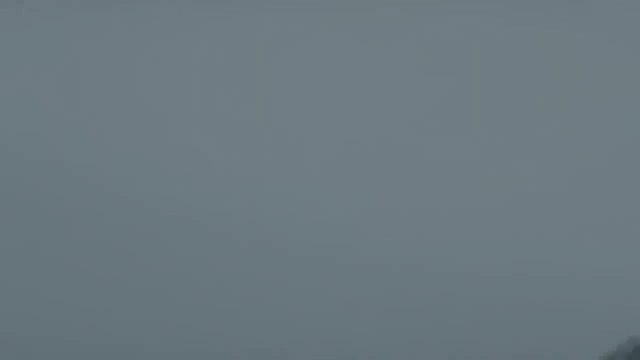 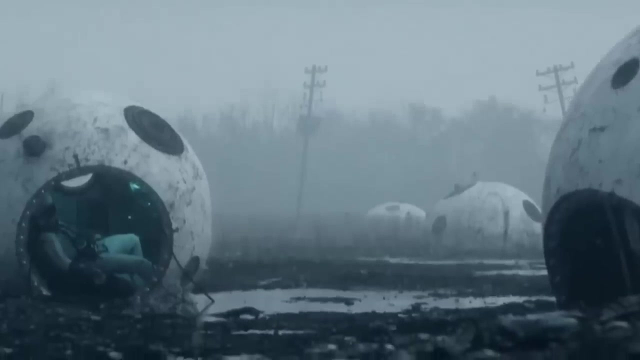 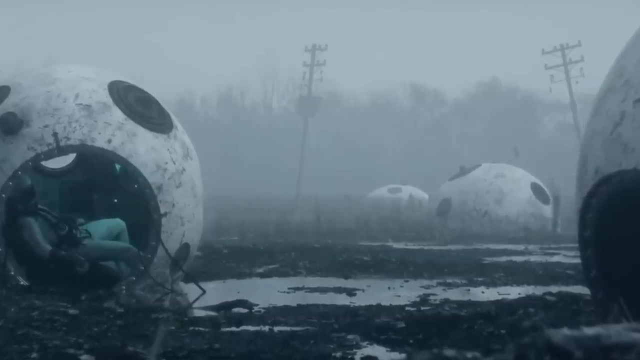 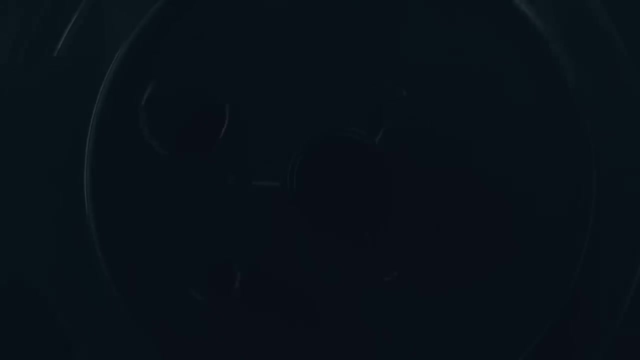 of cosmic evolution. The journey to the center of Andromeda was just the beginning and we are ready to chart a new course for the next great adventure And new discoveries. Now we know the top: unstructured, mysterious and mysterious. 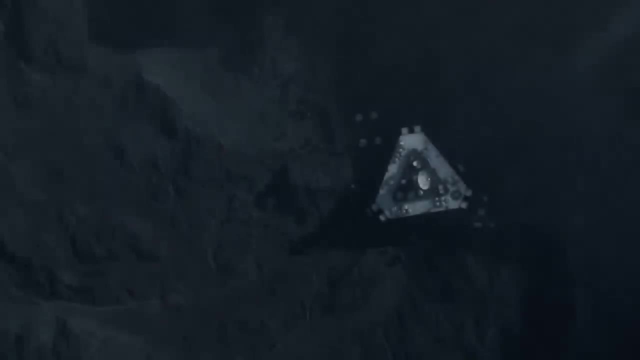 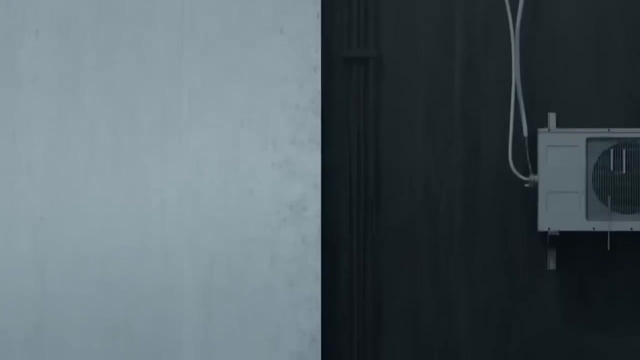 But we know we need to head for another one. We're, on a way, unobstructed On the weapon we're all so familiar with, But we need to get started. And now we're ready. We're ready to go, And here we are.